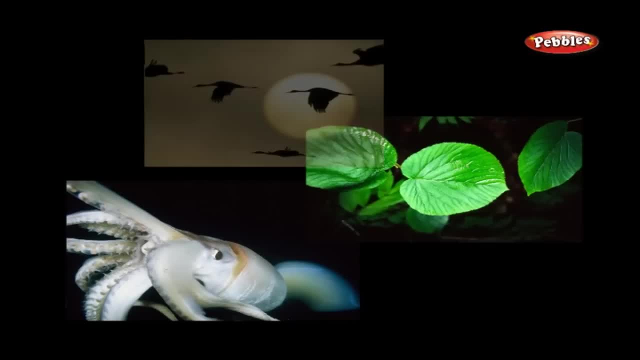 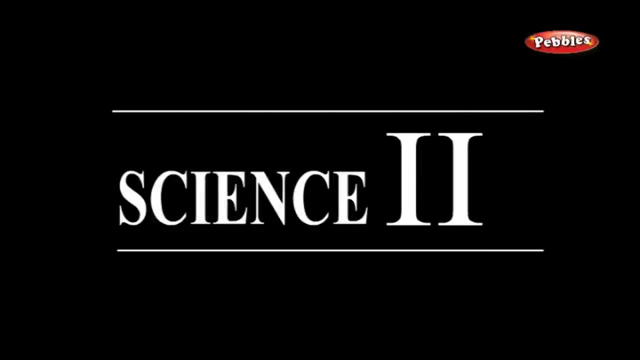 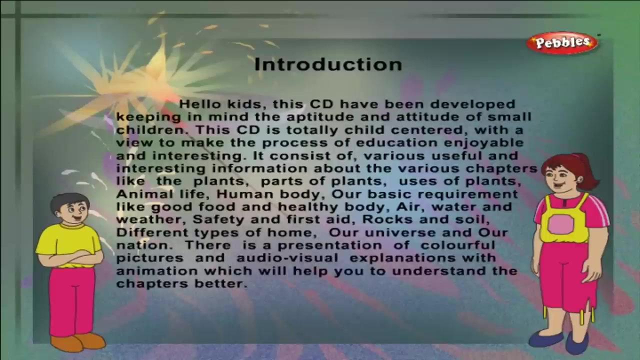 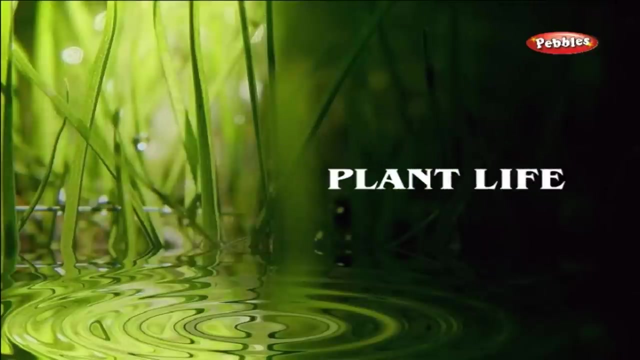 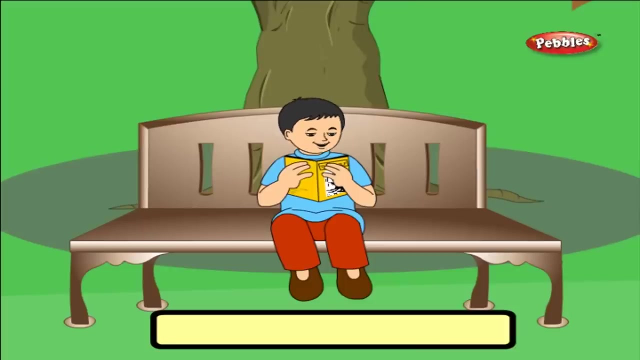 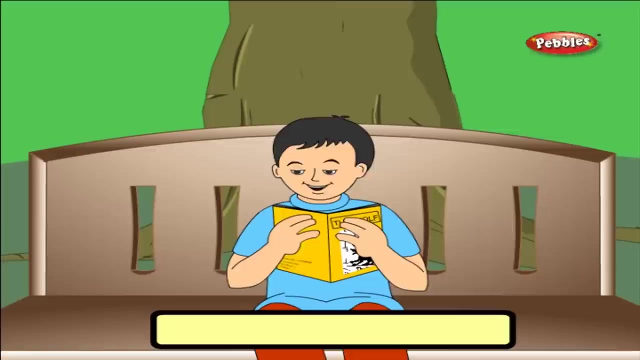 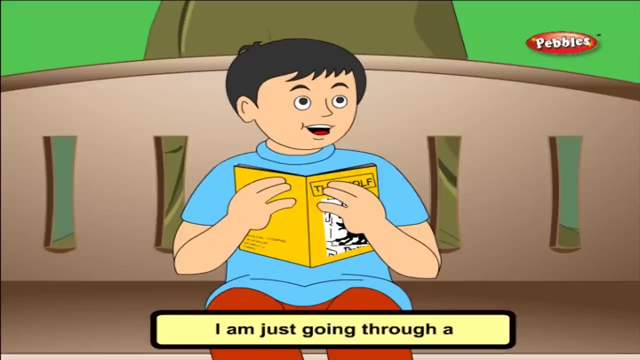 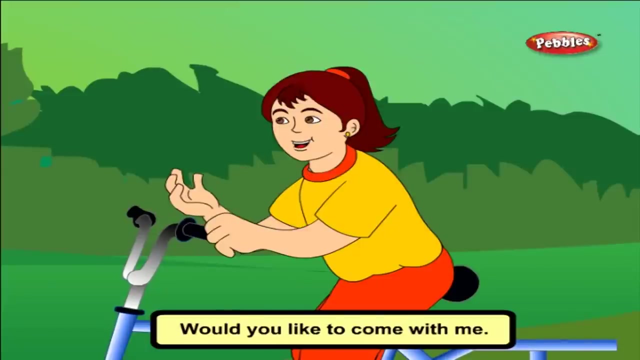 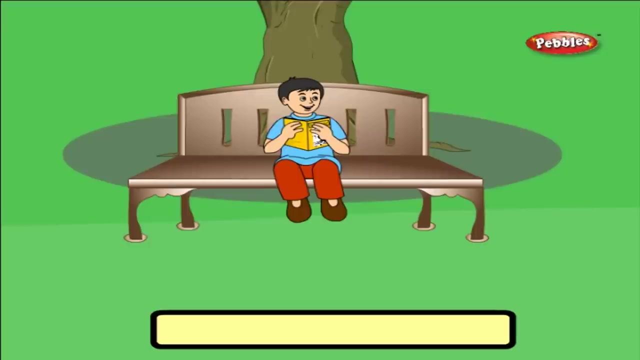 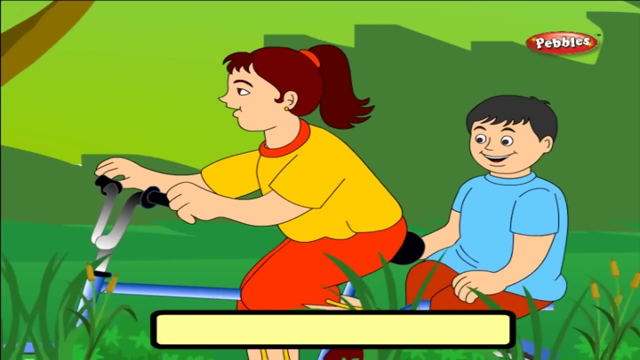 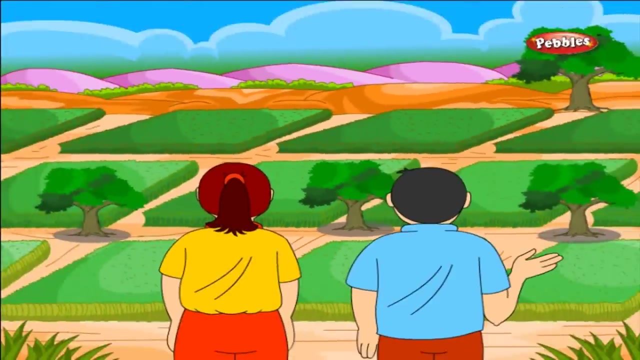 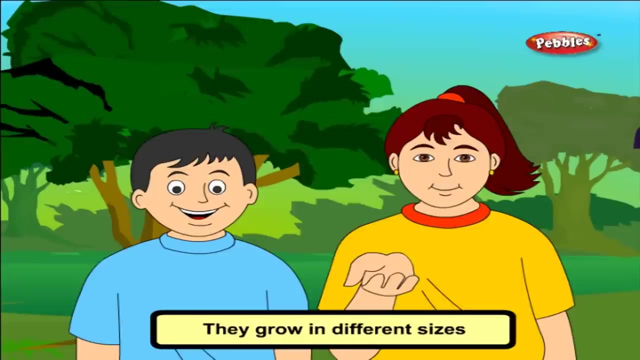 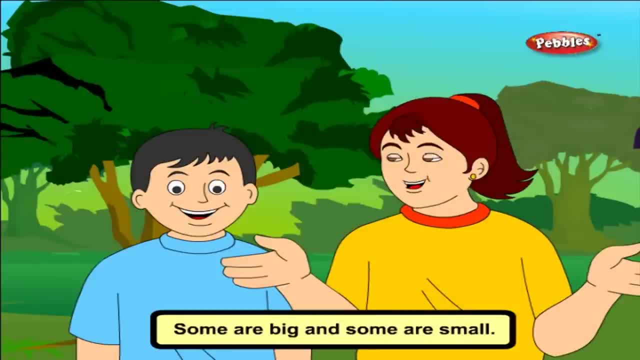 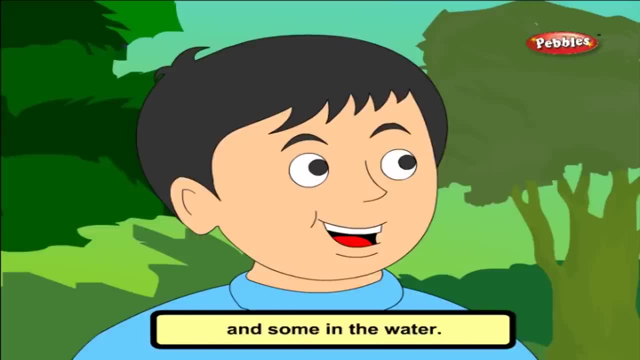 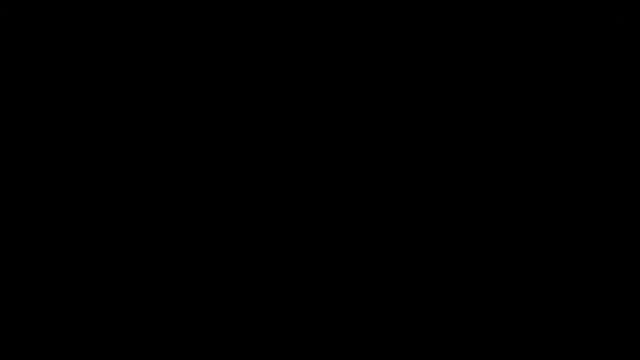 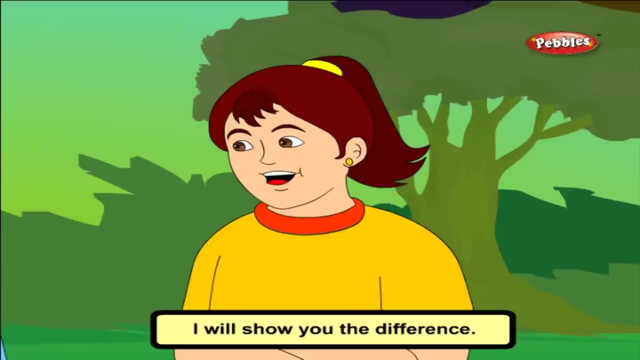 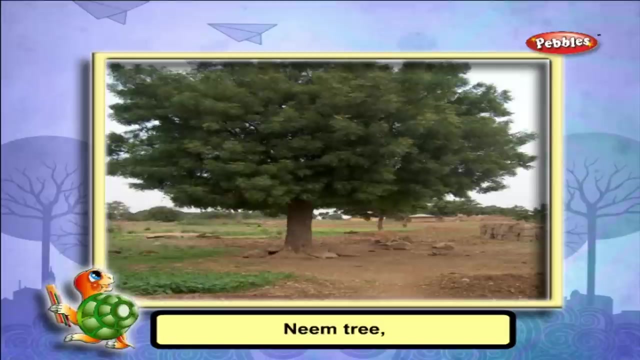 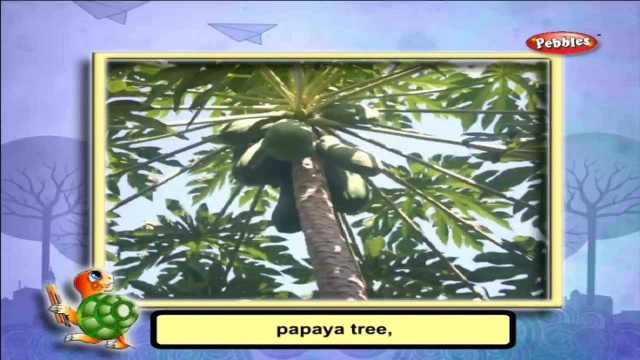 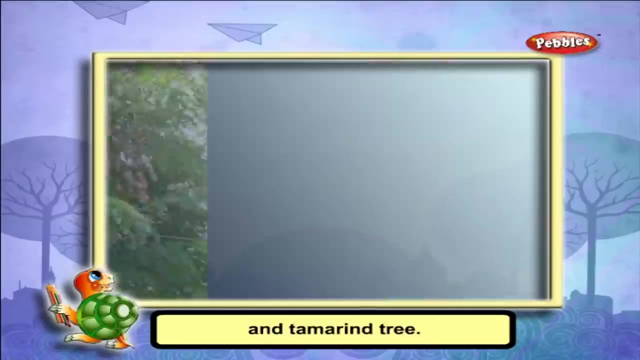 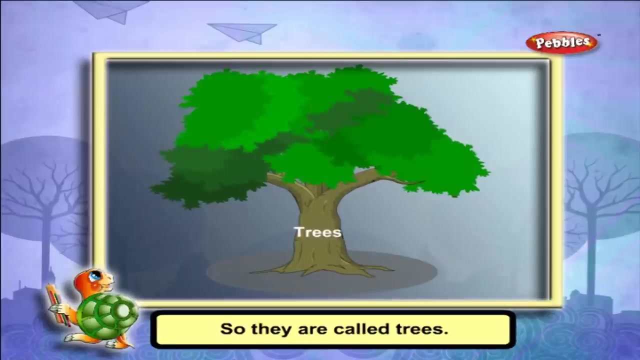 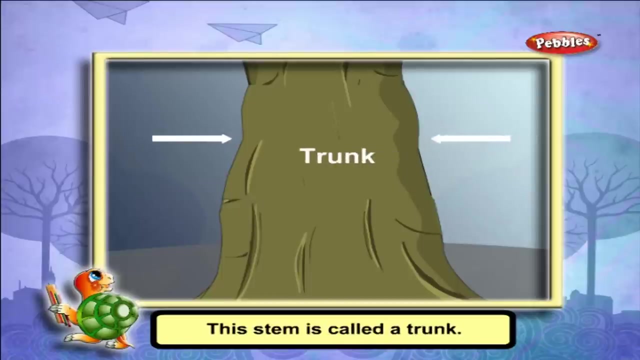 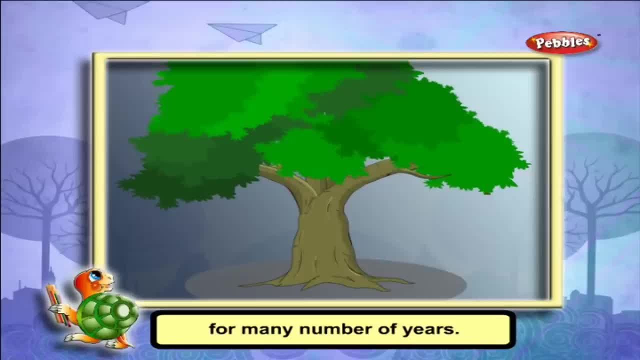 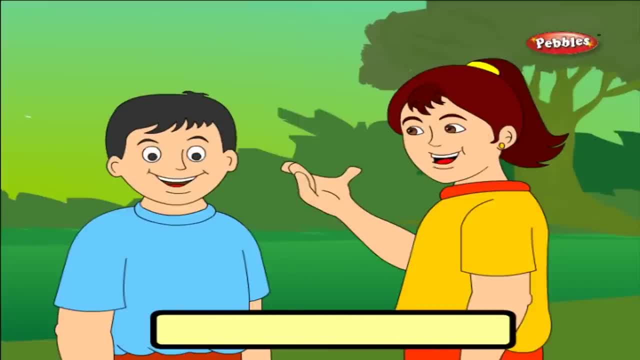 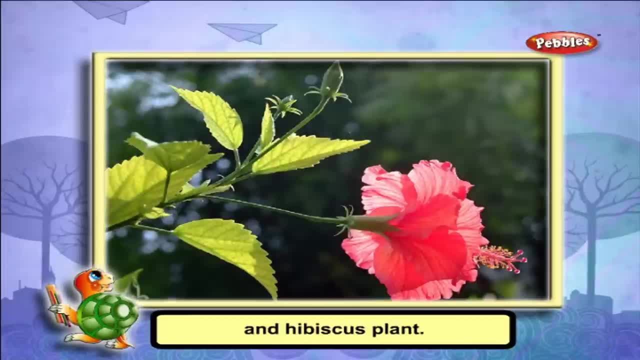 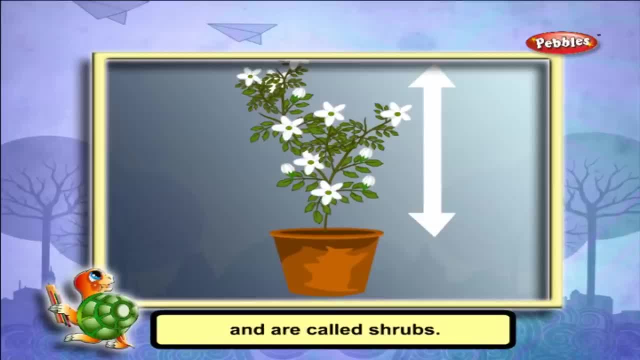 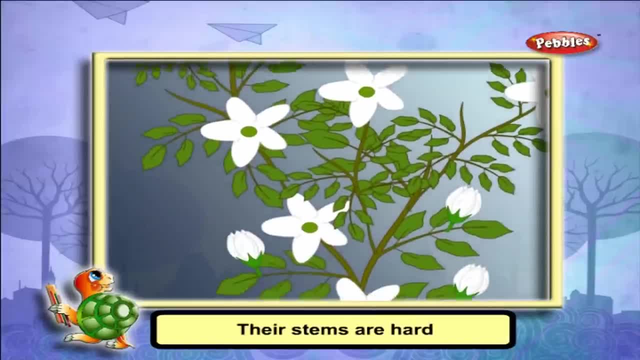 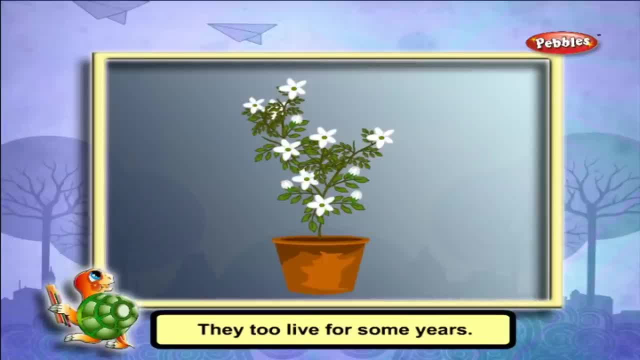 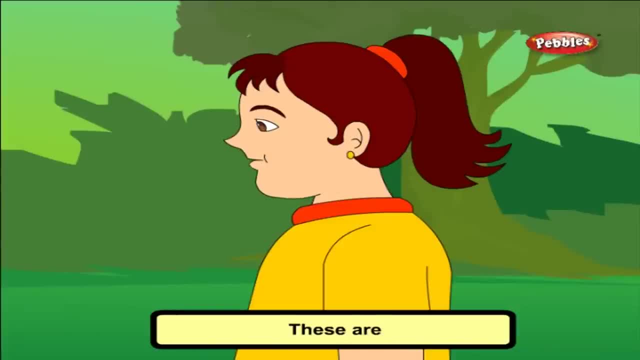 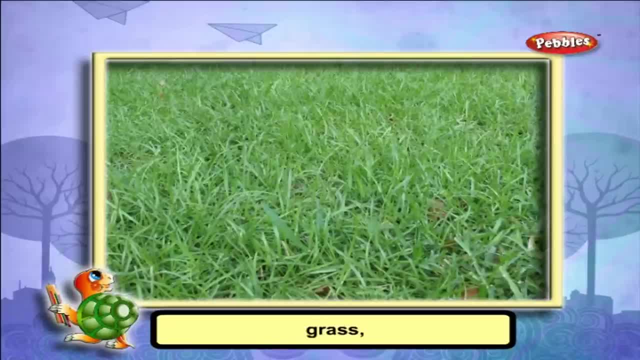 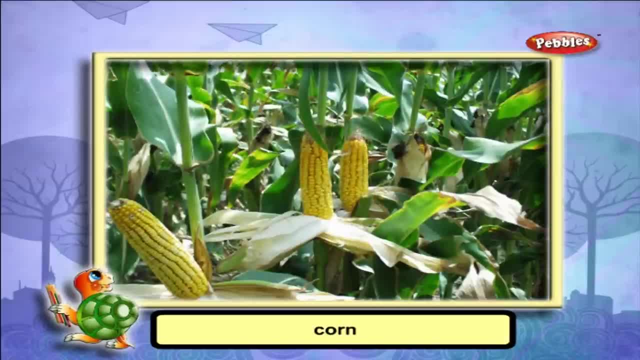 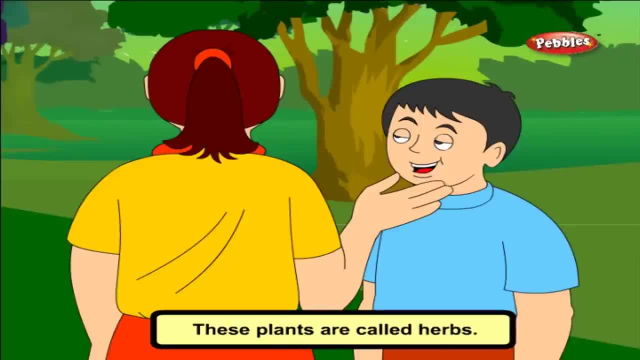 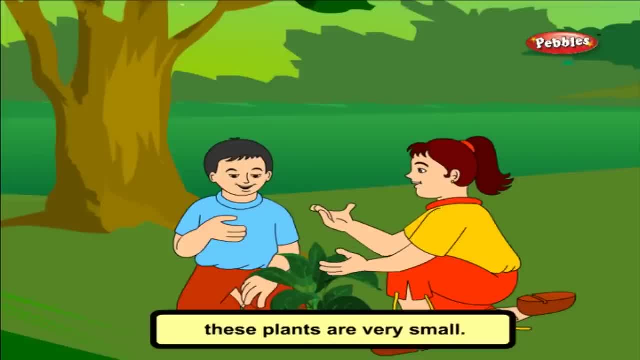 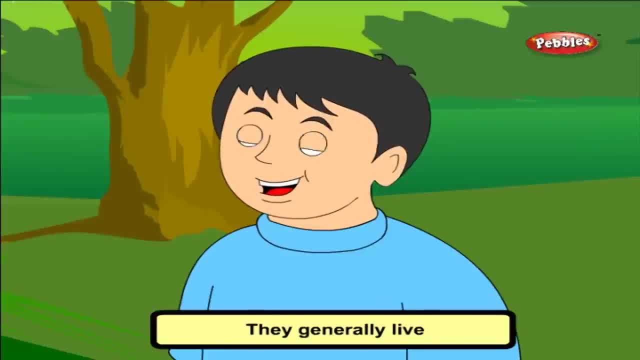 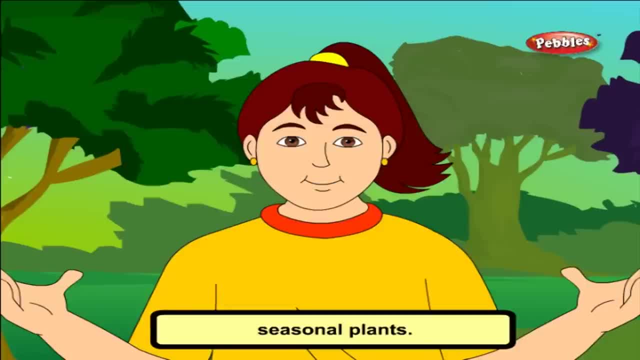 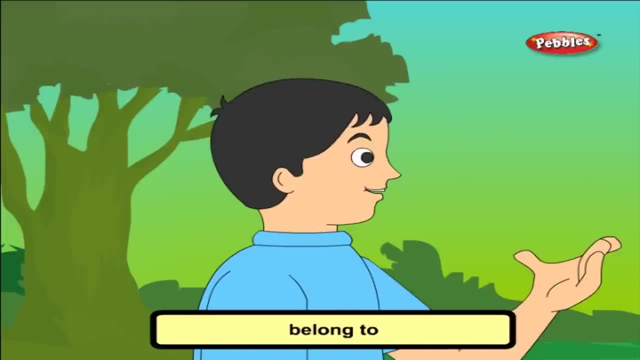 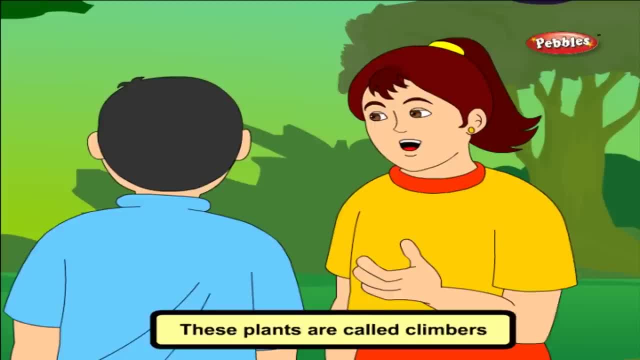 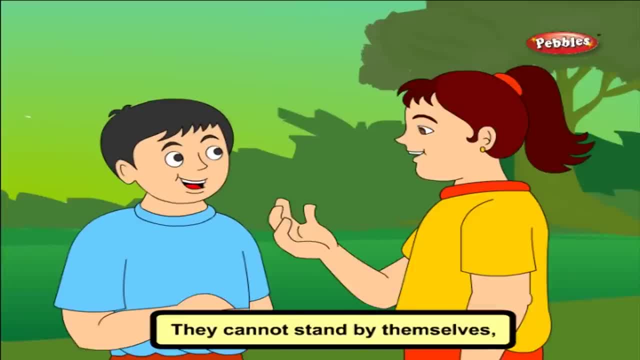 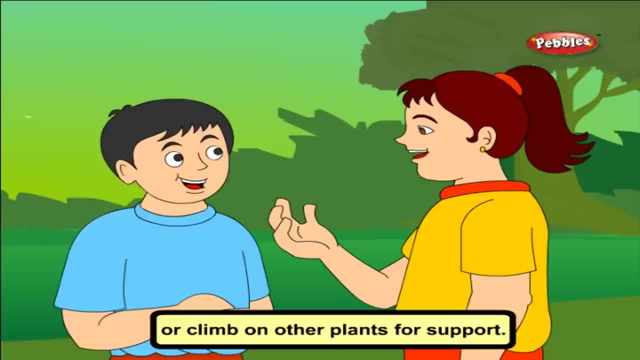 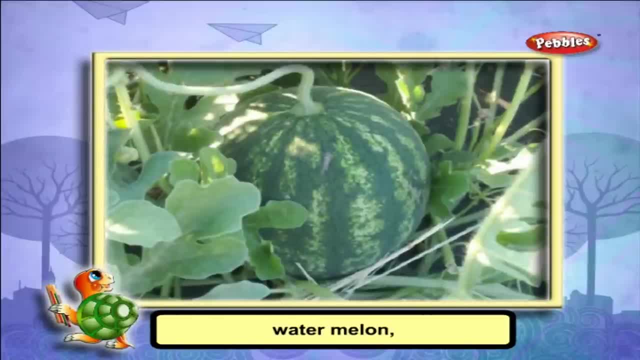 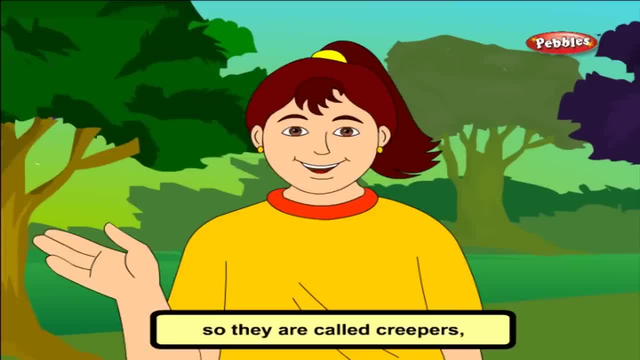 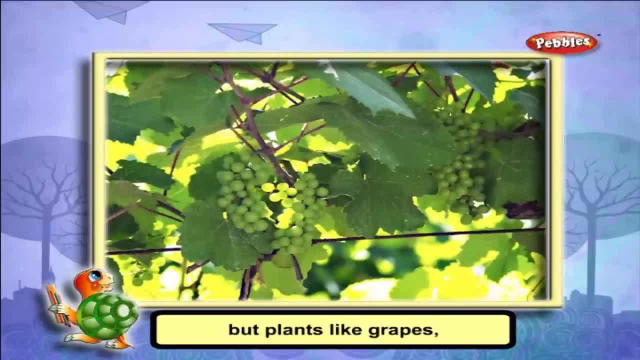 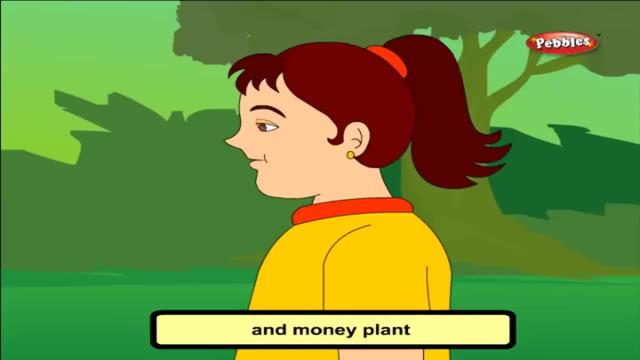 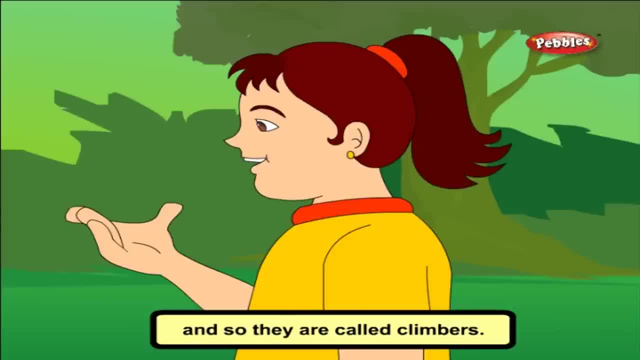 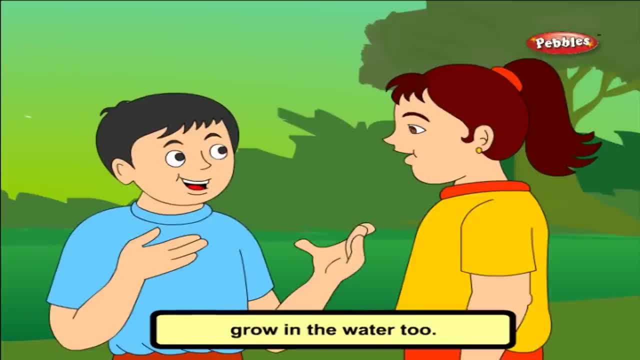 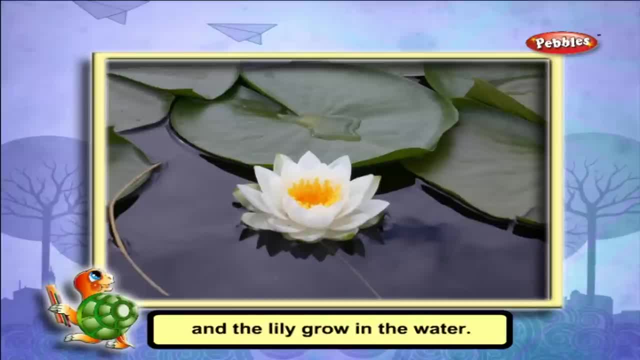 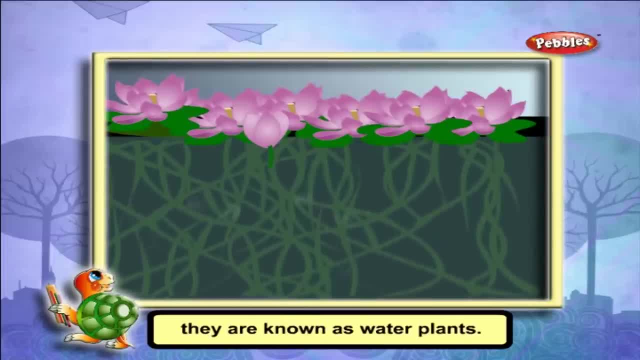 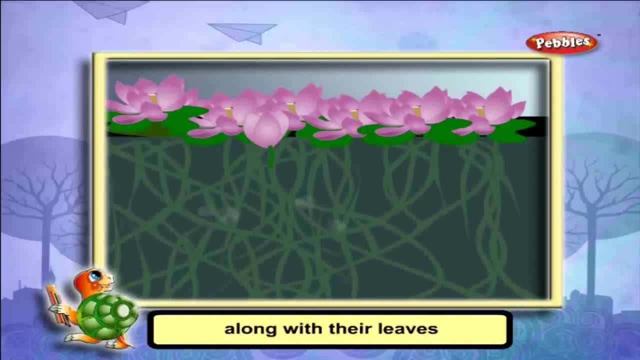 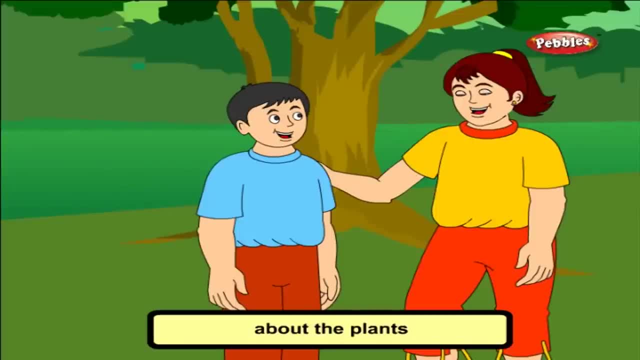 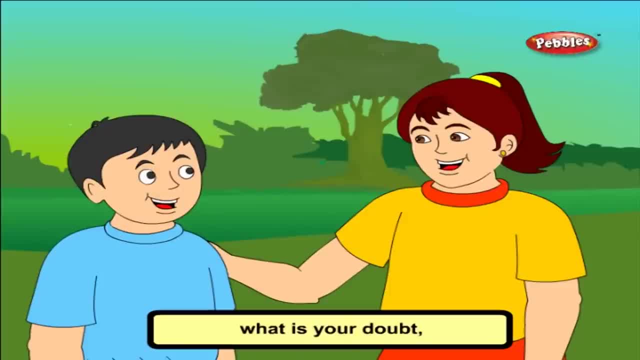 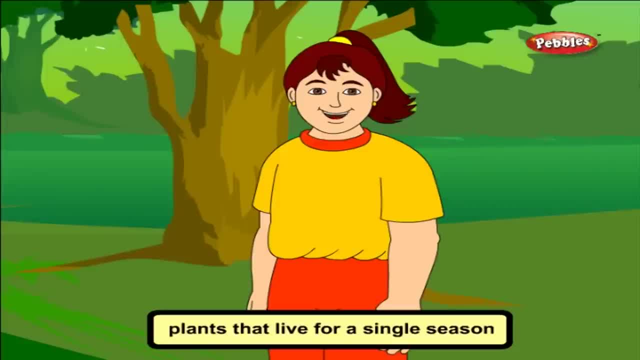 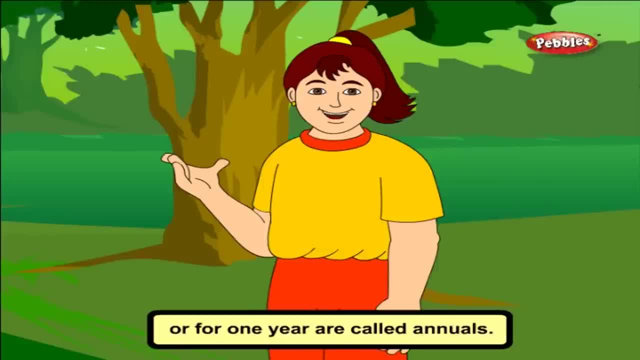 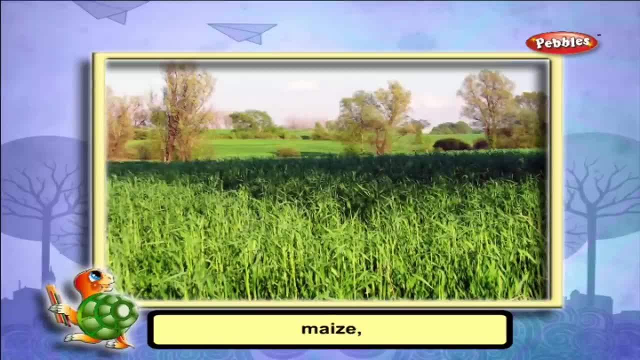 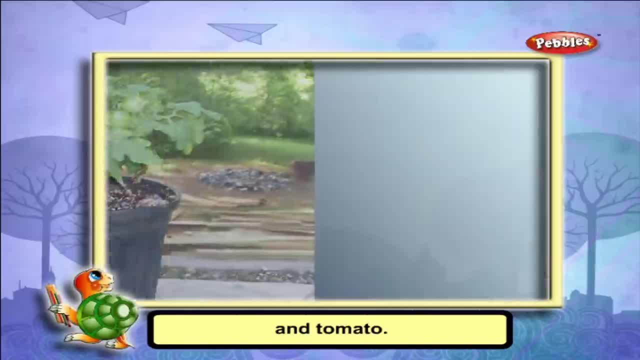 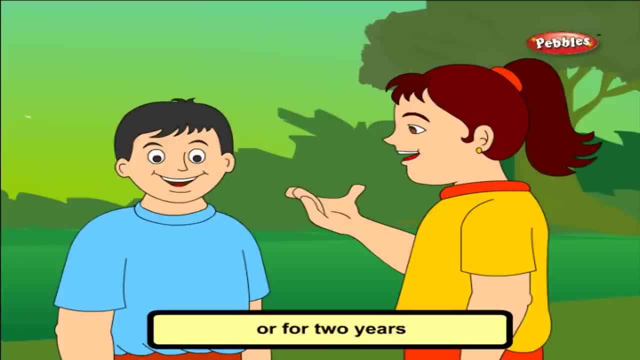 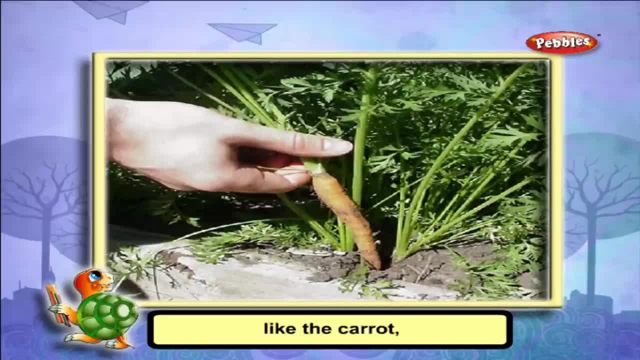 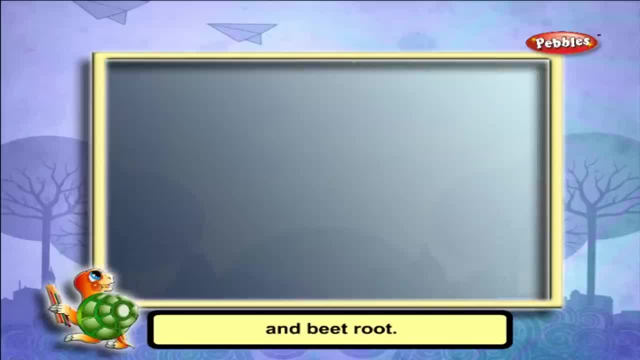 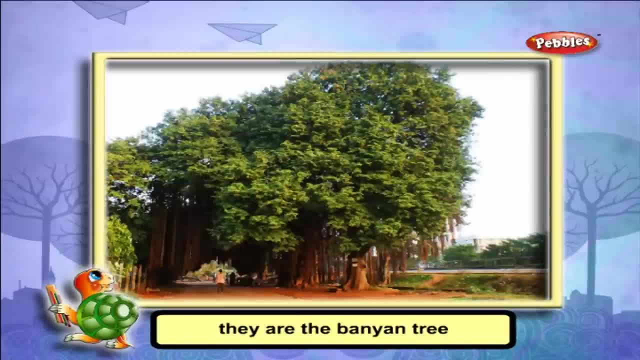 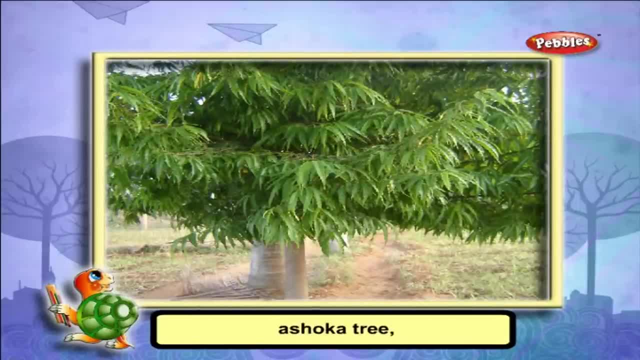 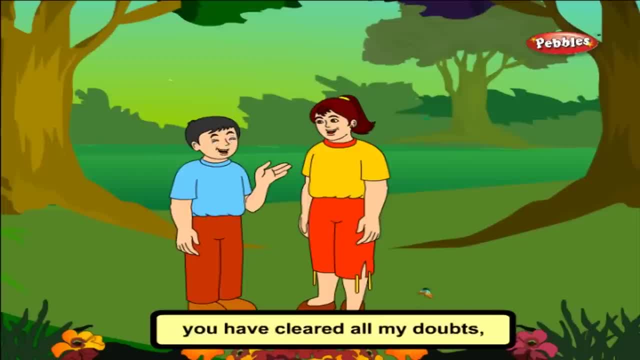 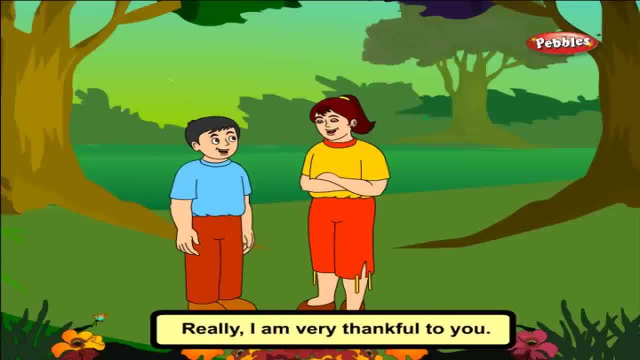 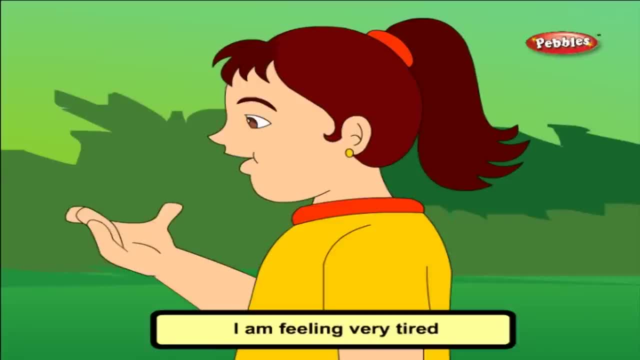 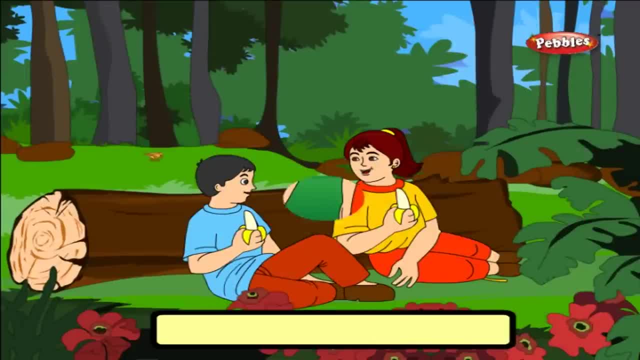 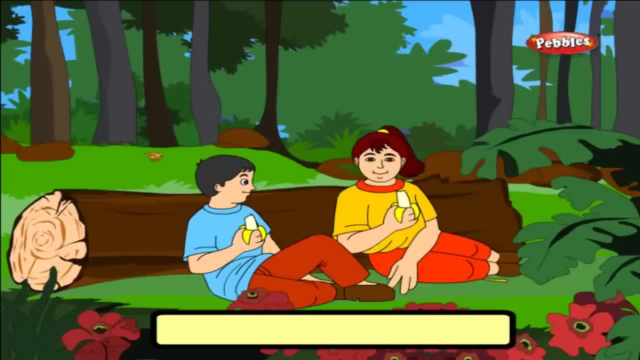 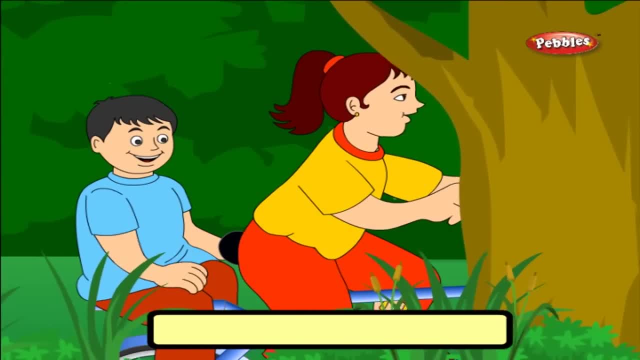 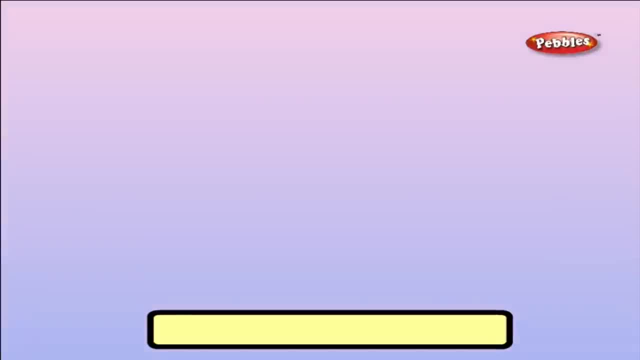 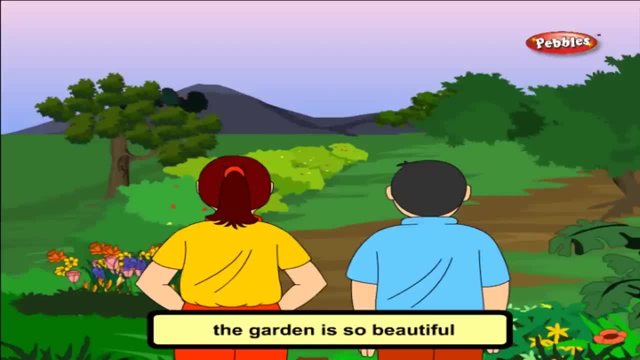 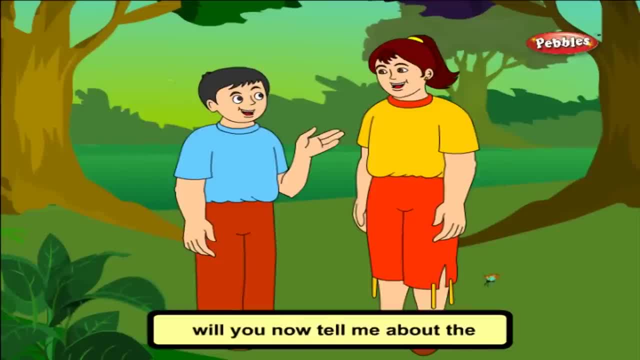 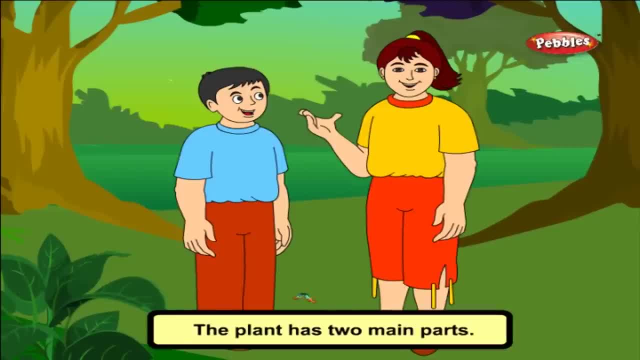 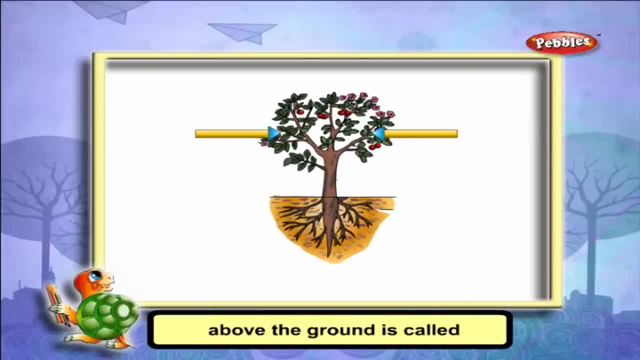 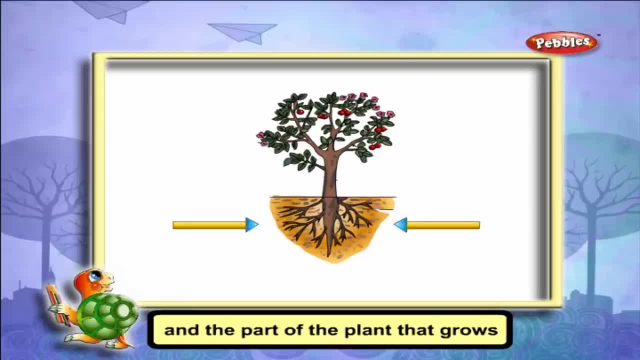 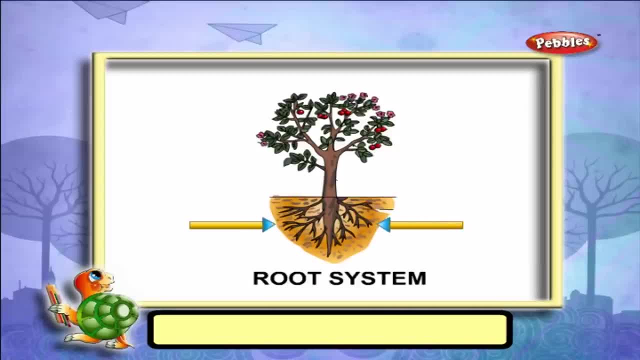 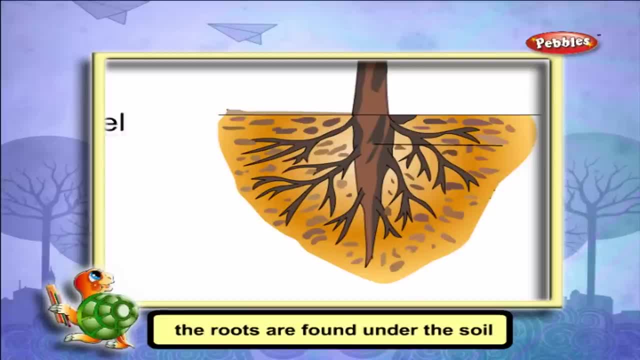 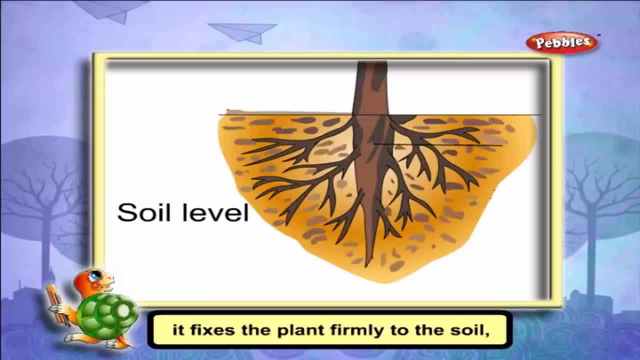 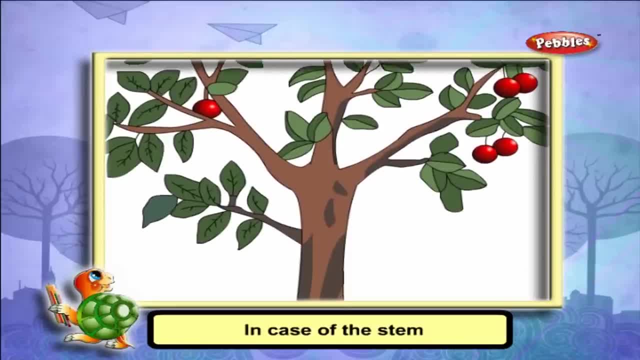 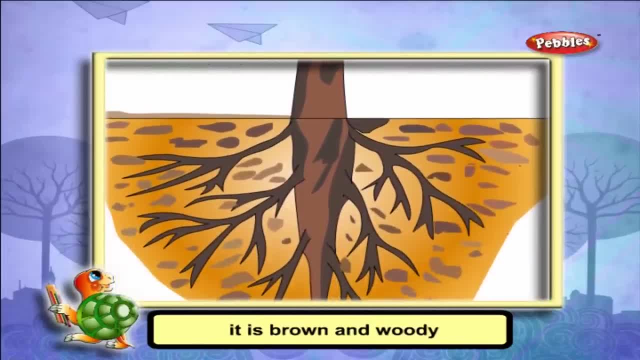 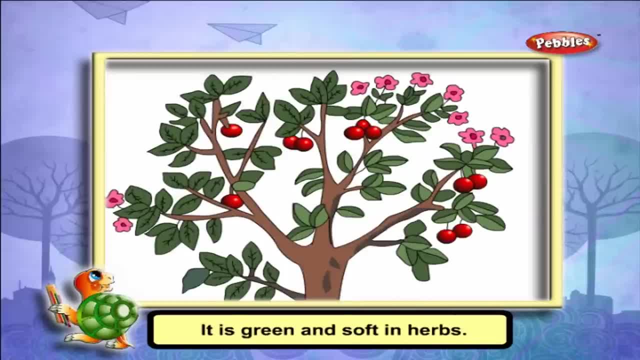 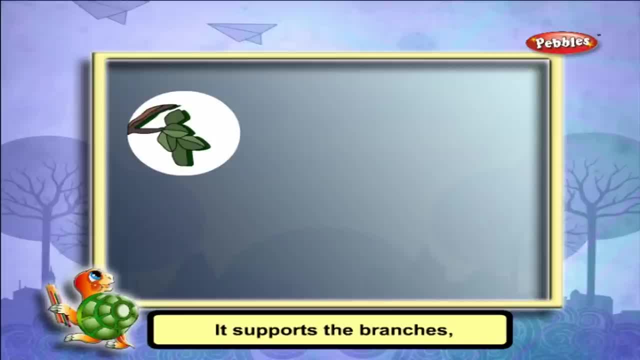 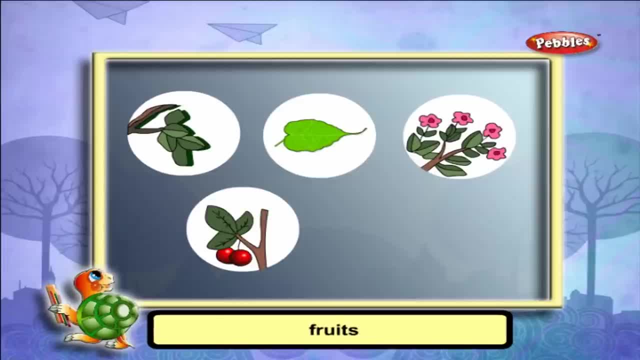 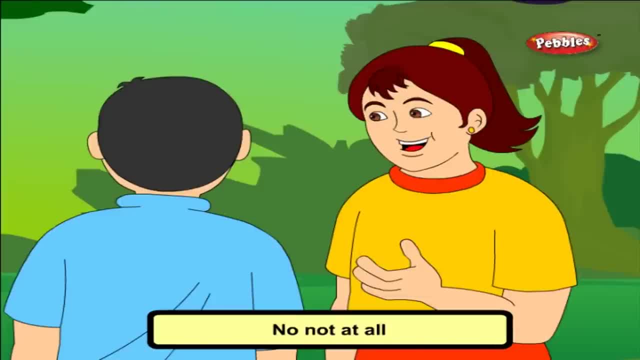 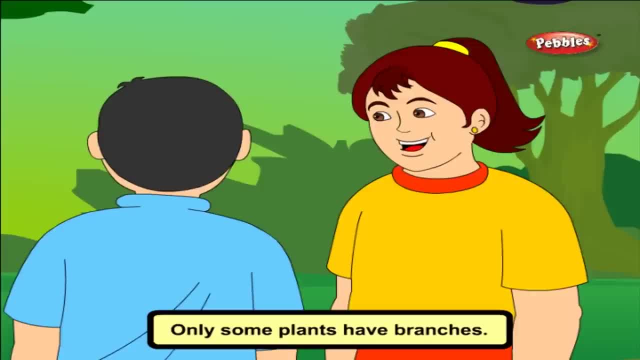 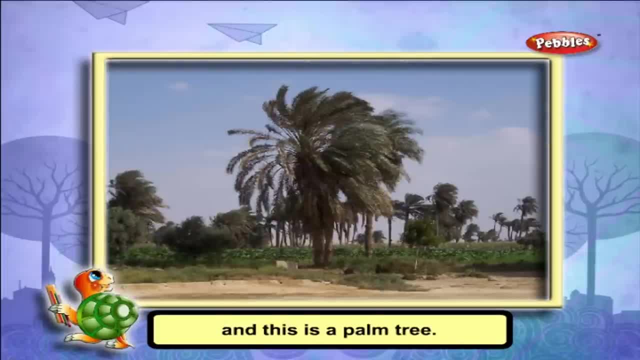 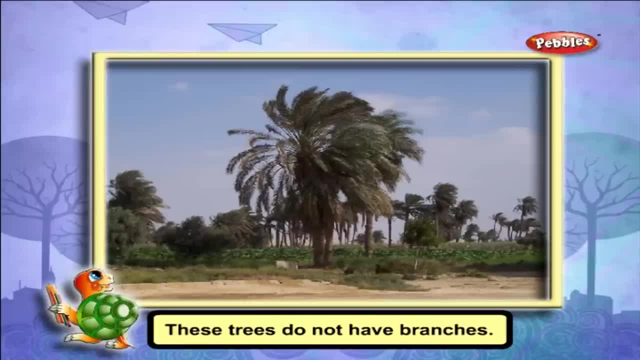 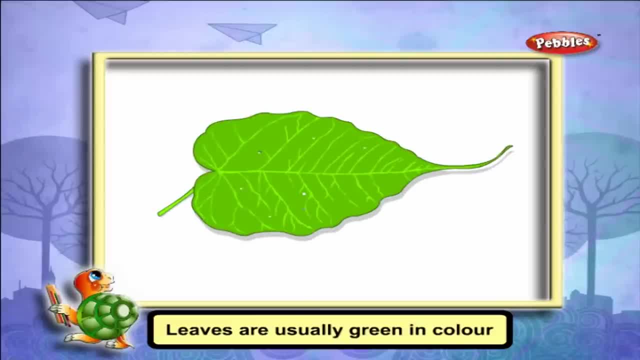 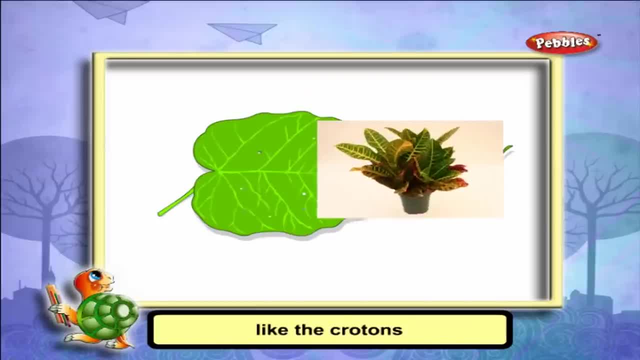 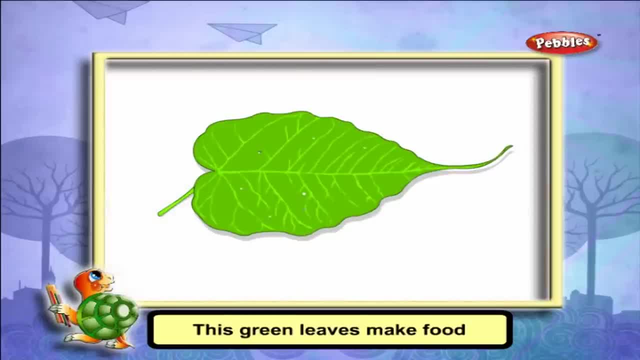 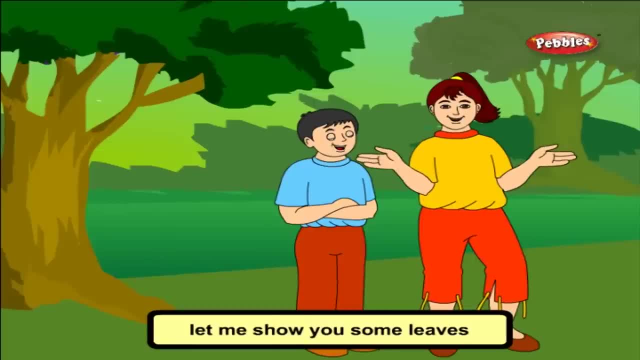 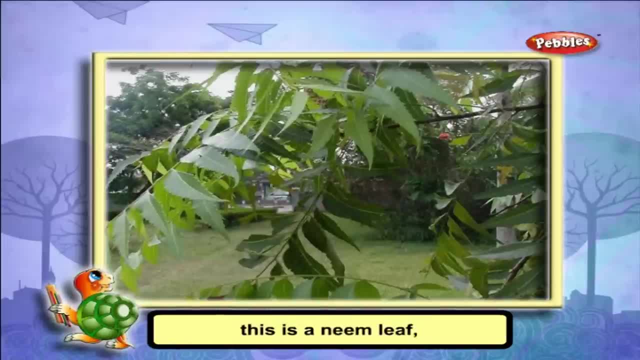 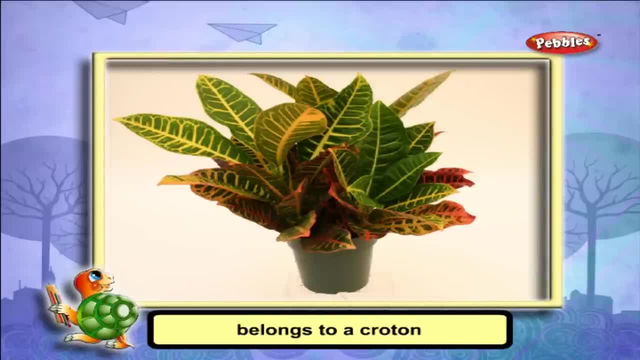 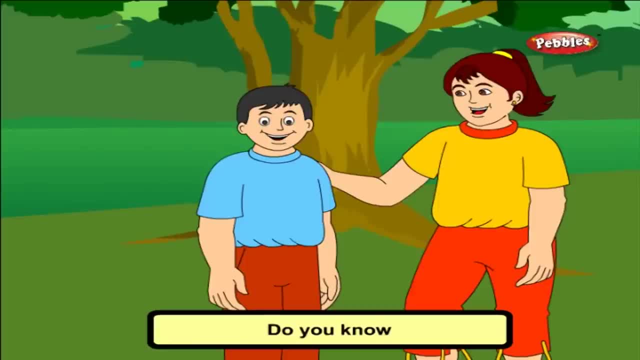 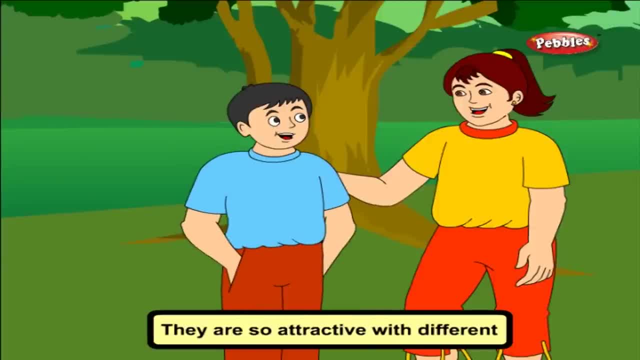 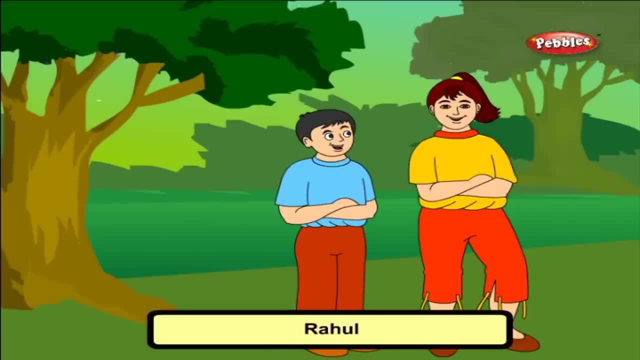 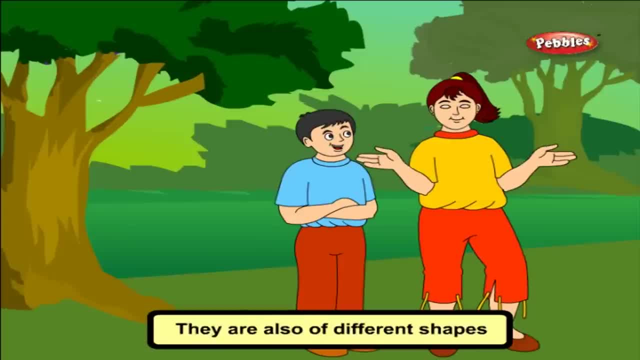 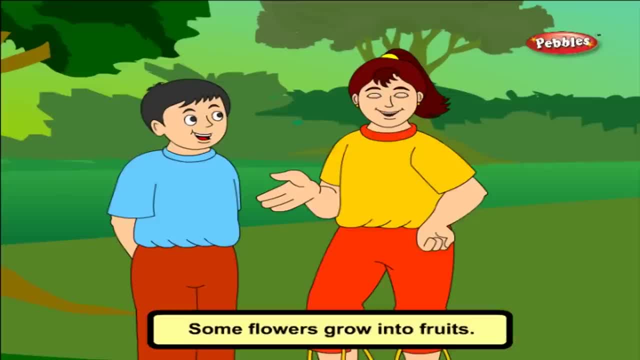 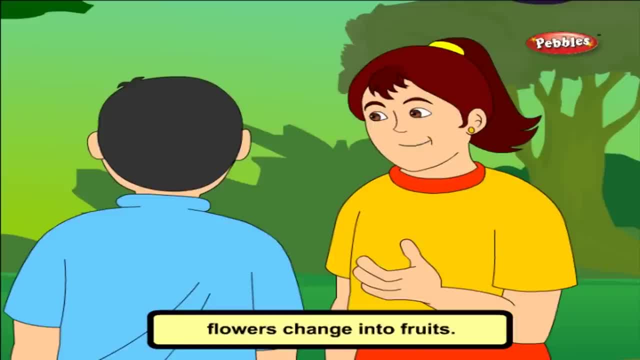 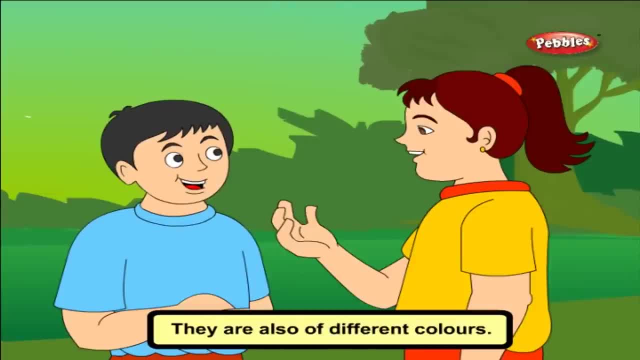 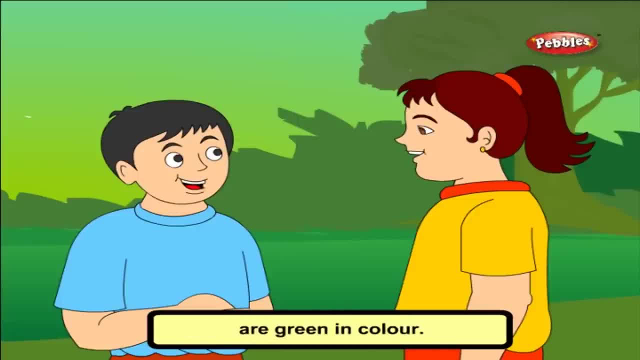 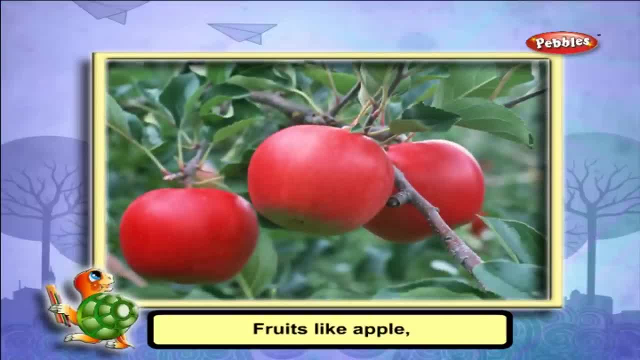 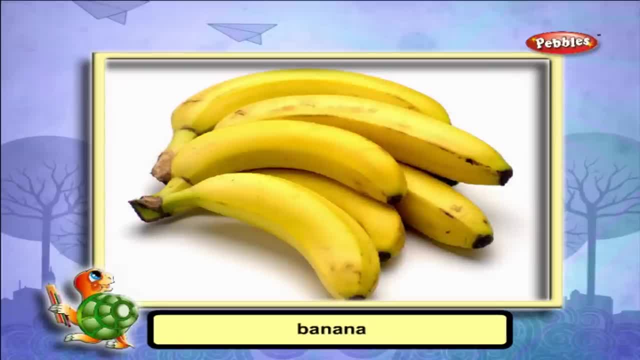 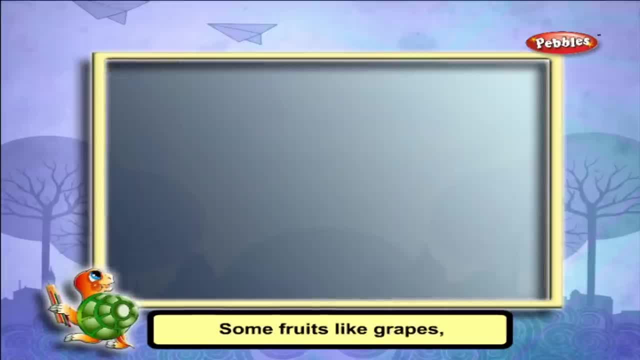 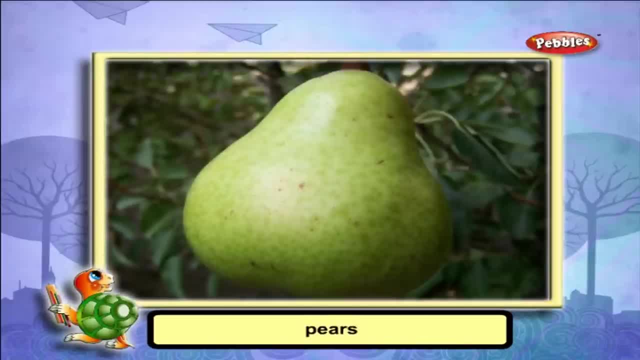 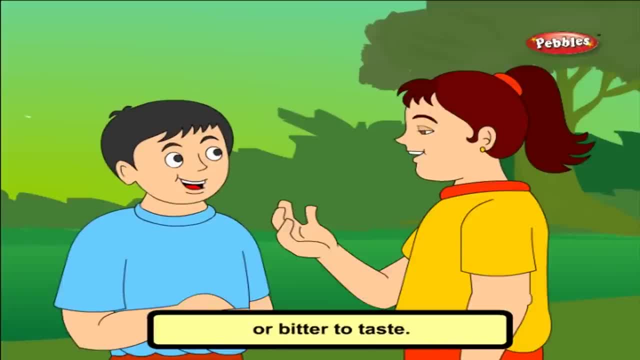 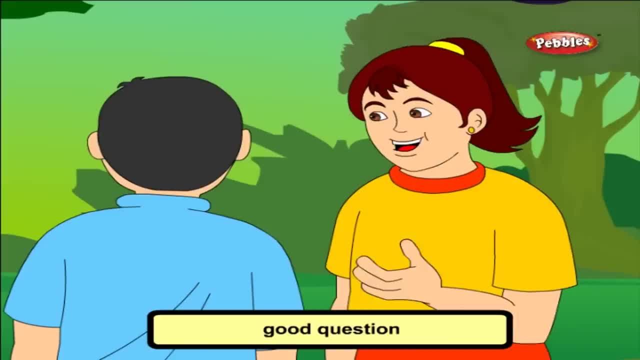 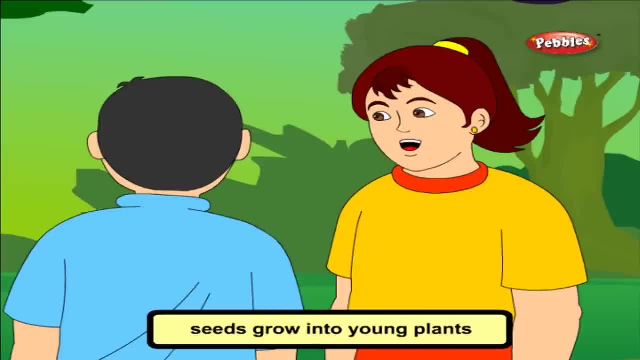 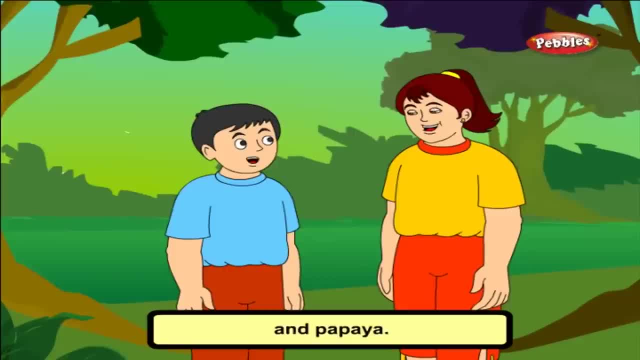 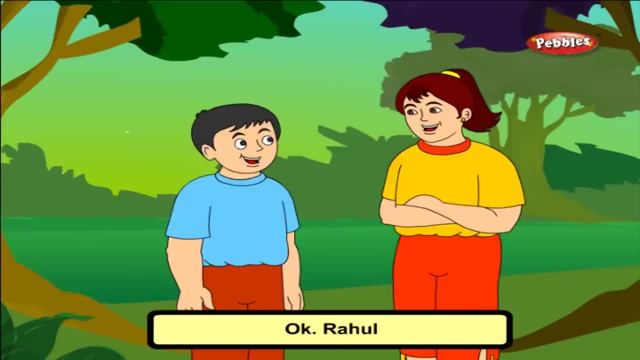 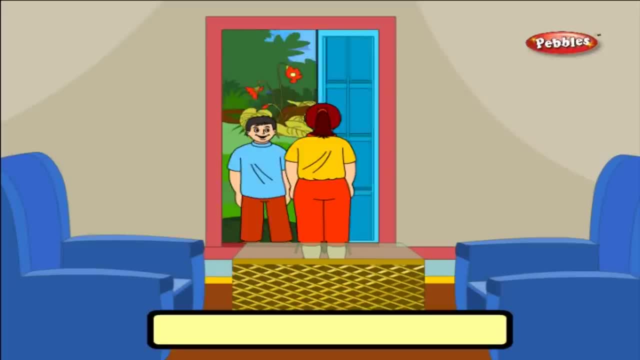 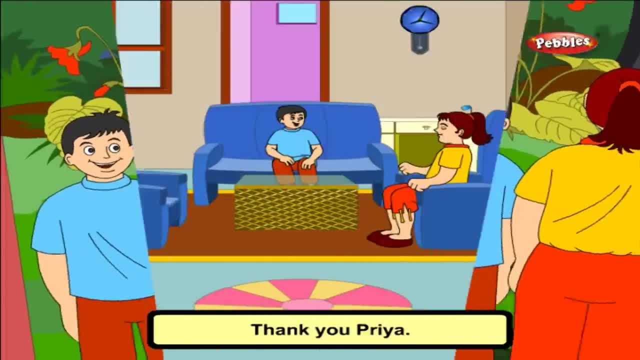 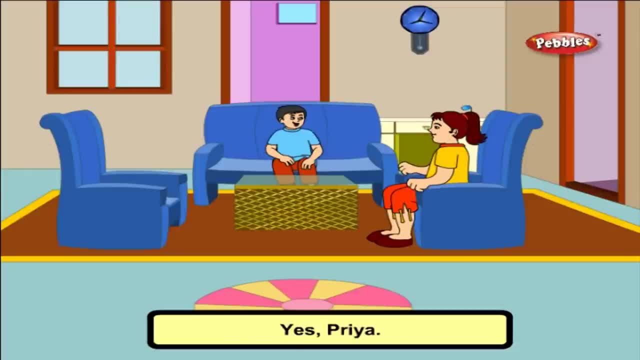 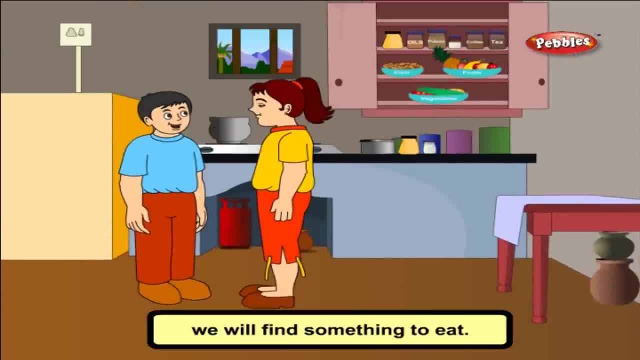 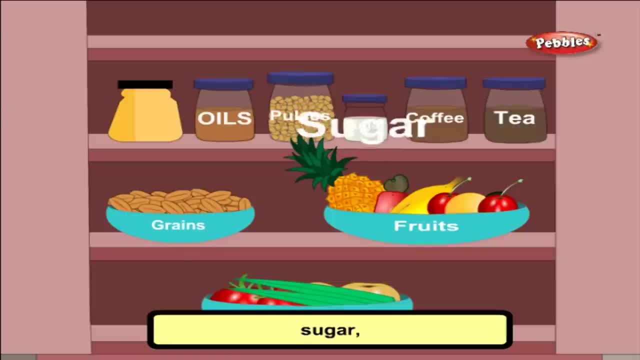 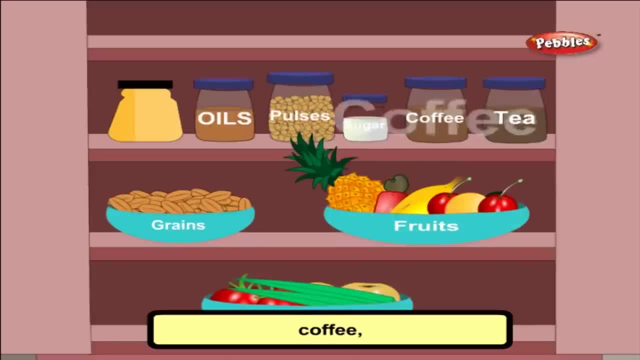 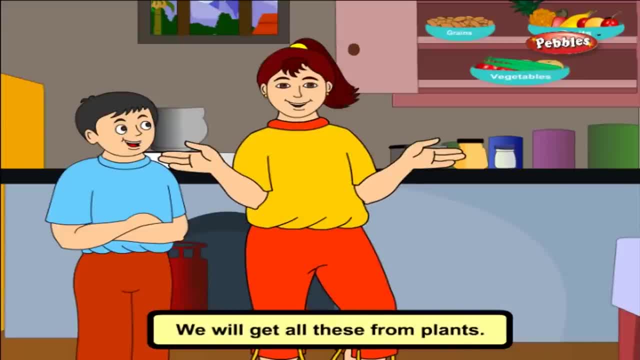 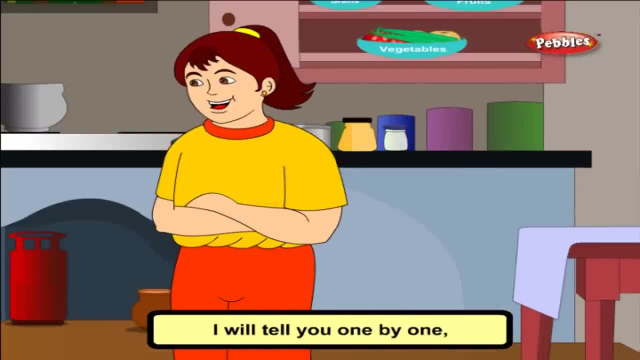 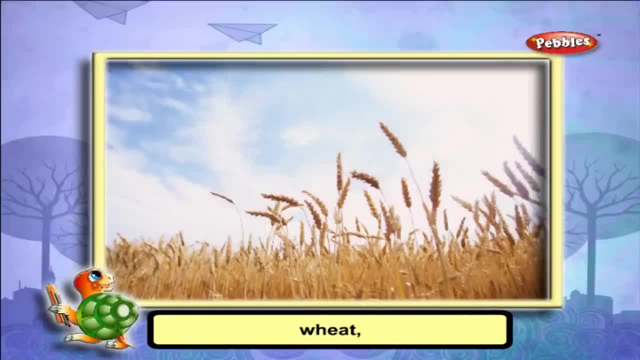 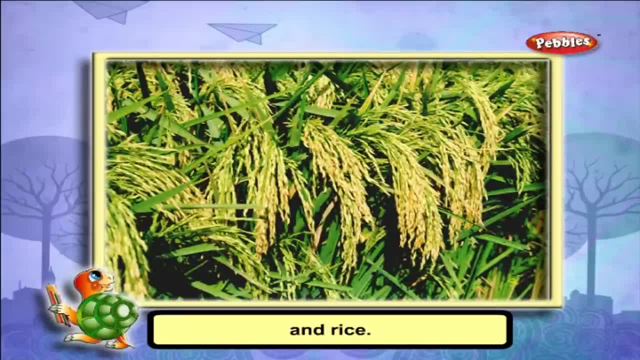 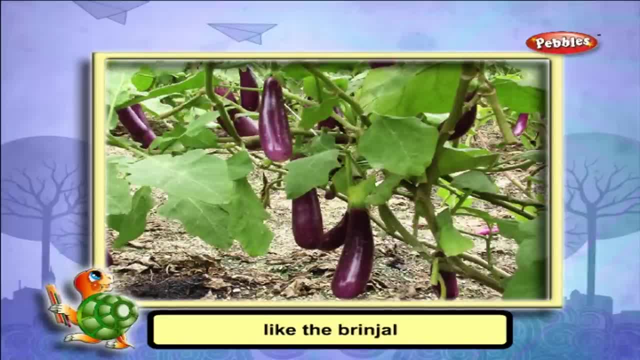 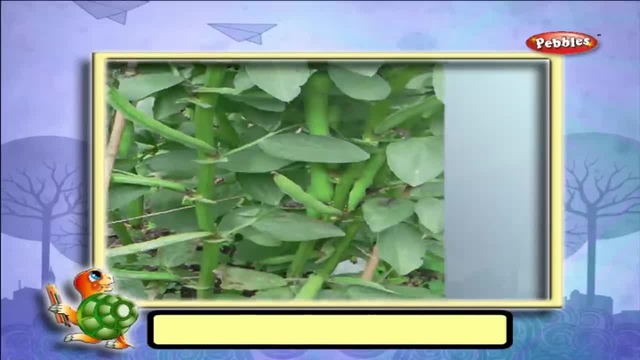 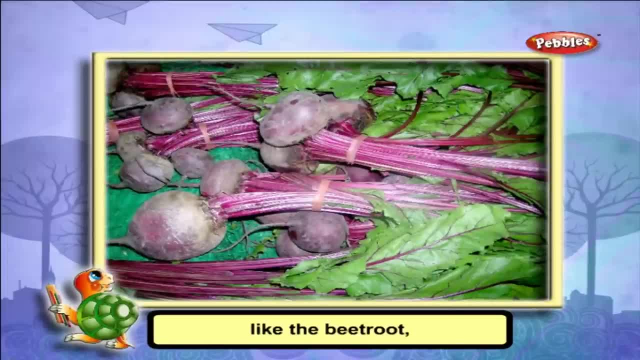 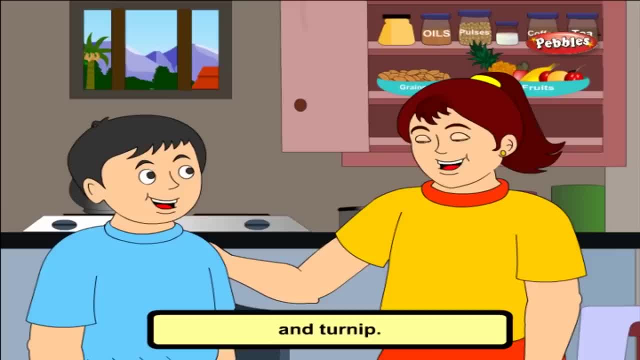 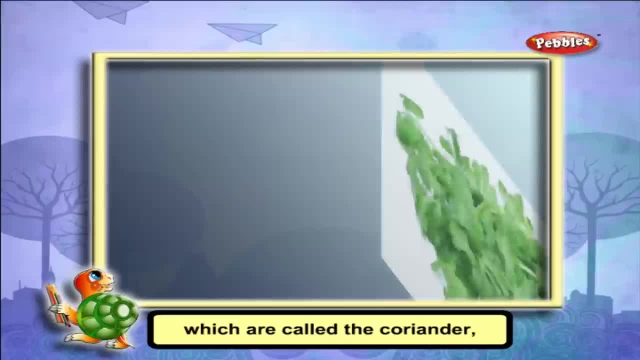 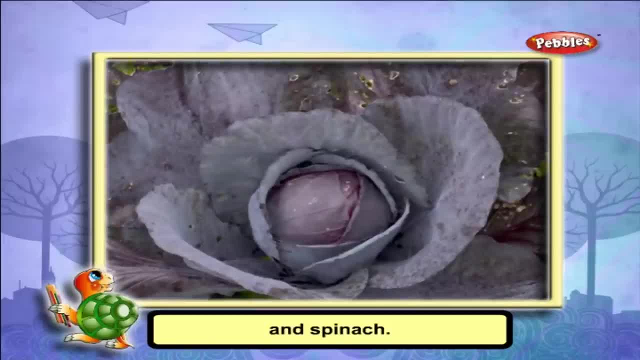 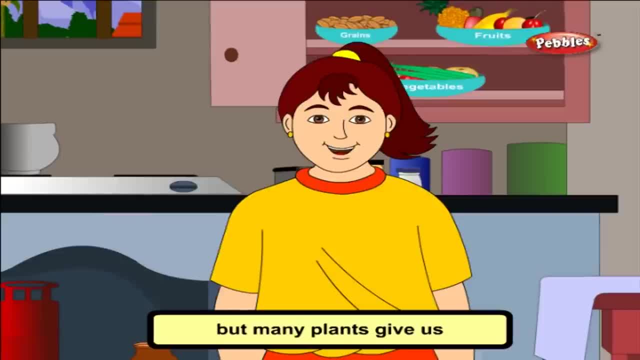 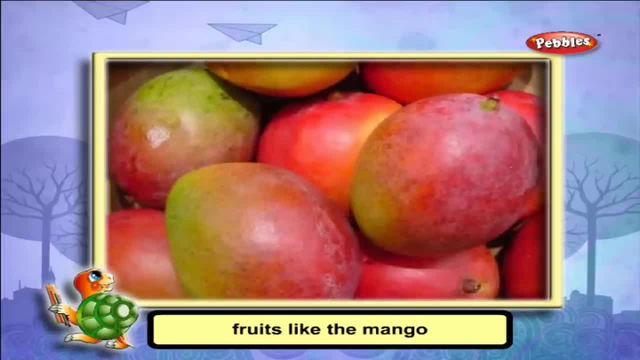 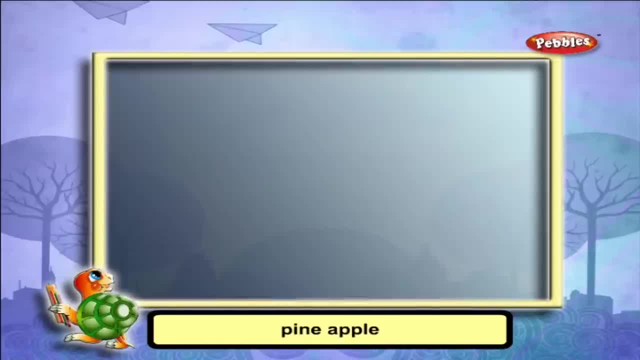 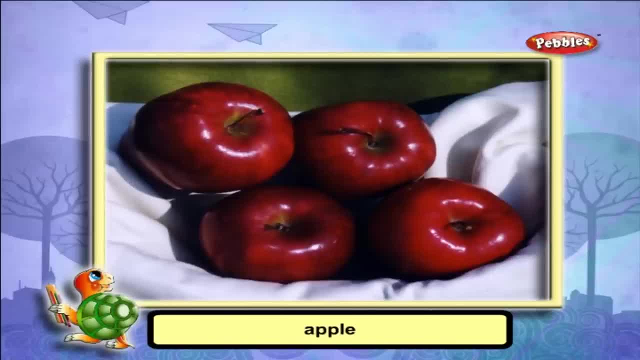 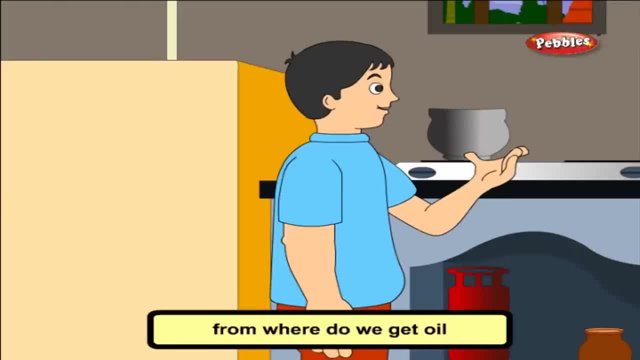 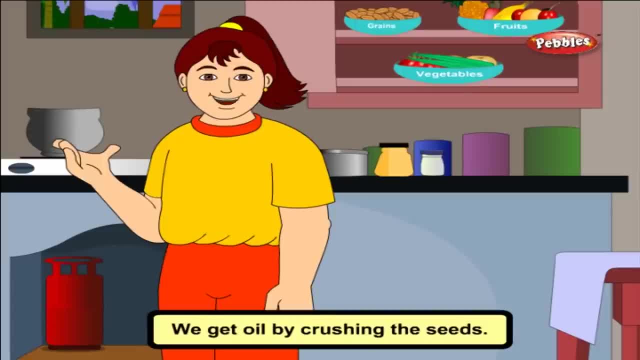 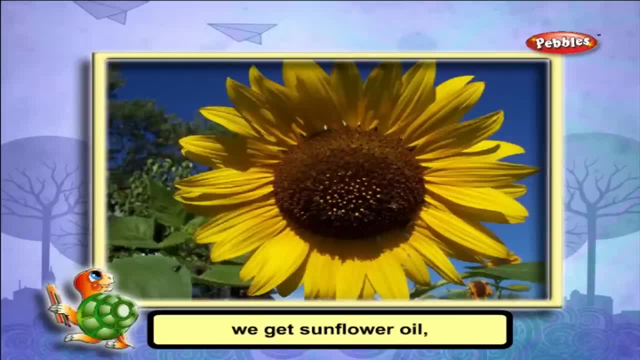 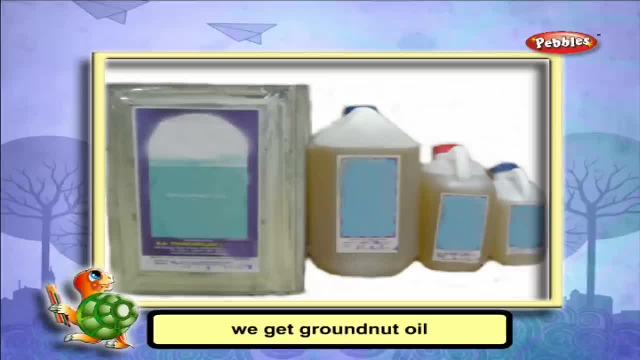 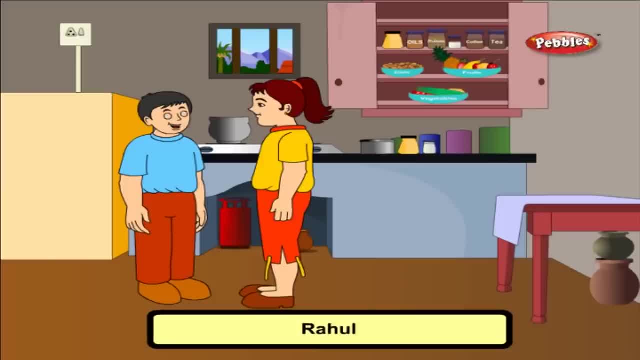 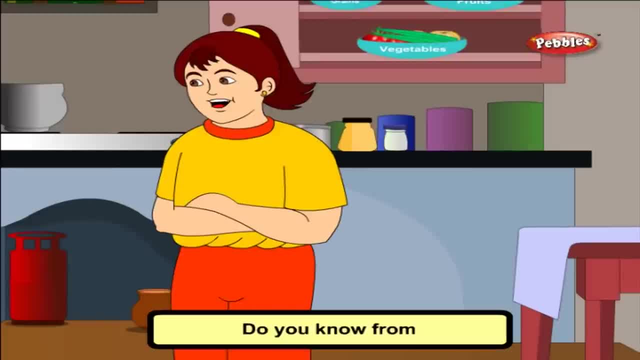 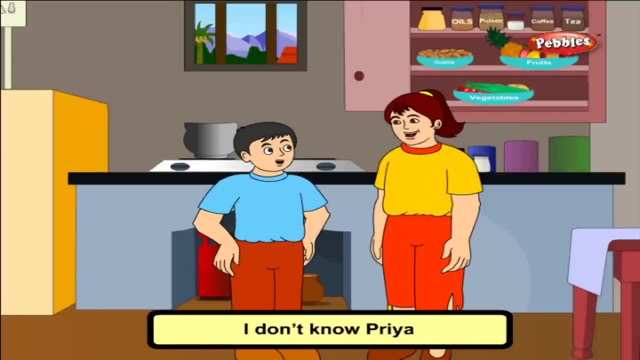 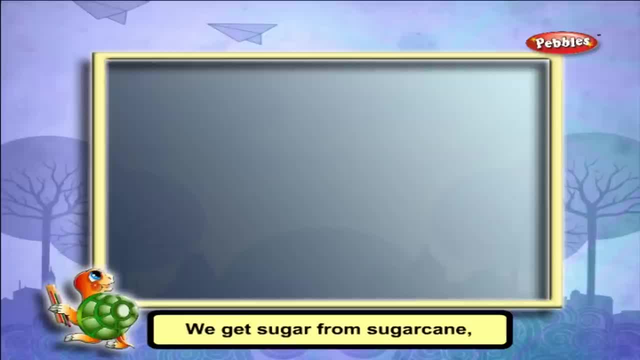 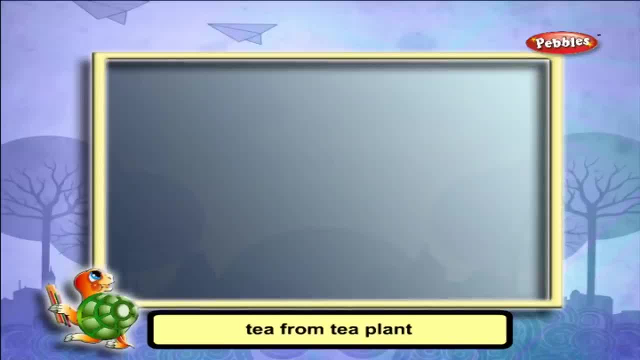 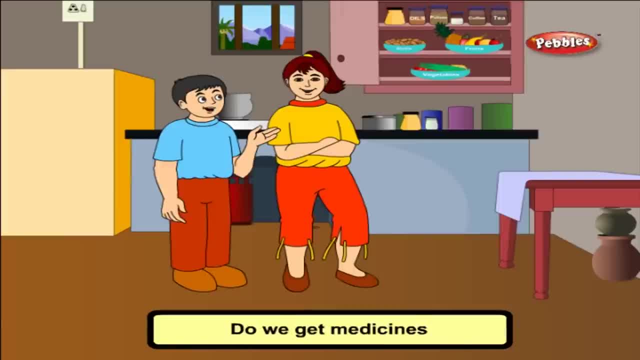 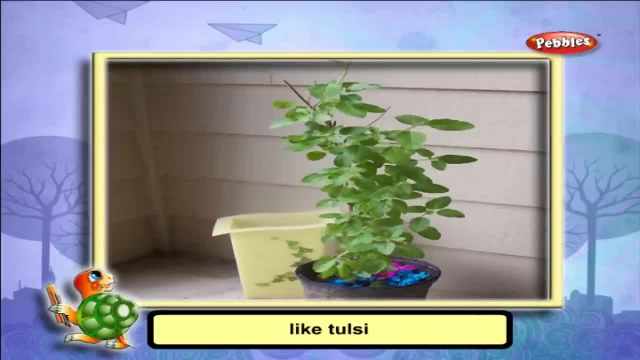 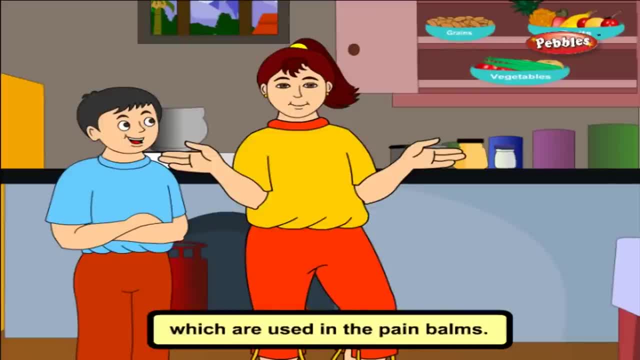 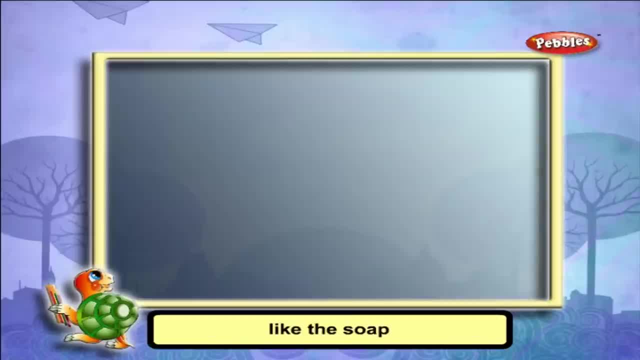 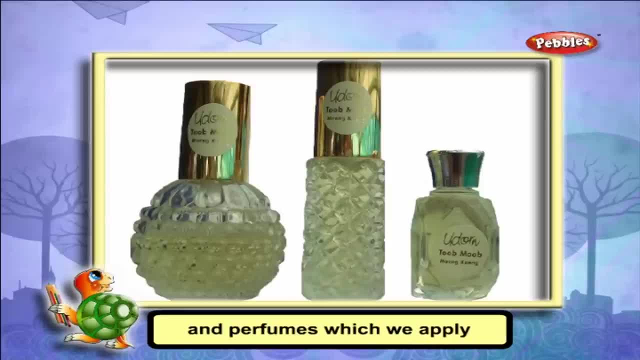 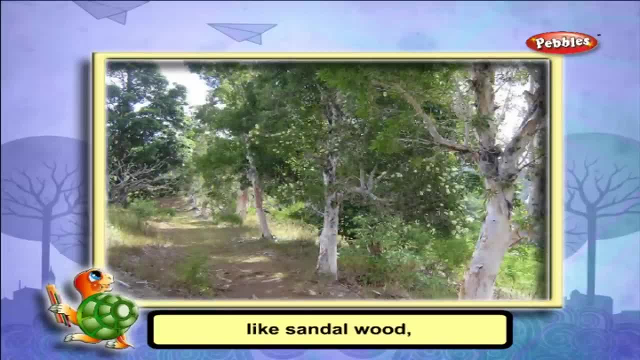 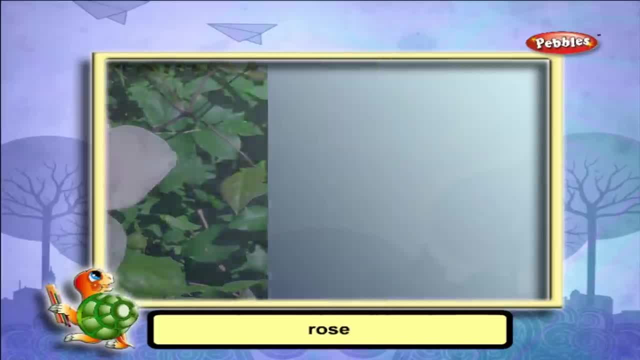 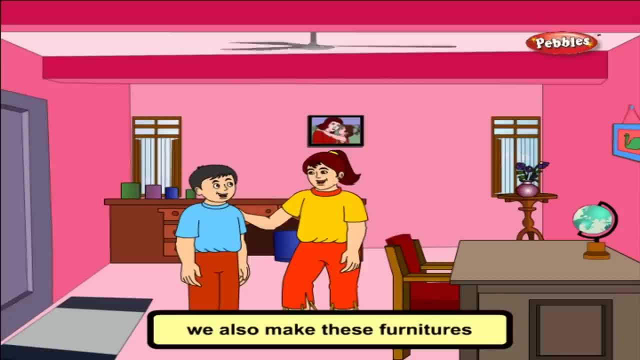 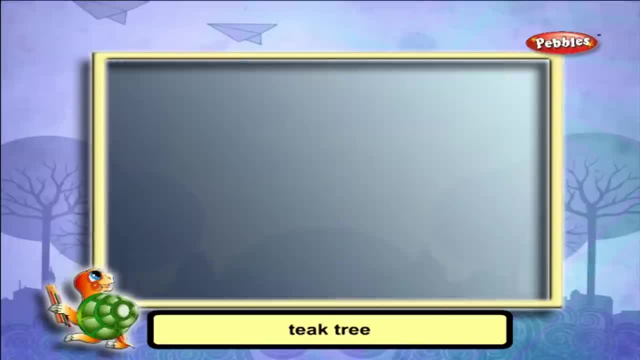 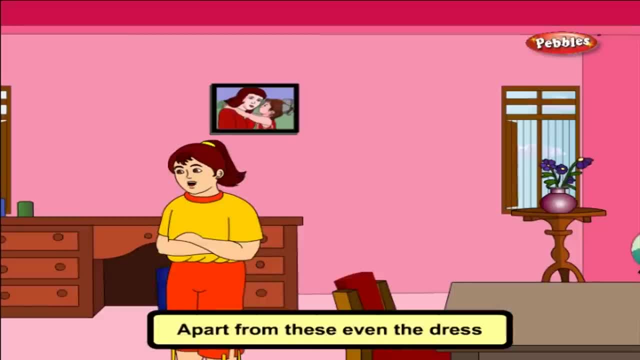 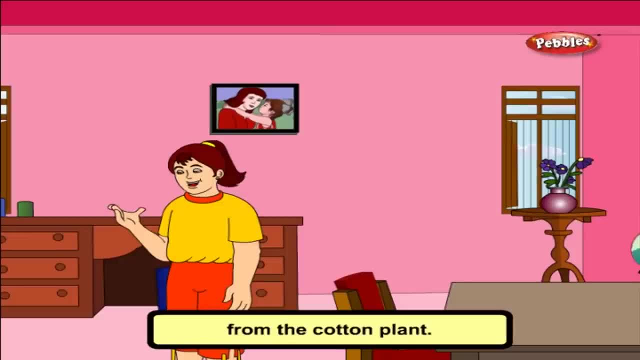 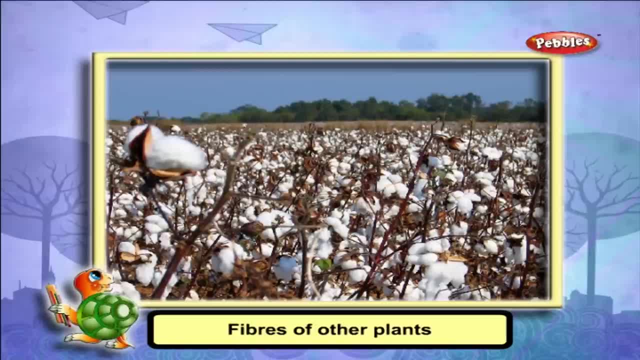 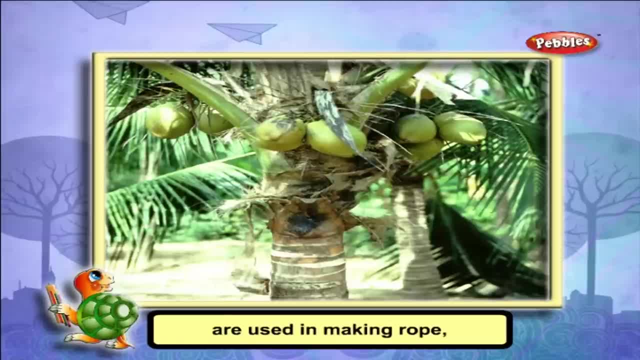 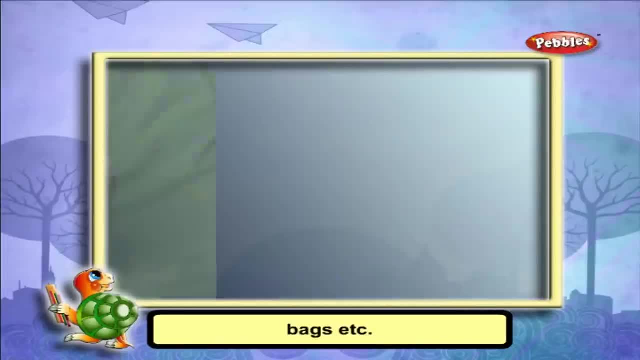 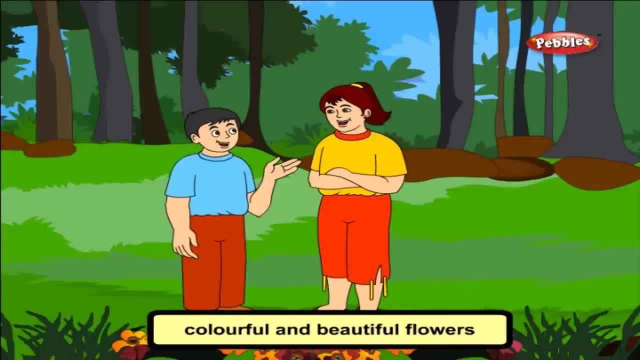 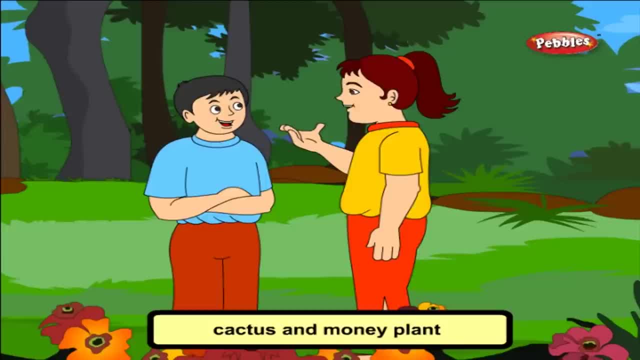 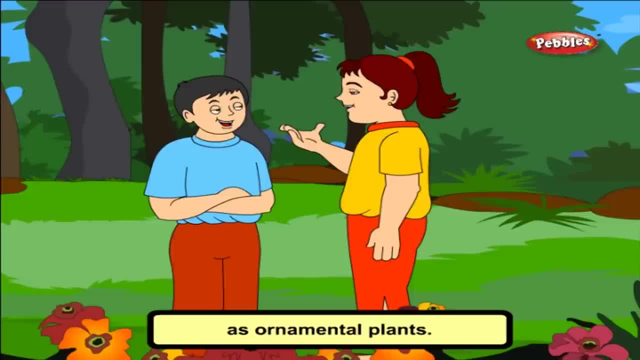 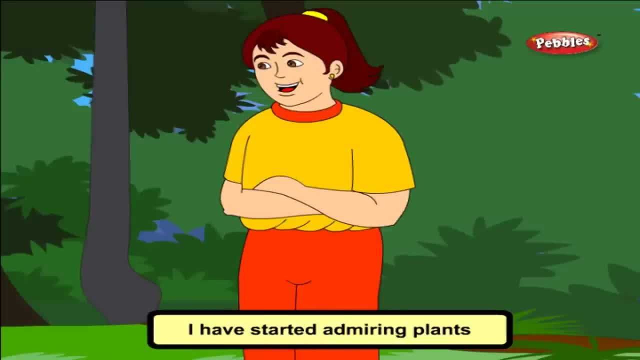 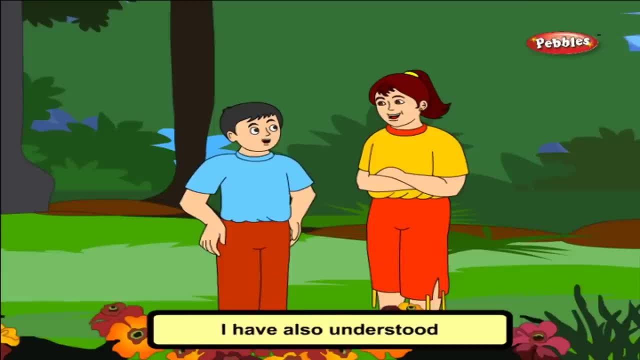 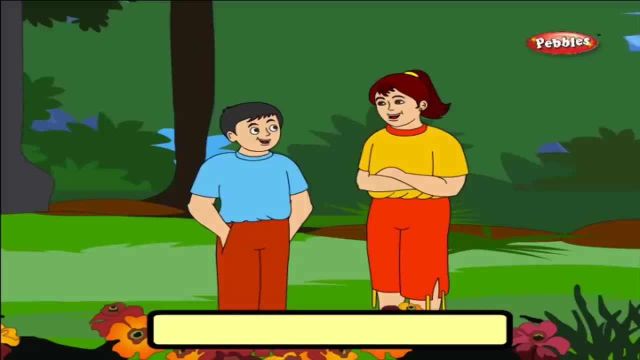 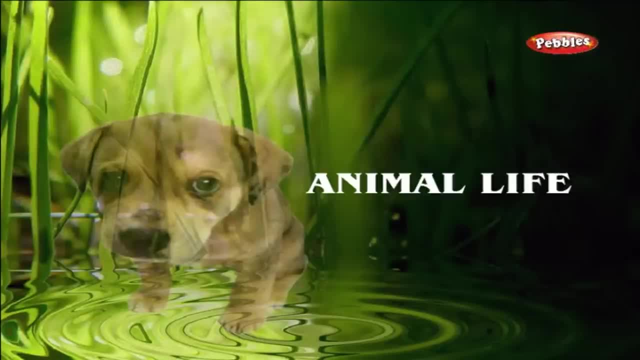 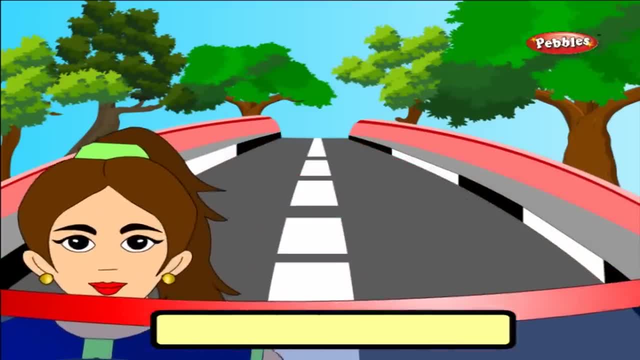 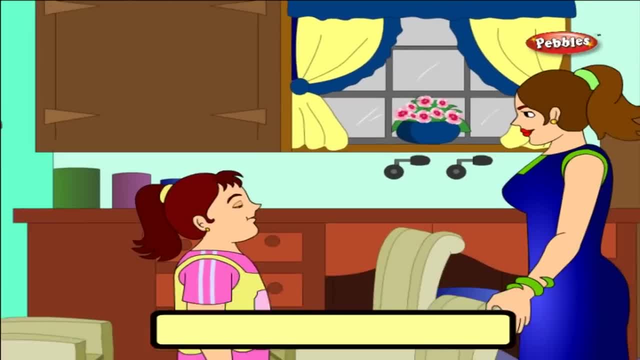 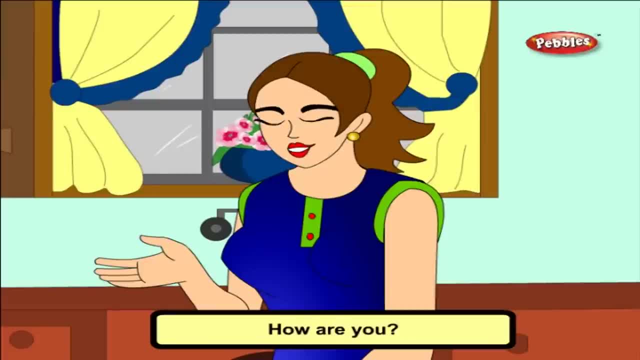 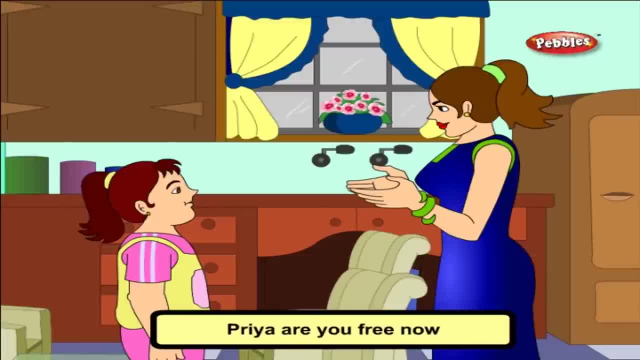 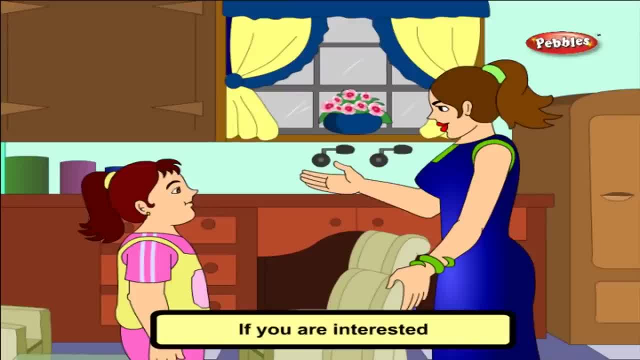 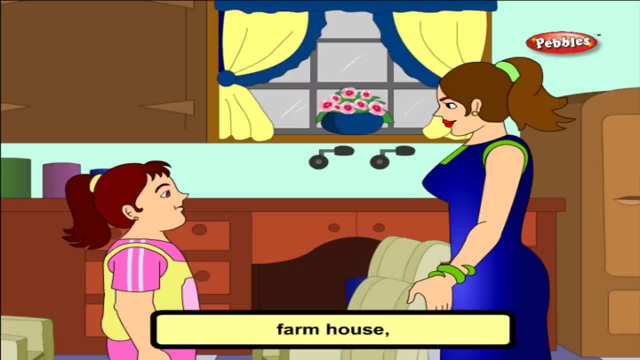 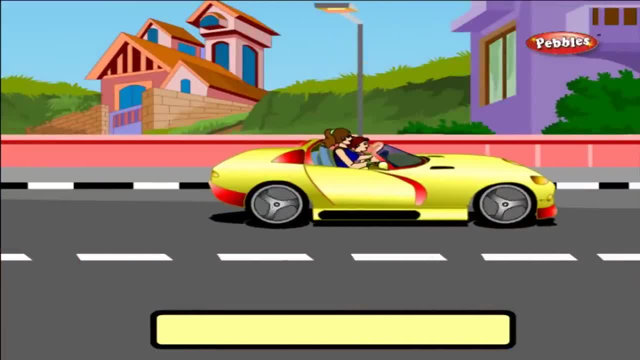 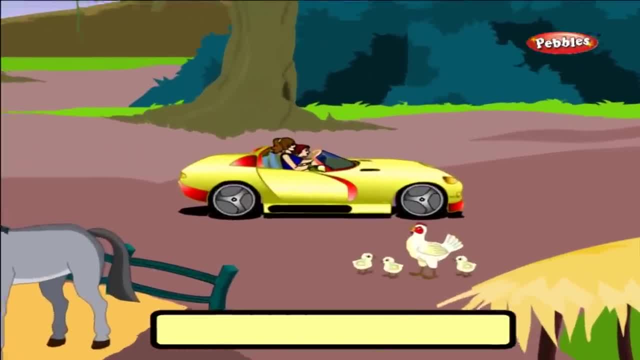 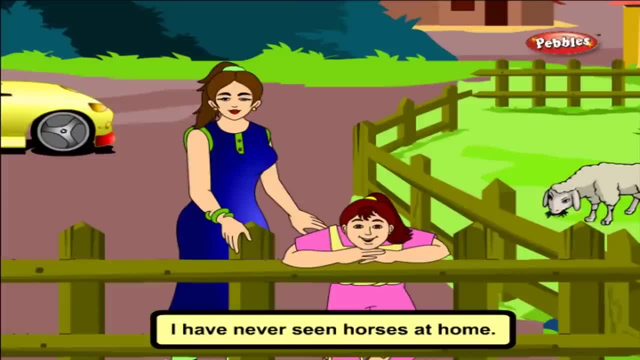 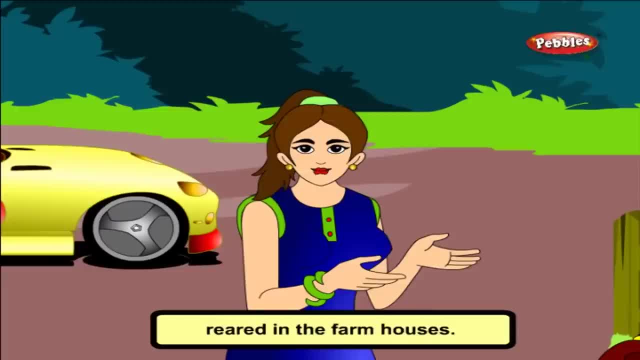 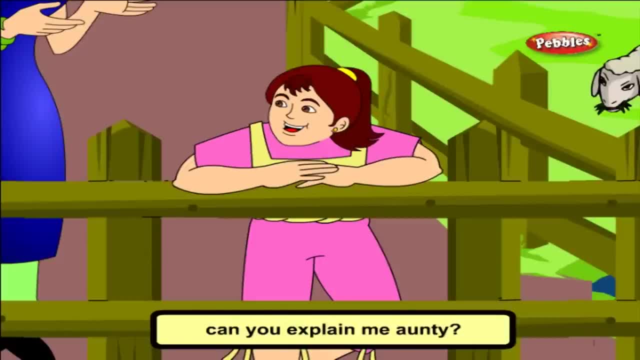 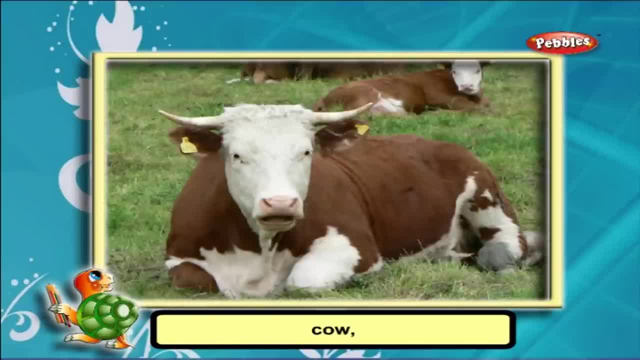 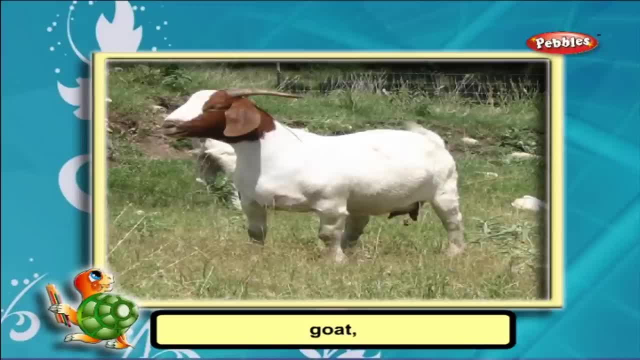 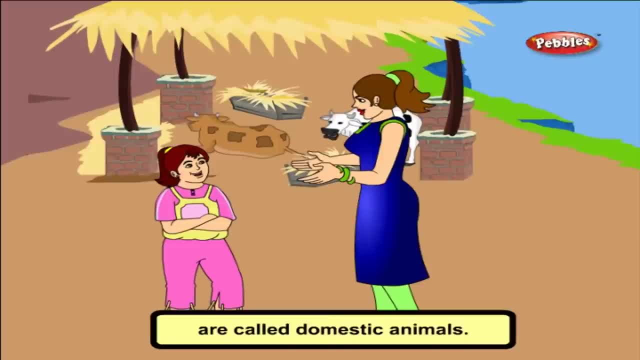 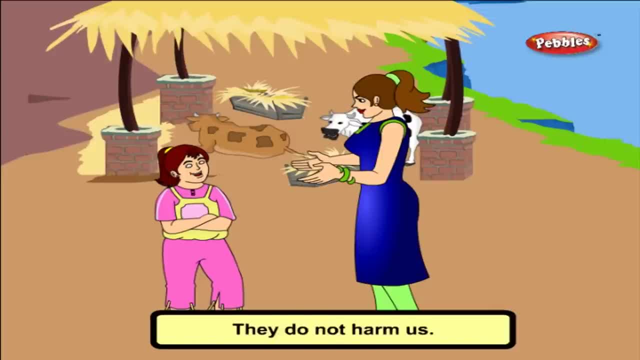 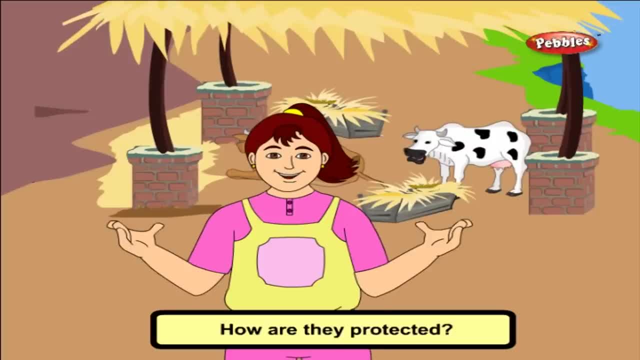 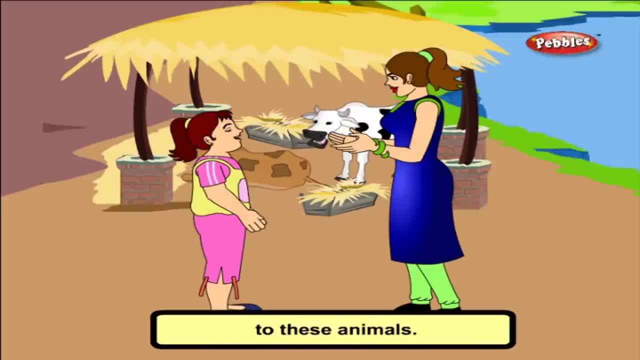 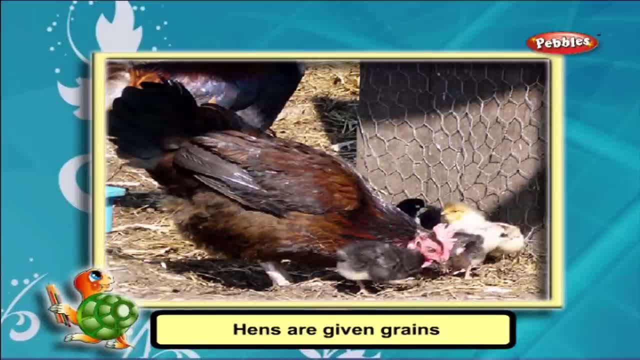 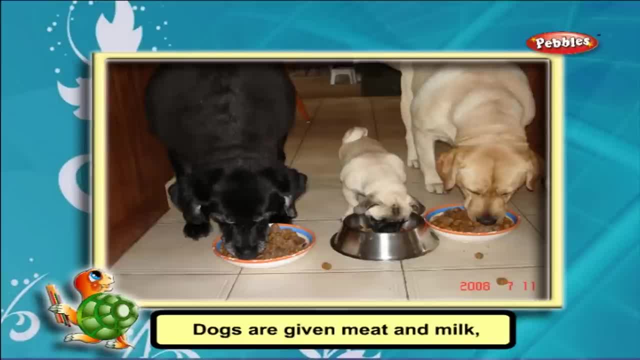 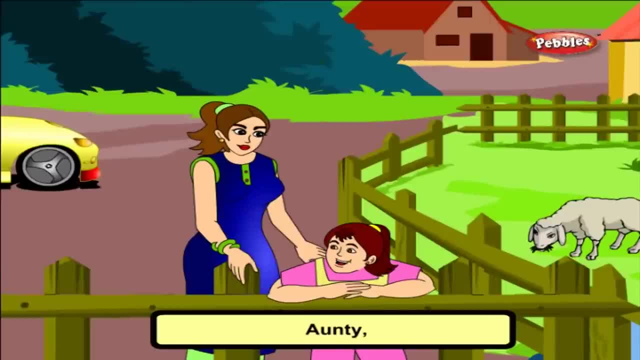 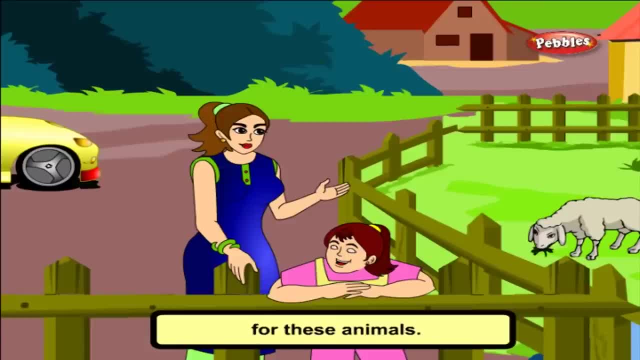 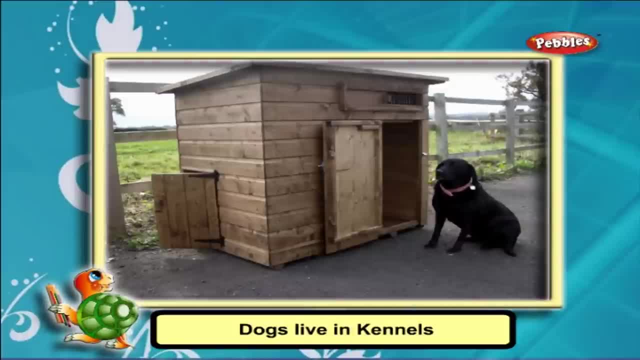 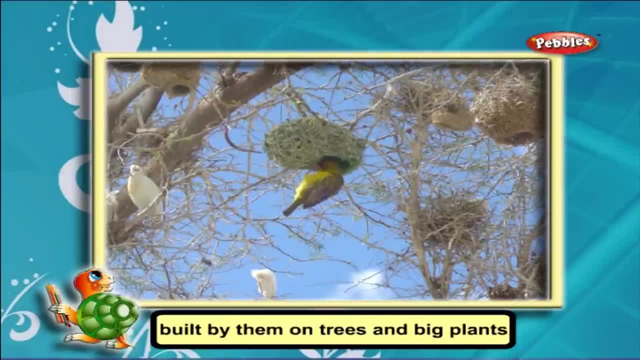 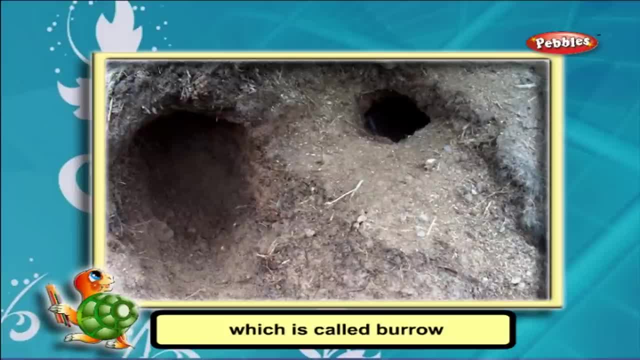 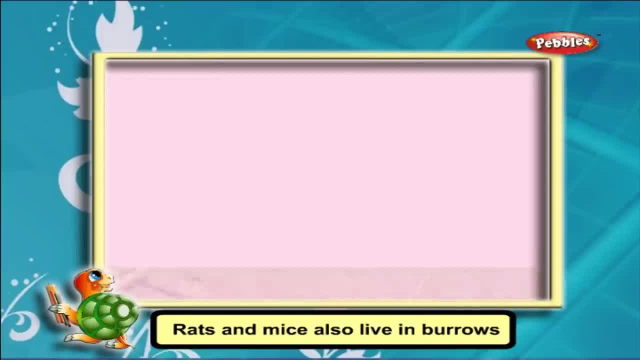 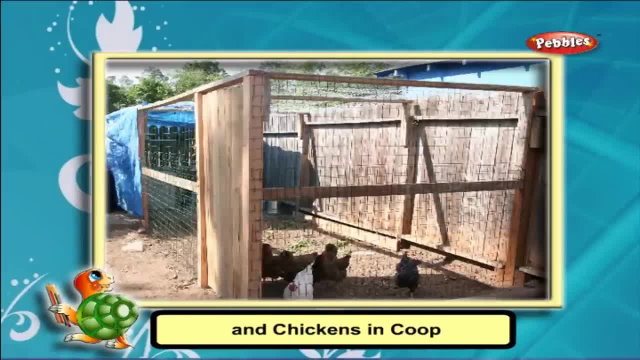 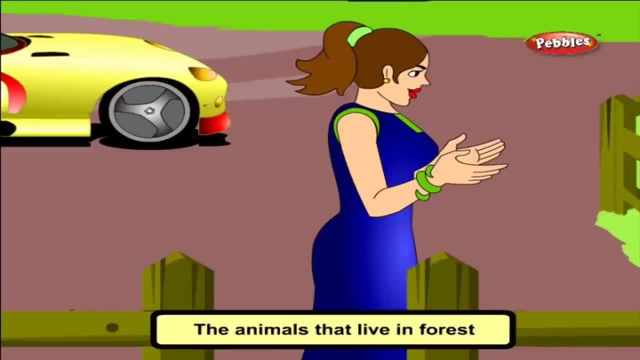 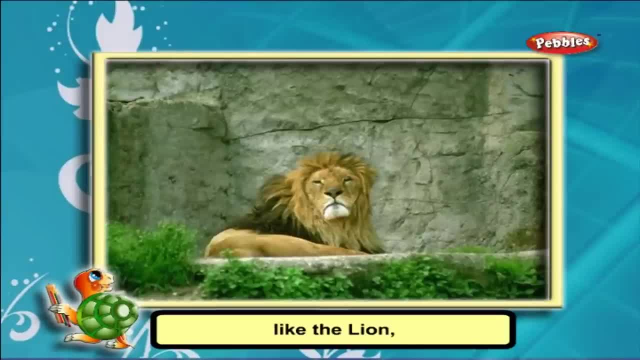 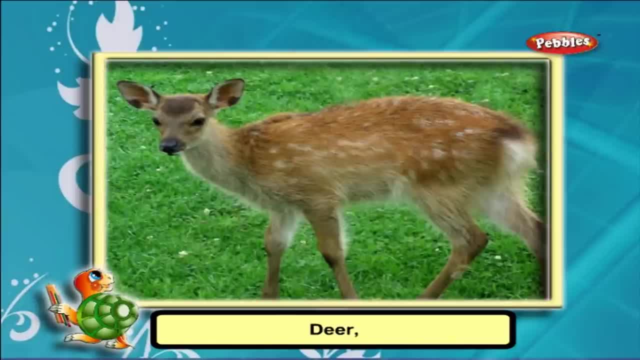 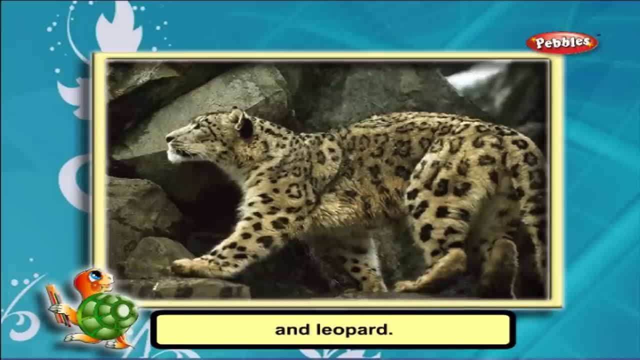 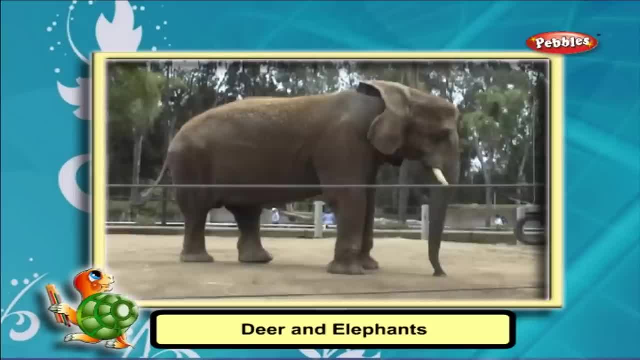 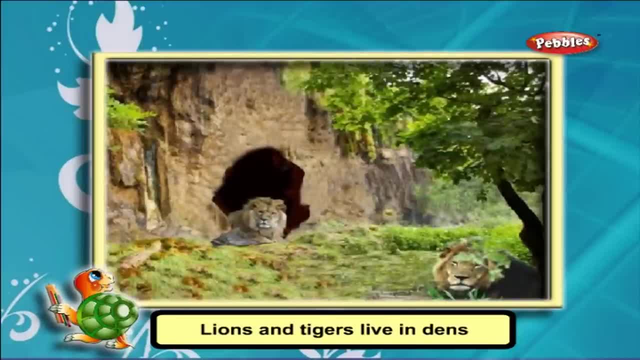 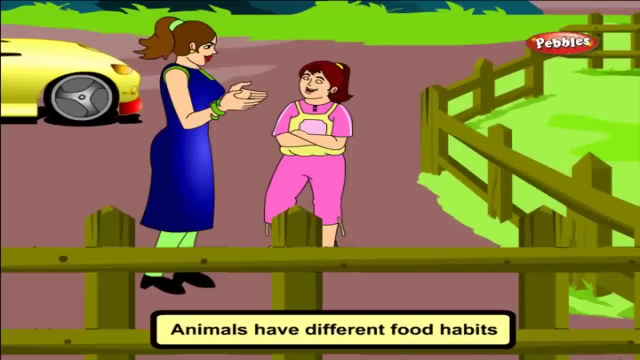 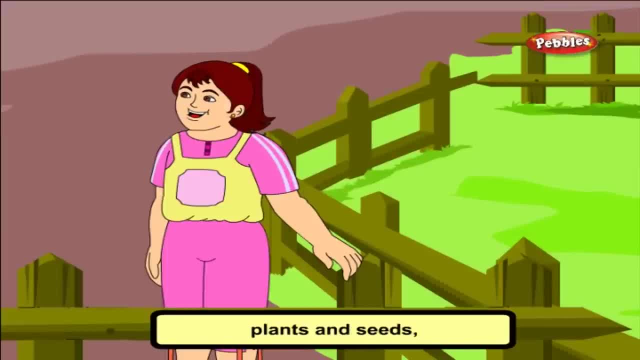 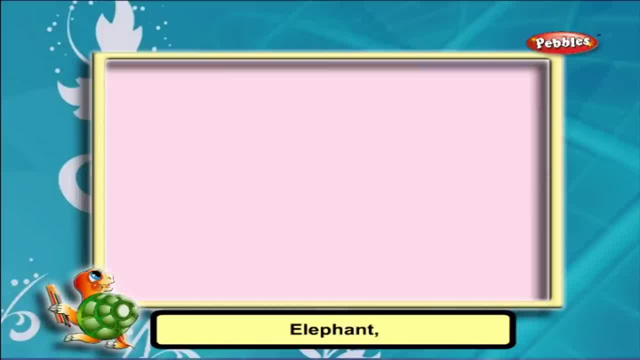 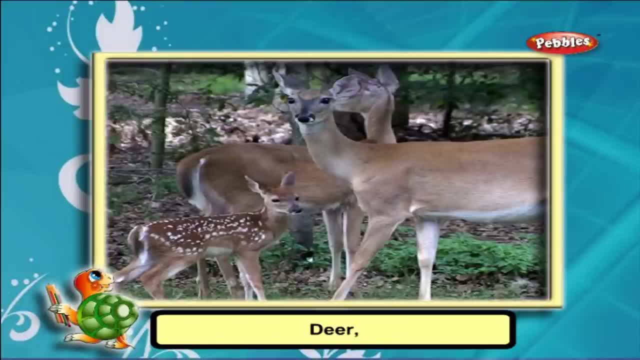 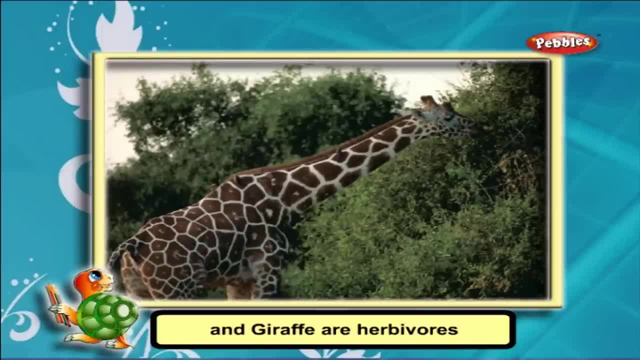 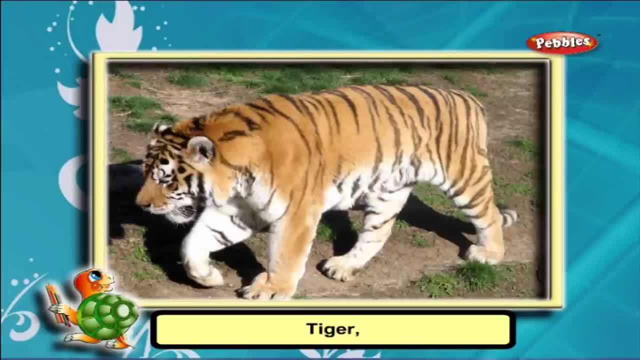 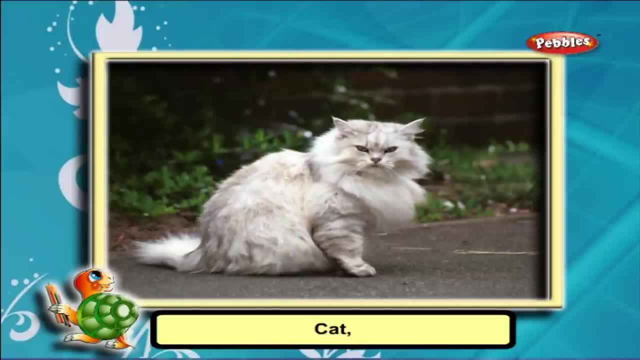 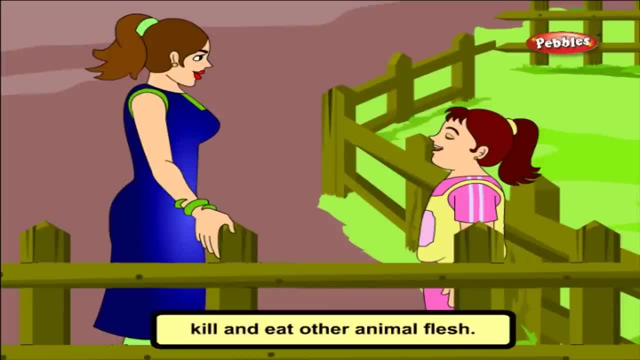 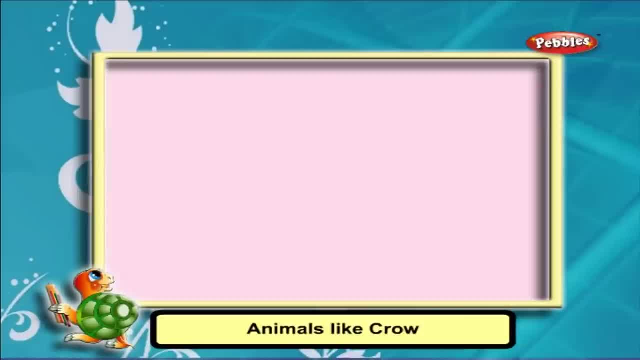 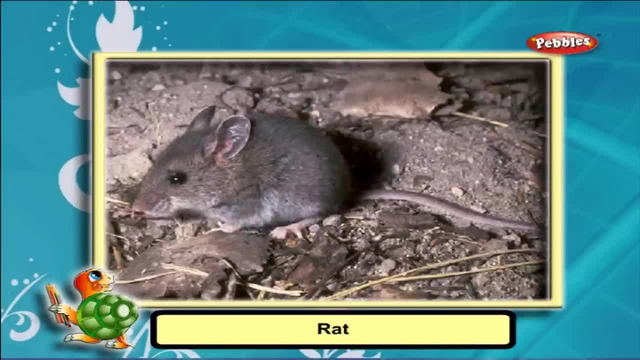 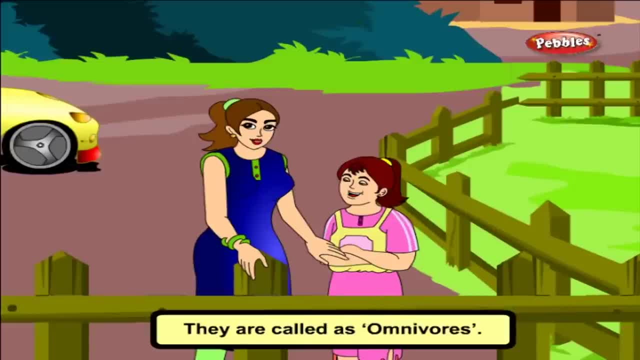 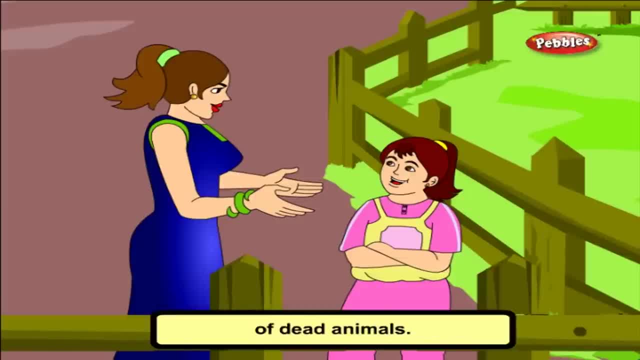 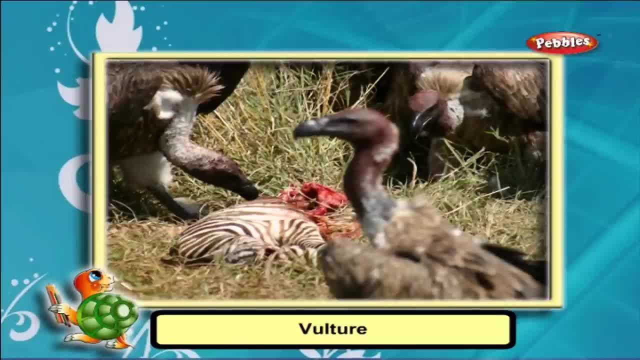 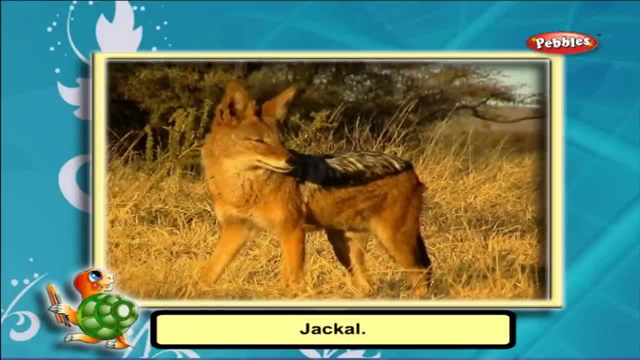 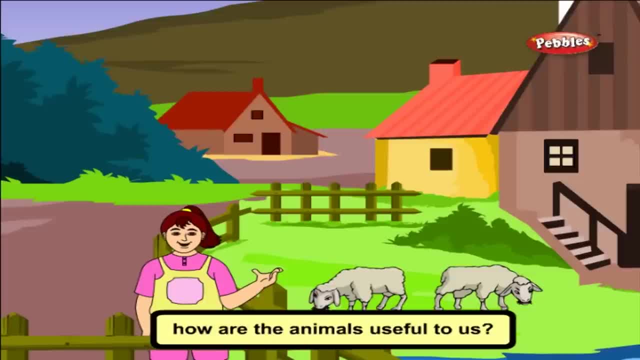 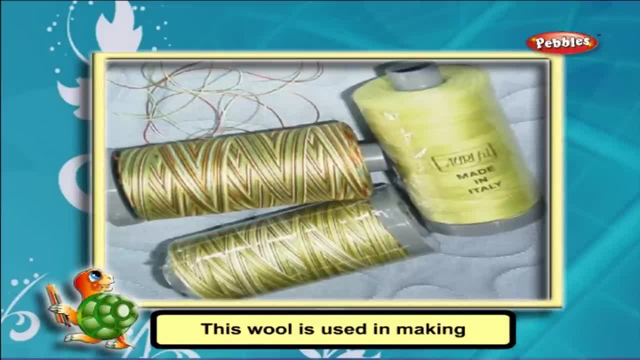 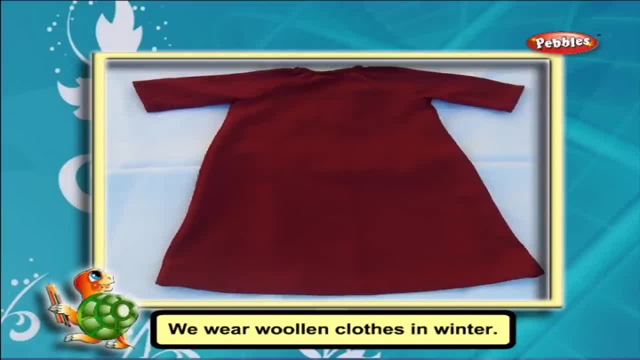 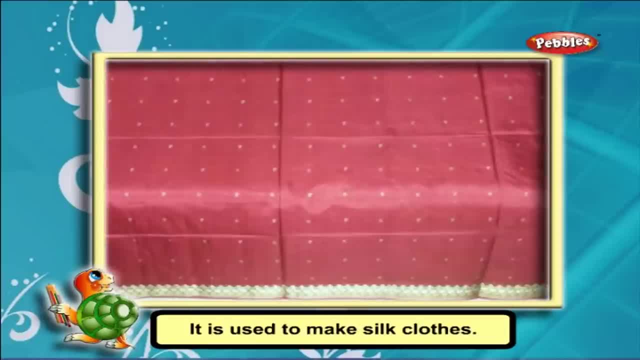 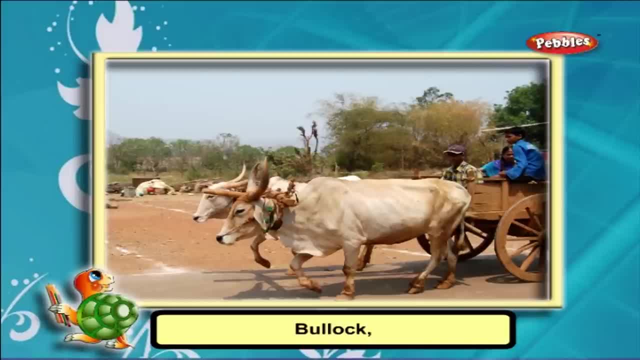 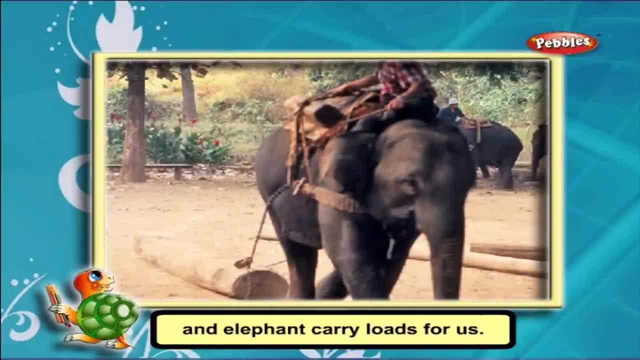 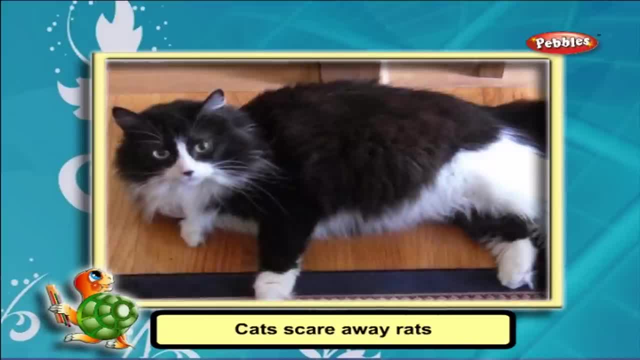 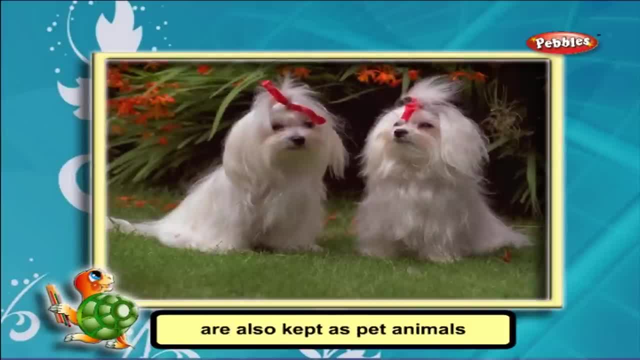 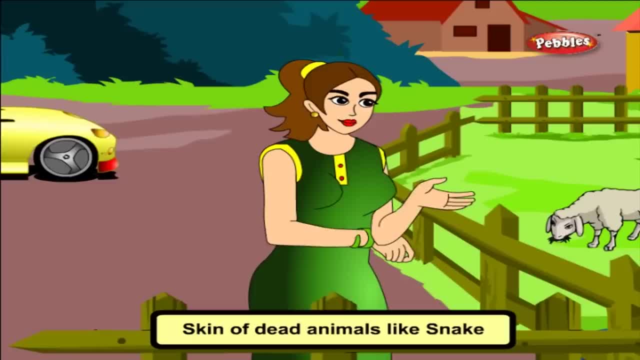 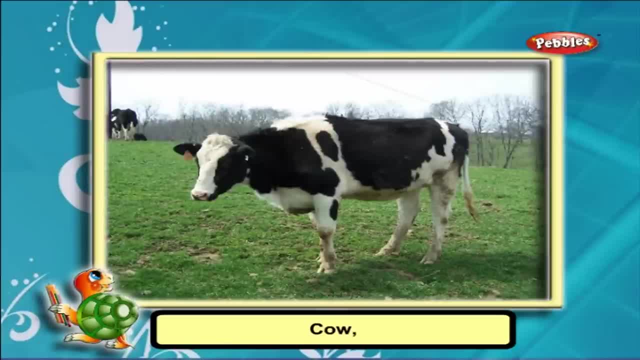 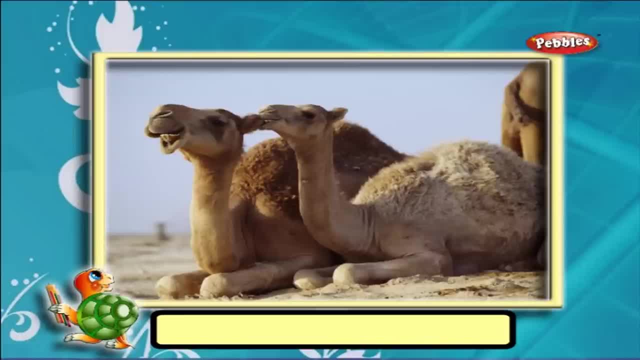 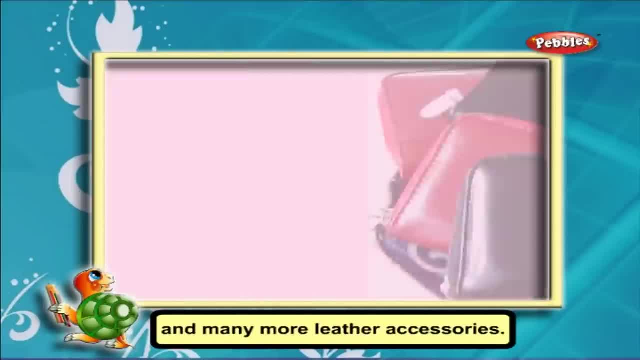 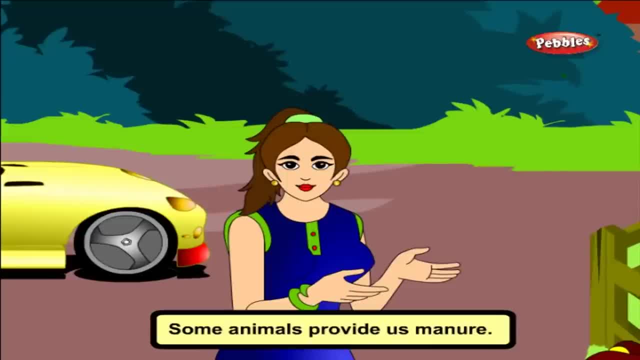 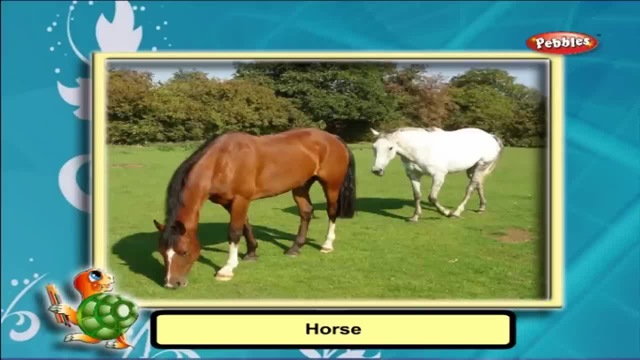 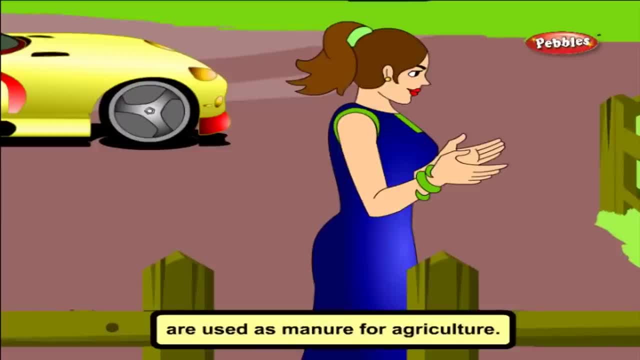 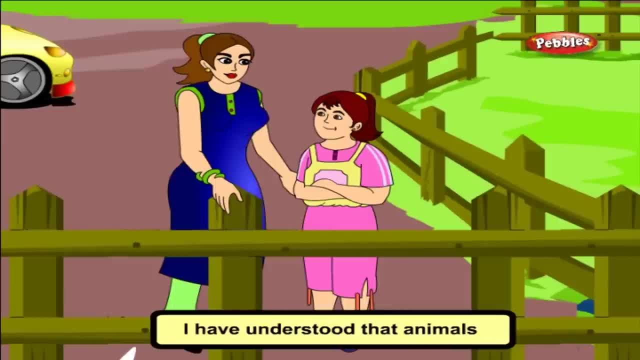 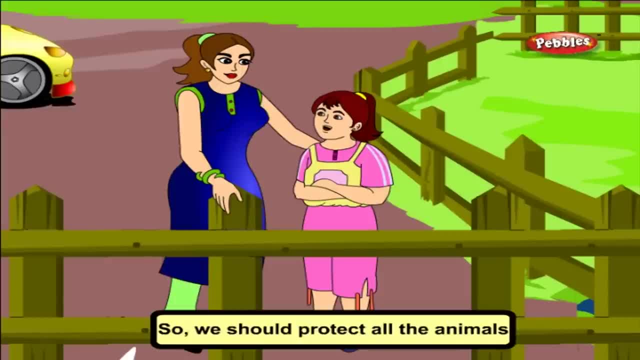 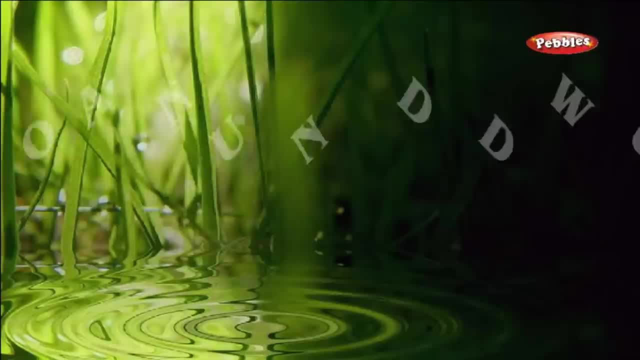 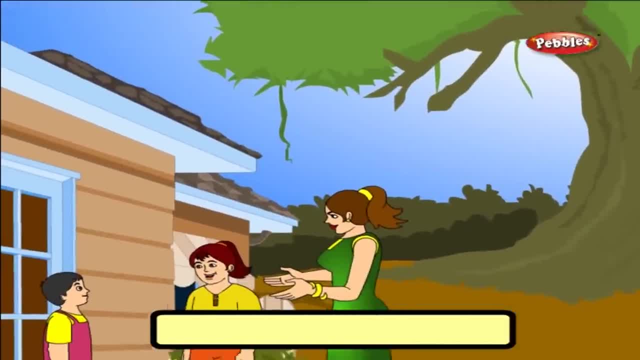 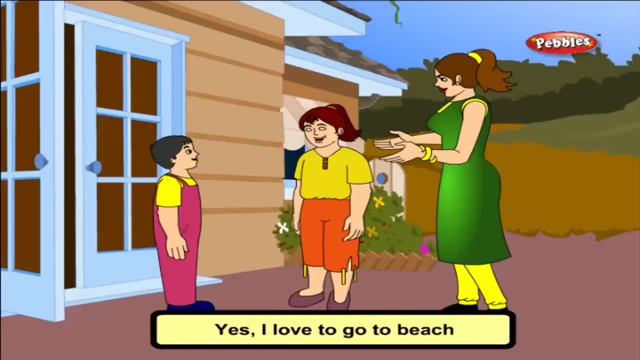 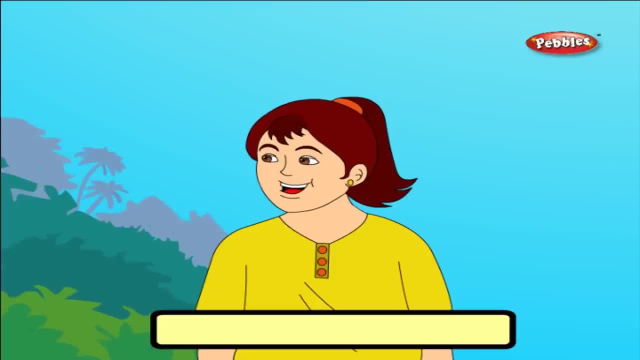 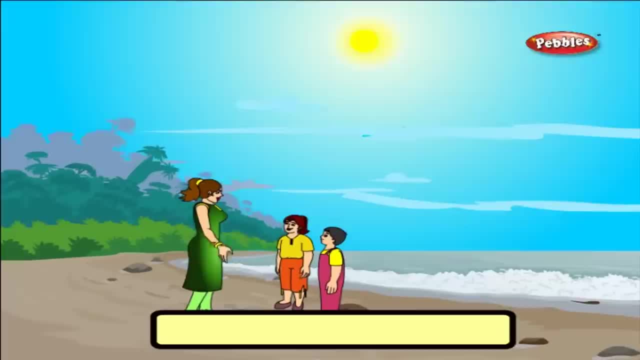 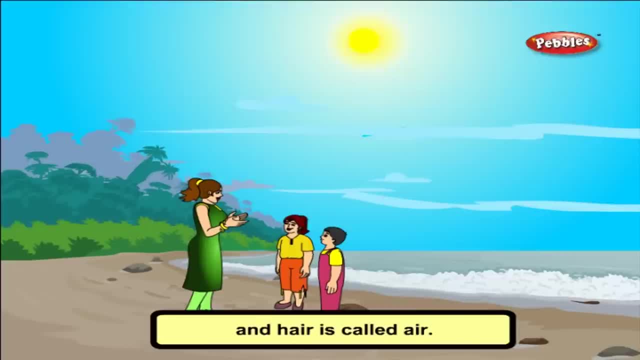 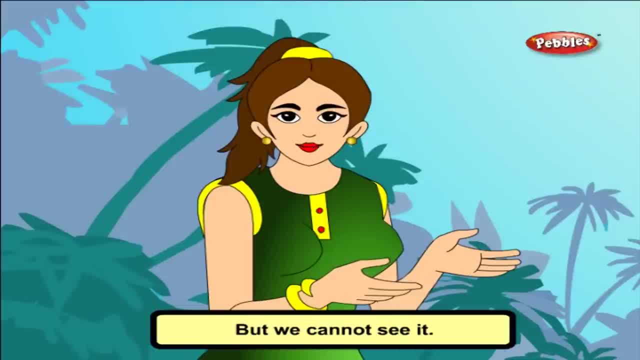 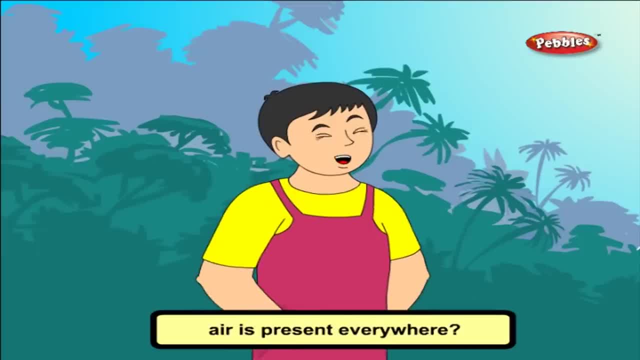 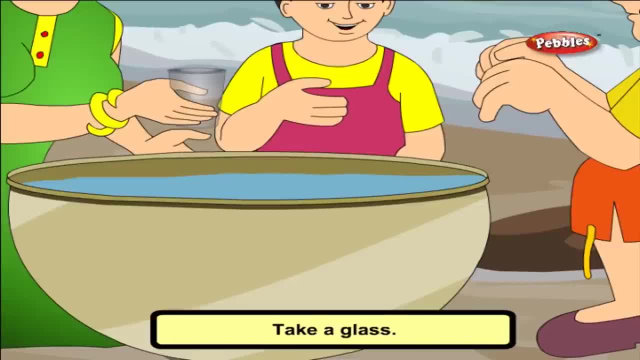 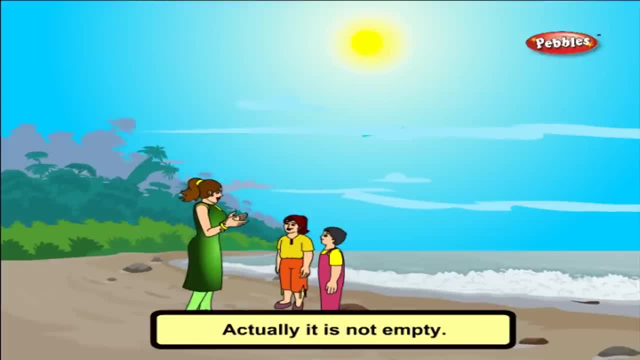 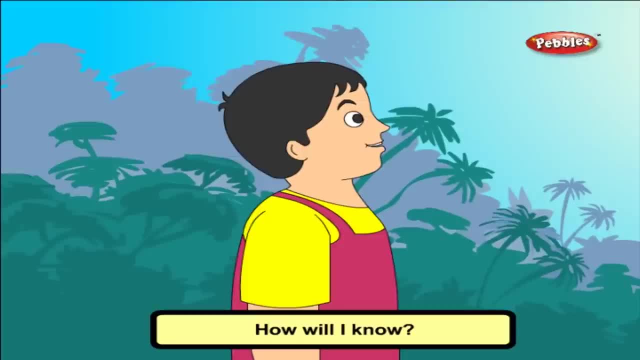 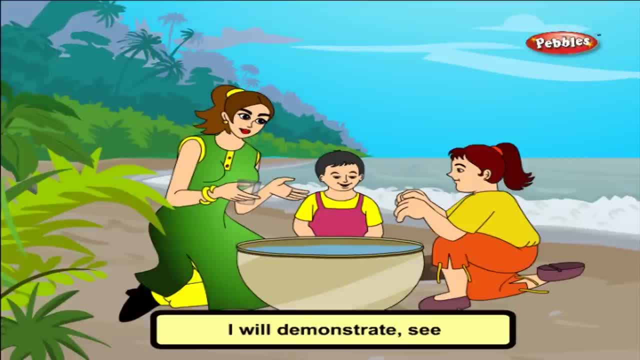 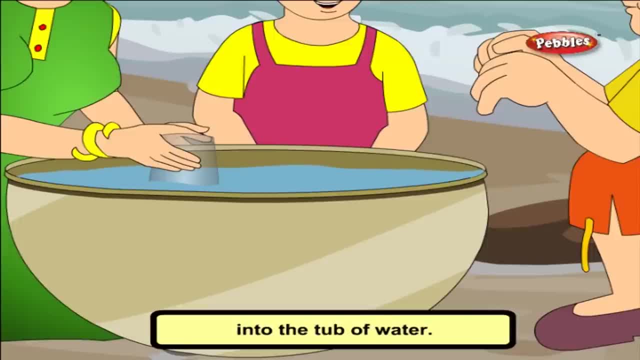 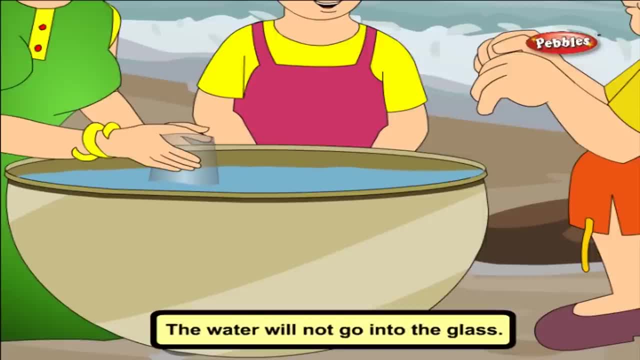 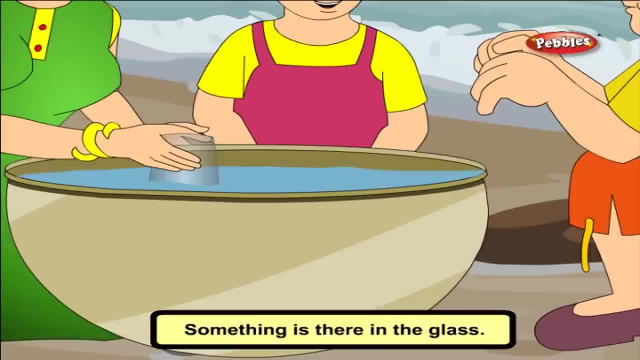 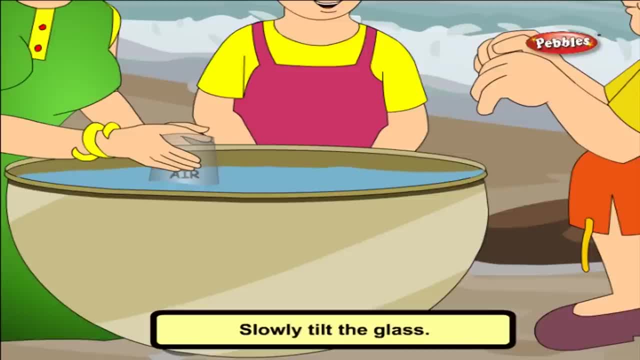 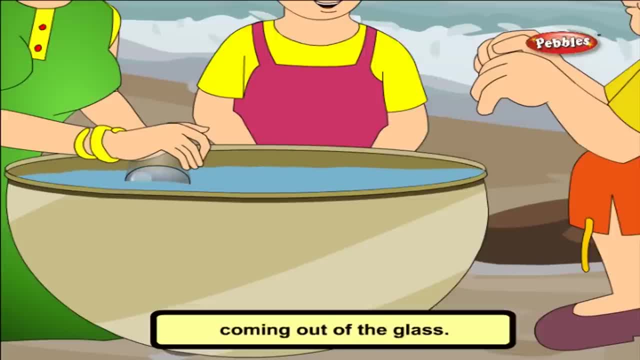 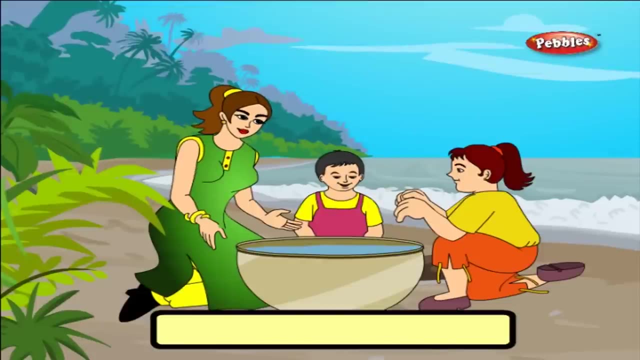 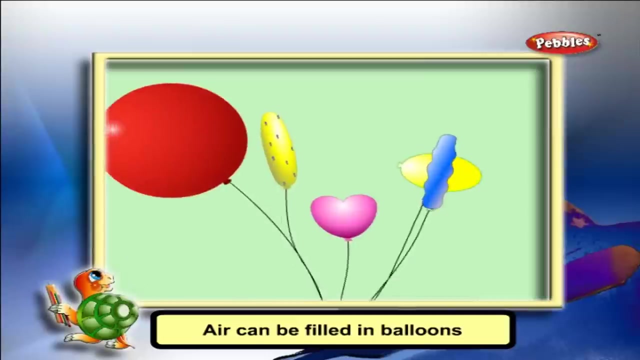 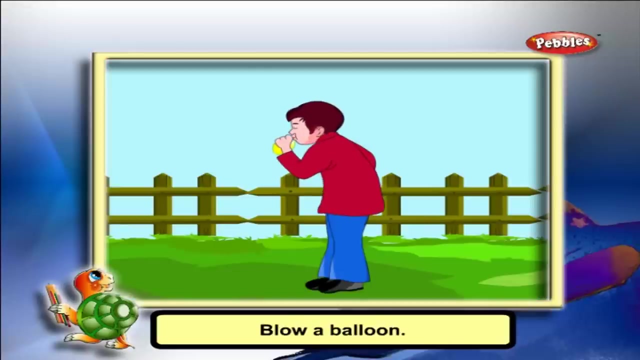 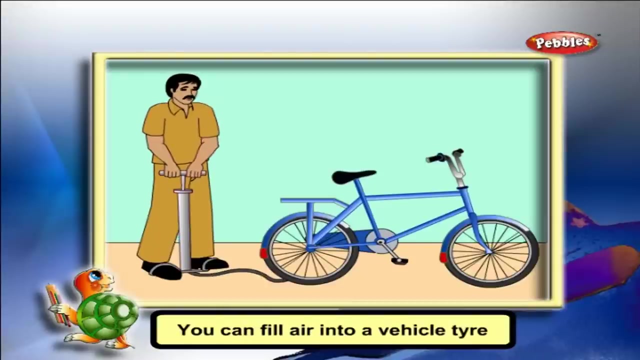 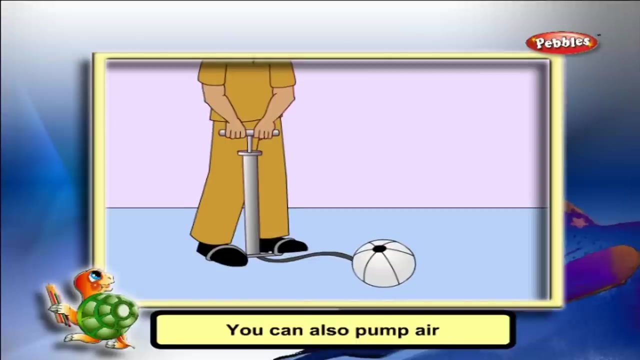 Thank you for watching the video. Please subscribe to the channel and give it a high rating. Blow a balloon. the balloon becomes big, Why it gets filled up with air. you can fill air into a vehicle tire With an air pump. you can also pump air into the football. 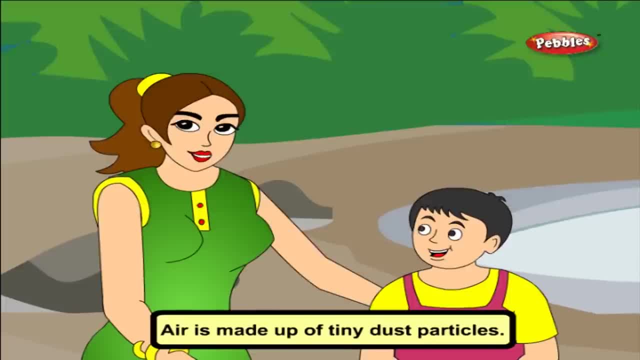 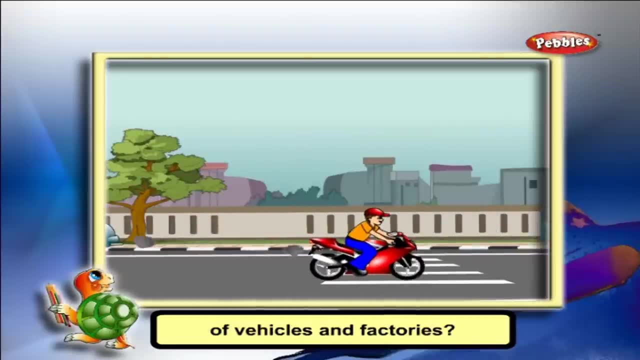 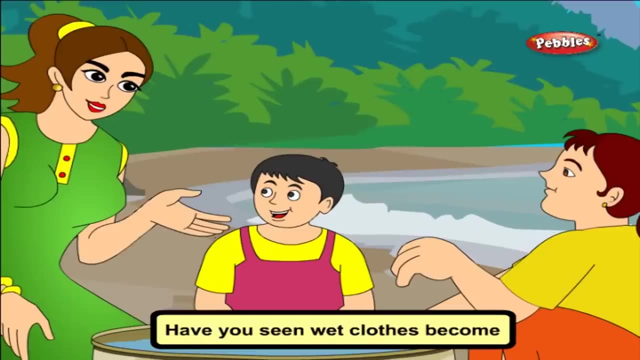 What does air made up of? air is made up of tiny dust particles. Have you seen smoke coming out of vehicles and factories? Where does the smoke go? it gets mixed with the air. Have you seen wet clothes become dry when you put them under the sun? 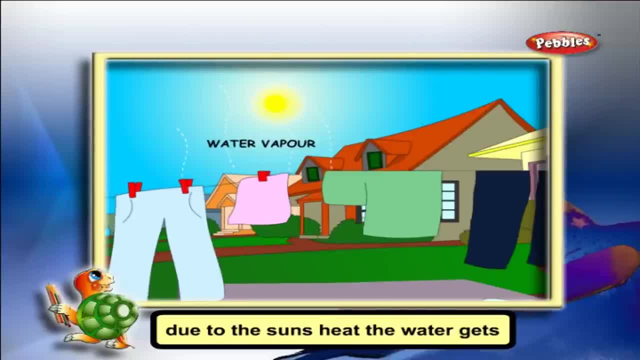 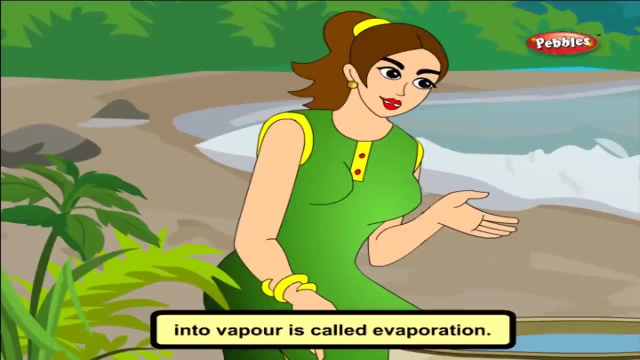 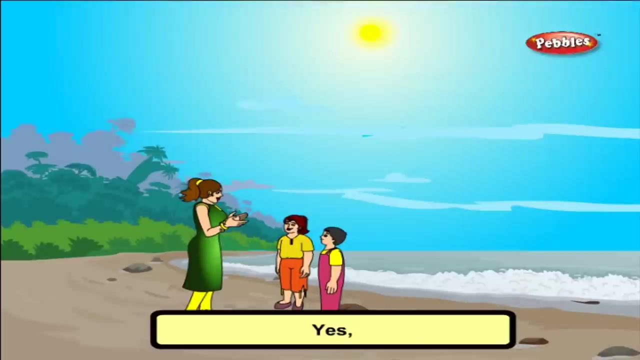 Where does this water go? due to the sun's heat, the water gets converted into water vapor and mixes up with air. this process of conversion of water into vapor is called evaporation. Are we breathing this air which has dust? Yes, but Polluted air is not good for our health. We must breathe in fresh and clean air. 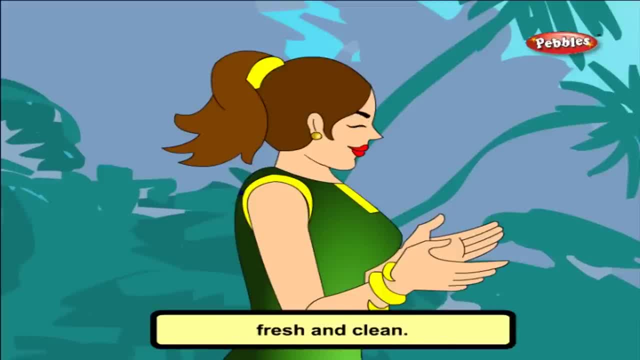 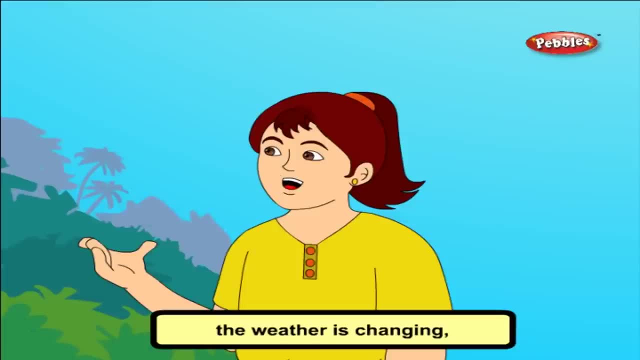 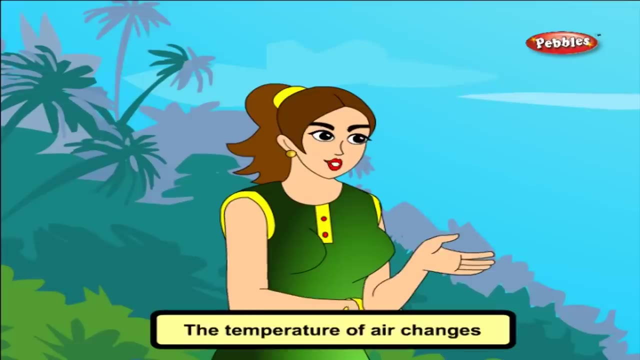 Plants helps keep the air fresh and clean. we should grow green plants. Auntie, the weather is changing. It's It's becoming very cold. now, What is weather? the temperature of air changes from day to day and from time to time This is called weather. Sometimes it is very hot. 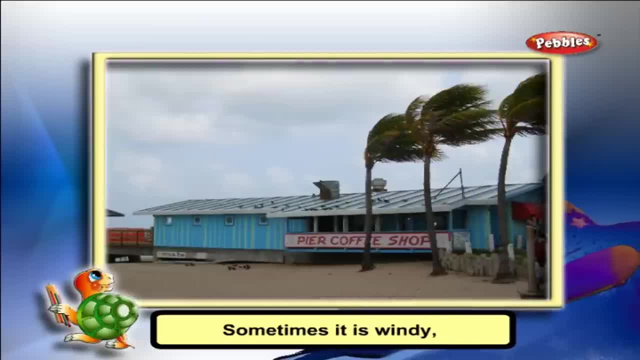 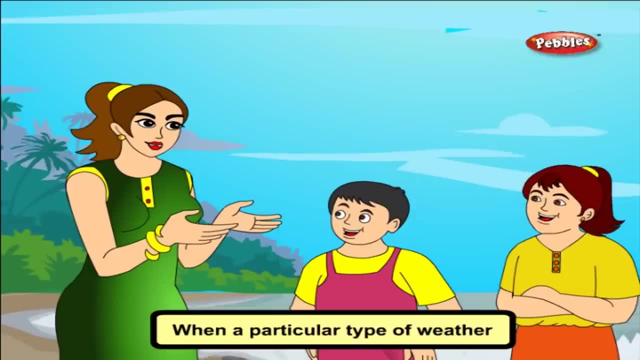 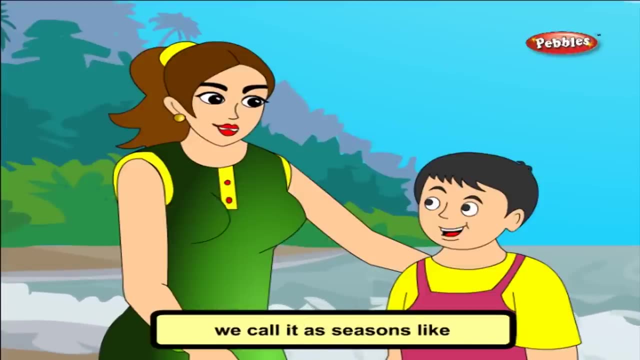 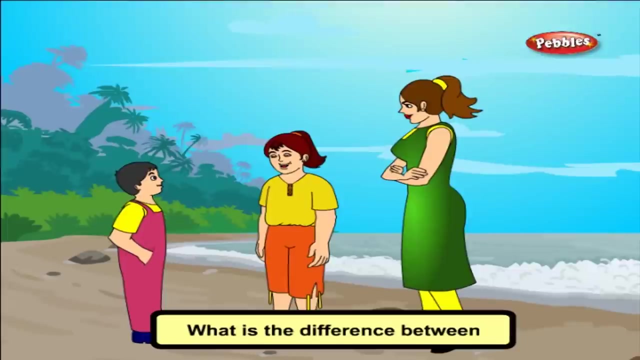 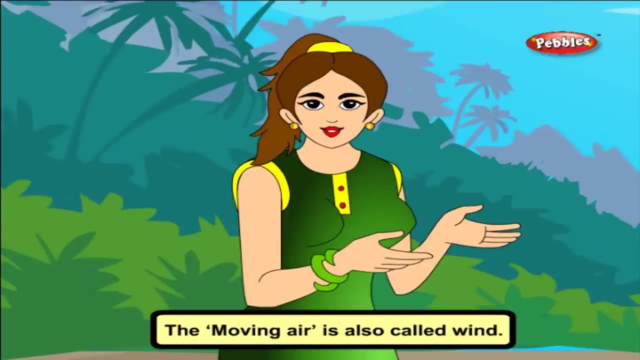 Sometimes it is very cold, Sometimes it is windy. when heavy winds blow, when a particular type of weather prevails For longer days, We call it as seasons like summer, rainy season and winter. What is the difference between wind and breeze? The moving air is also called wind. 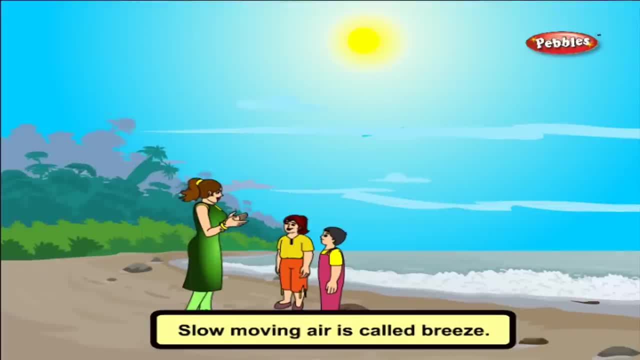 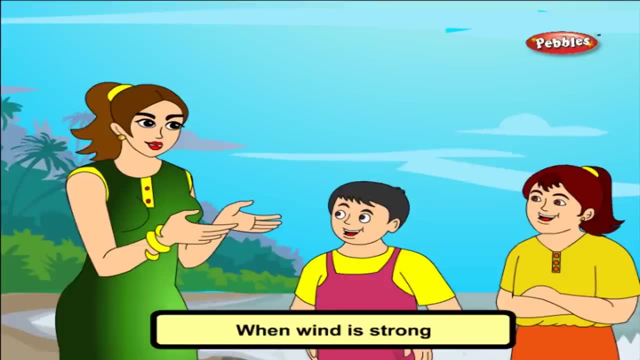 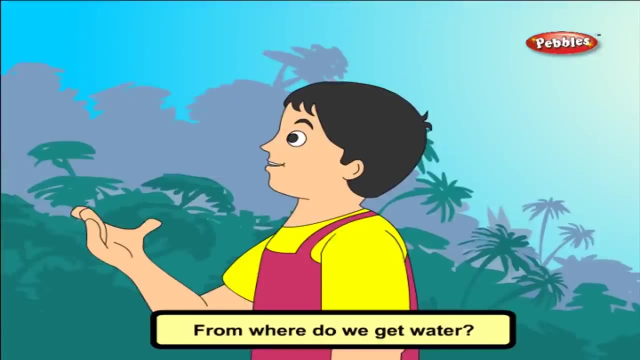 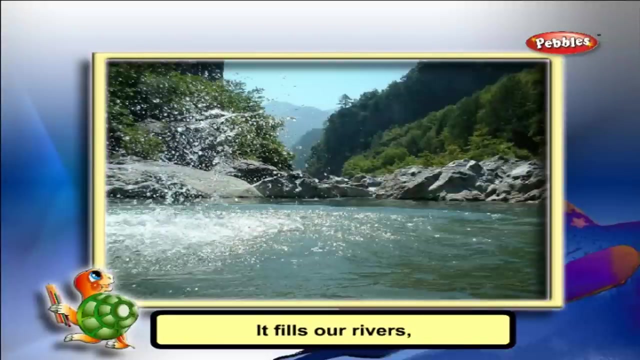 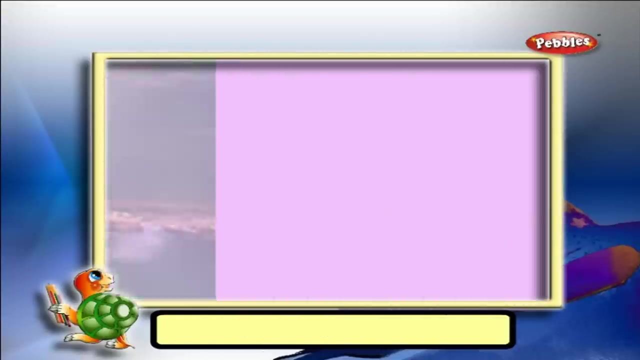 Slow moving air is called breeze. It is gentle and blows softly. When wind is strong and blows very fast, It is called a storm. From where do we get water? We get water from rain. It fills our rivers, lakes, ponds and streams, But I have seen the rivers and lakes are dirty. 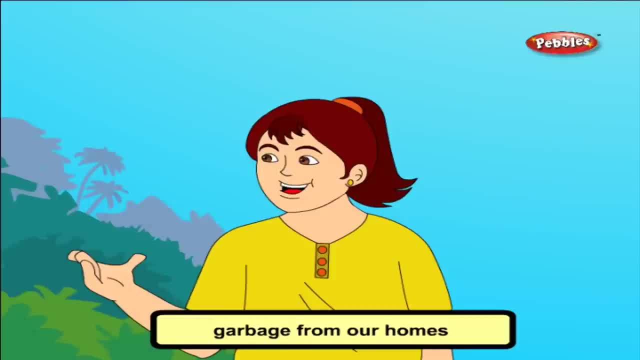 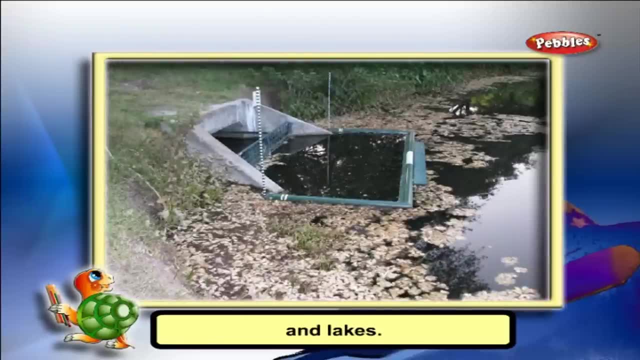 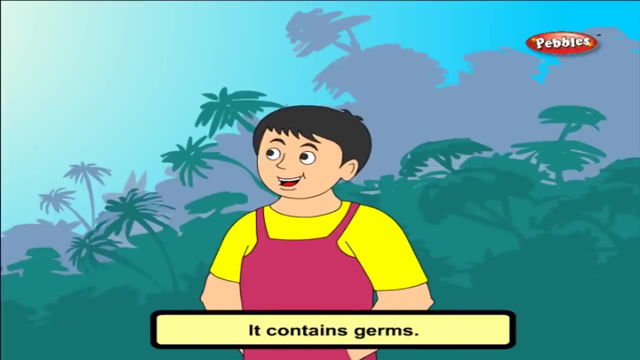 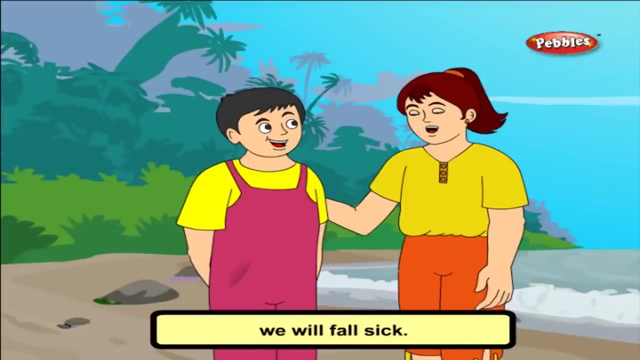 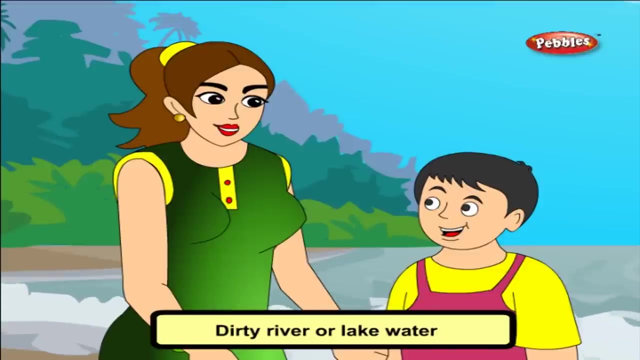 Garbage from our homes and factories is thrown into rivers and lakes So the water becomes dirty. It contains germs. if we drink water containing germs We will fall sick. But how do I get clean water in my house? The dirty river or lake water is taken to the water works in our city. 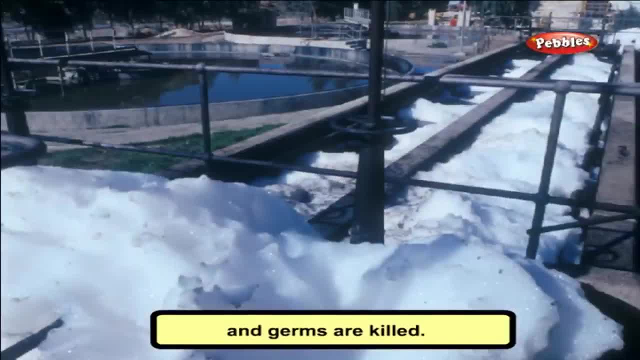 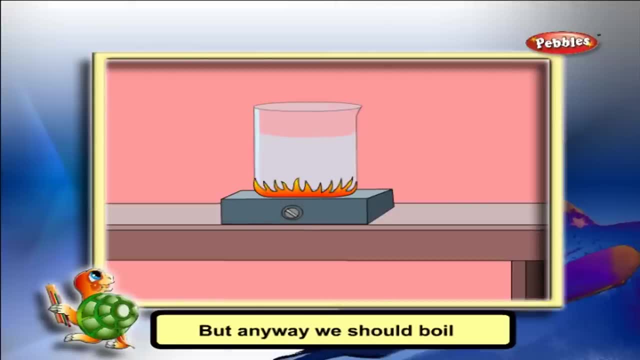 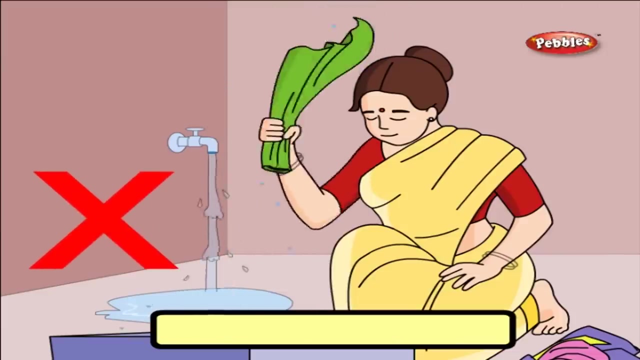 Here the dirt is removed and germs are killed. Then the clean water is supplied to our homes. But anyway, we should boil the water before drinking Boiling water will kill the germs. We should keep water in closed containers- containers- We should not waste water. 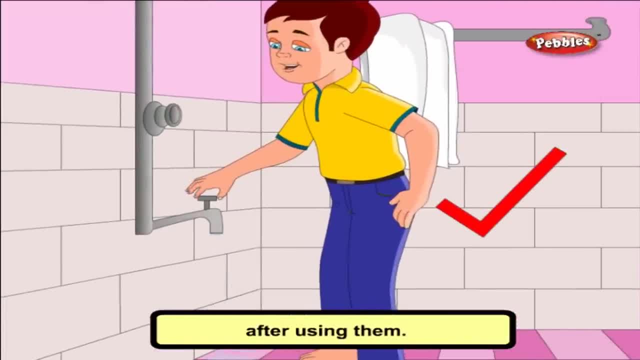 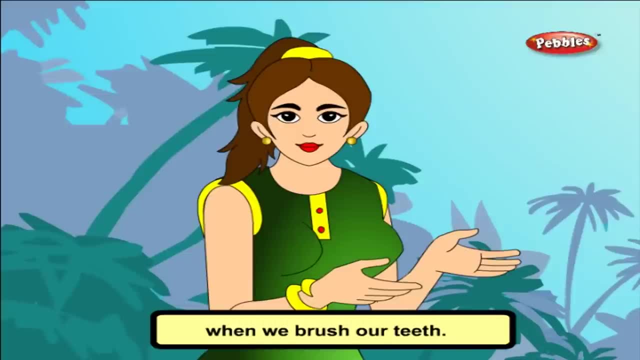 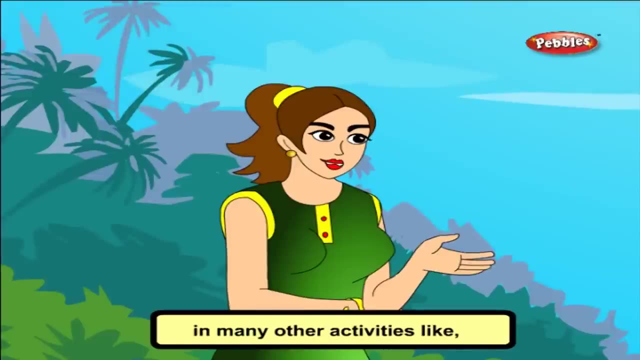 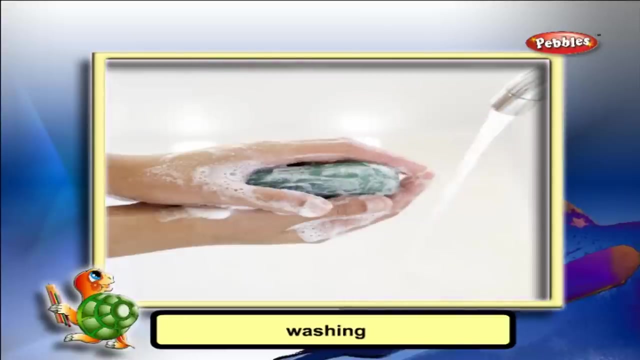 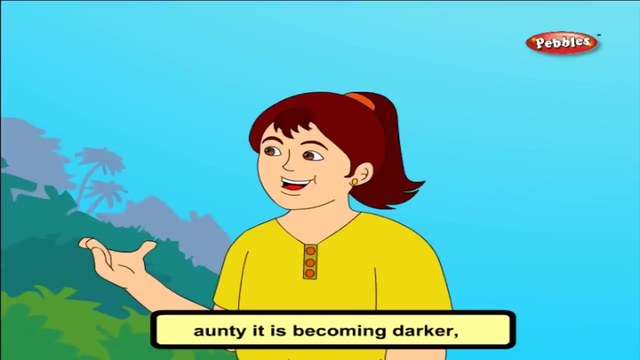 We should turn off the taps after using them. We should not let the tap open when we brush our teeth. Apart from drinking water is also useful in many other activities like cleaning, bathing, washing and watering plants. Yes, let us start from here. 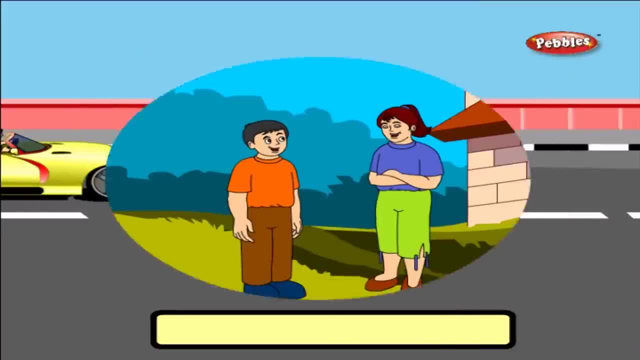 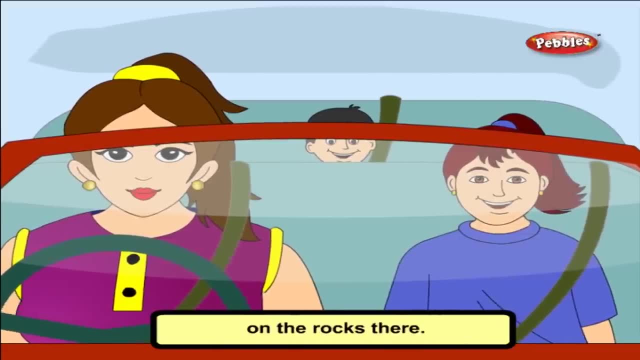 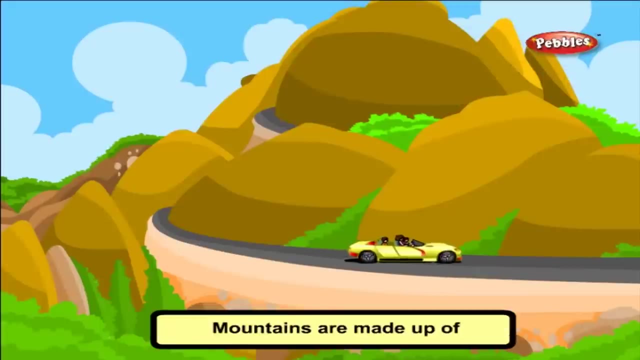 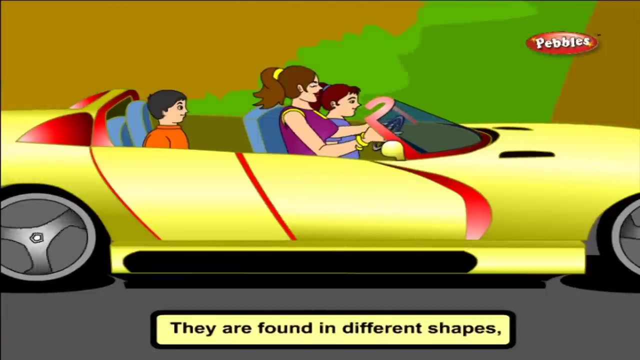 We can see temples and carvings on the rocks there. Half of the earth is made up of rocks. Mountains are made up of hard matter called rocks. There are many kinds of rocks. They are found in different shapes, sizes and colors. 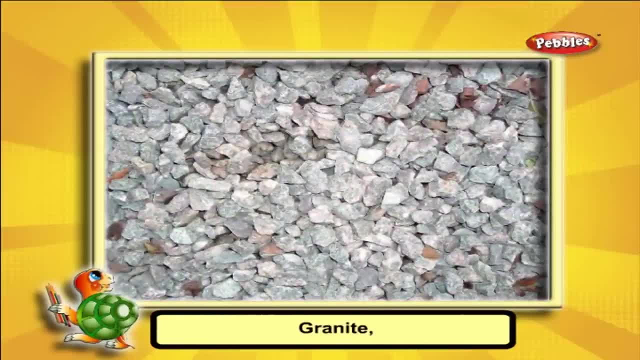 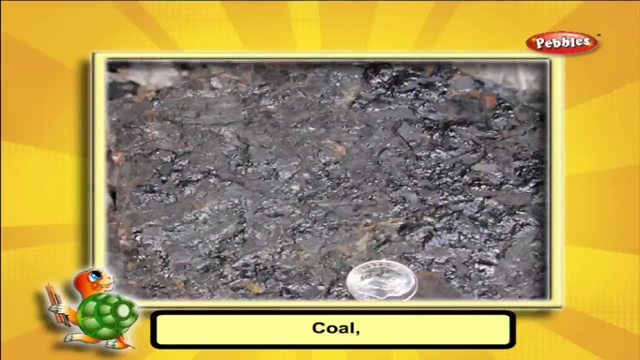 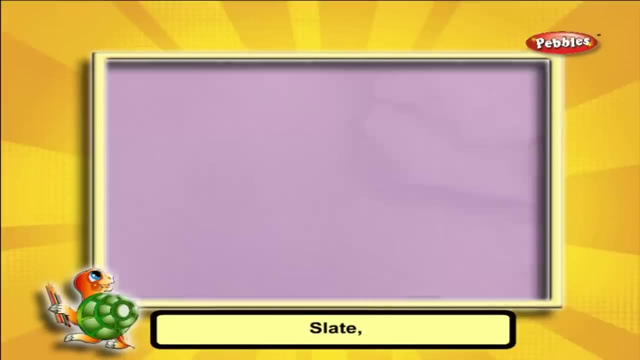 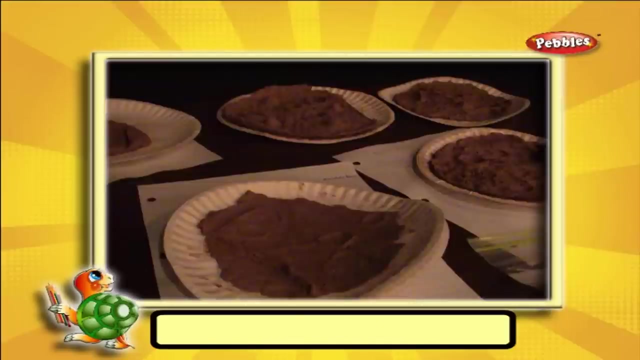 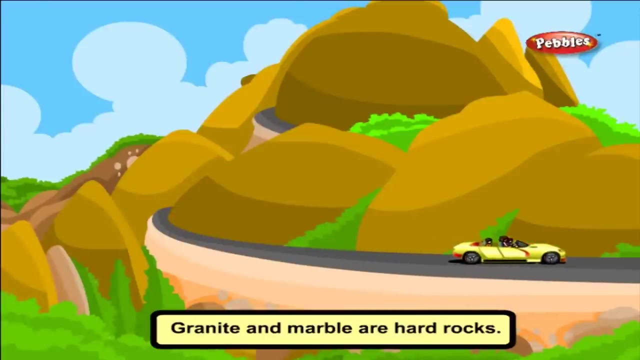 The different kinds of rocks are called rocks. The different kinds of rocks are called rocks. The different kinds of rocks are called rocks. They are granite, marble, sandstone, coal, graphite, slate, limestone, talc and clay. Some rocks are very hard. some are soft in nature. 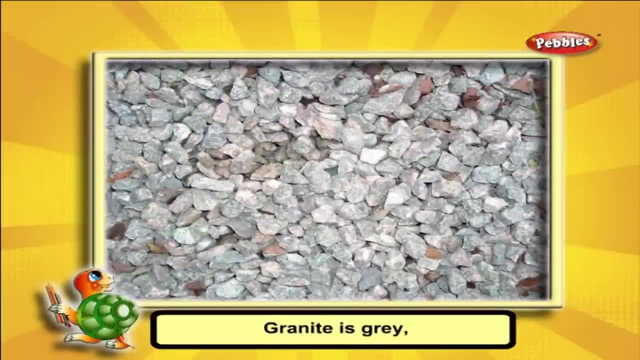 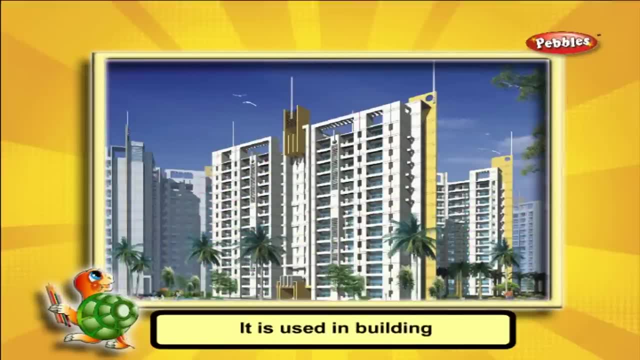 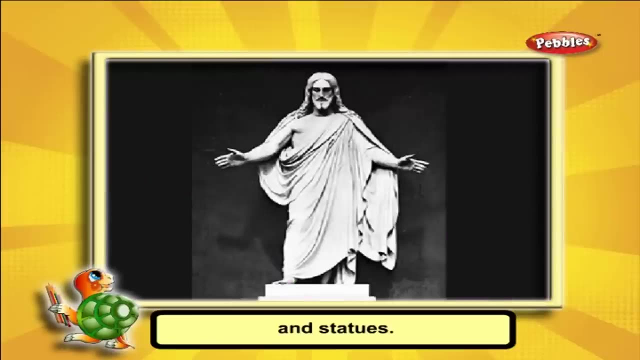 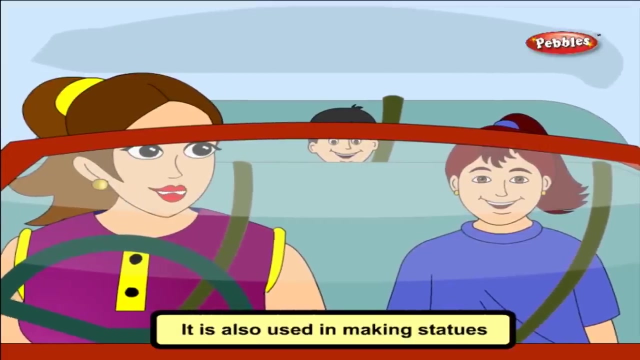 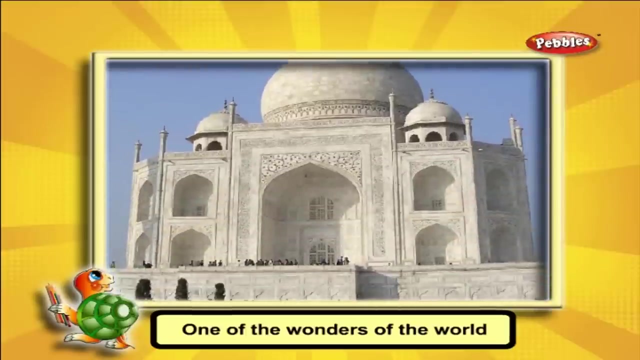 Marble are hard rocks. Granite is grey, black or light red in color. It is used in building houses, roads and statues. Marble is a smooth rock. It is also used in making statues and buildings. One of the wonders of the world is Taj Mahal. 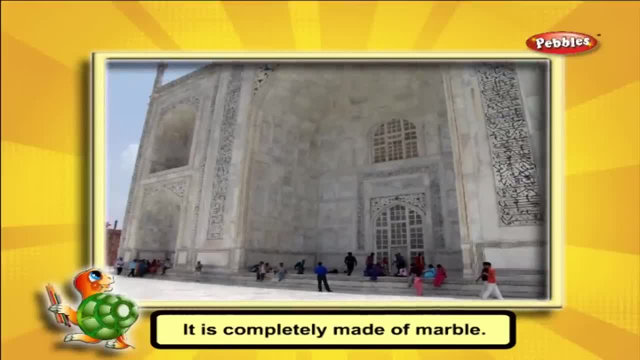 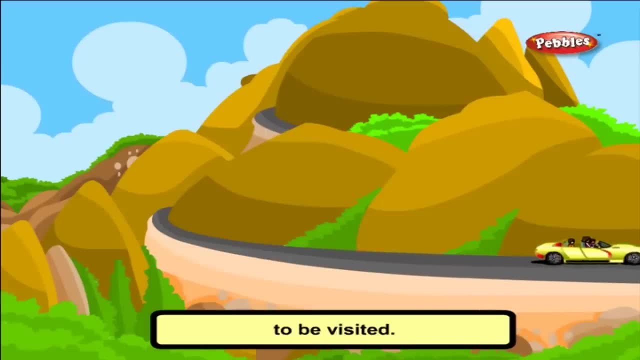 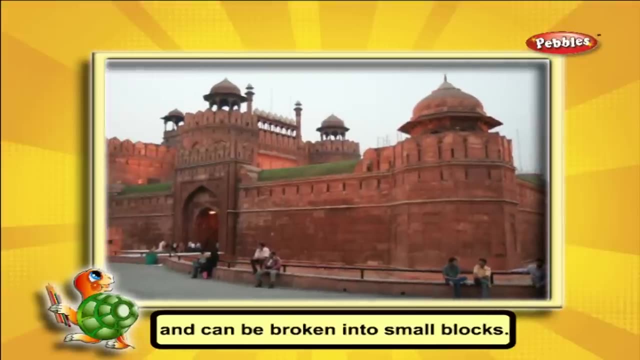 It is situated at Agra. It is completely made of marble. Have you visited Delhi before? There are many important buildings to be visited. Red fort in Delhi is made of sandstone. It is a soft rock and can be broken into small blocks. 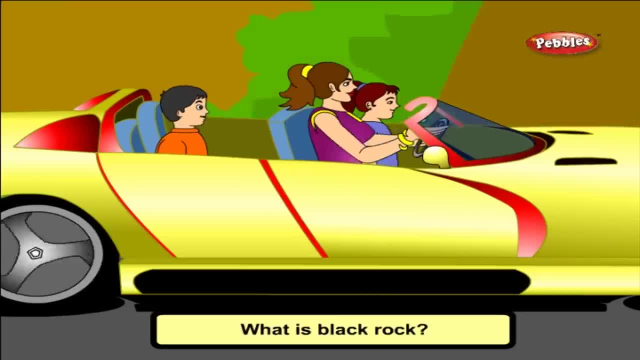 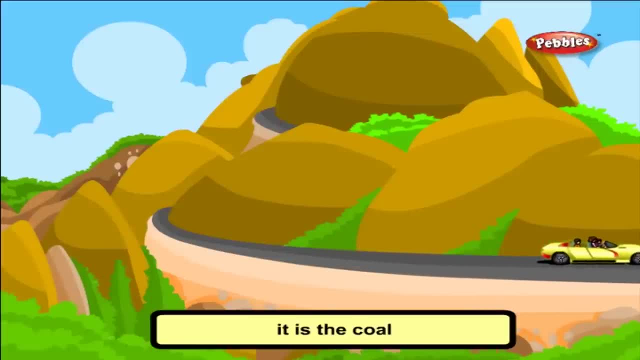 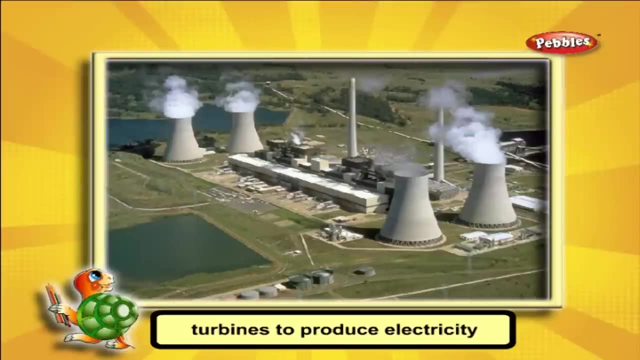 Sandstone is red in color. The red stone is made of sandstone. It is a soft rock and can be broken into small blocks. Sandstone is red in color, Re pearl in red color. It is a black rock. It is a special rock and can be broken into small blocks. 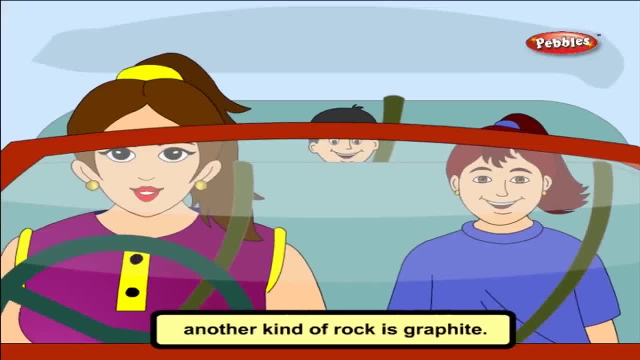 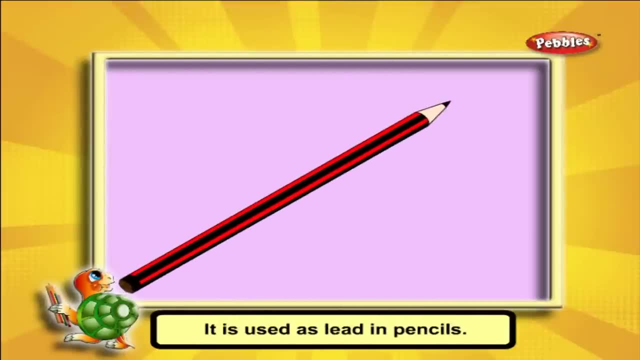 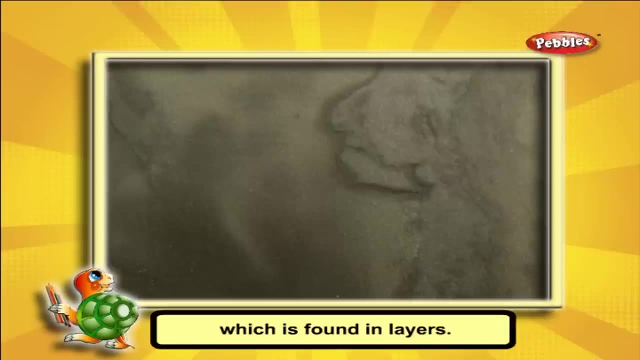 Another kind of rock is graphite. Graphite is black in color. It is used as lead in pencils. This black rock is called nile. It has a small rock in it. Next is the Slate. It is a smooth rock which is found in layers. 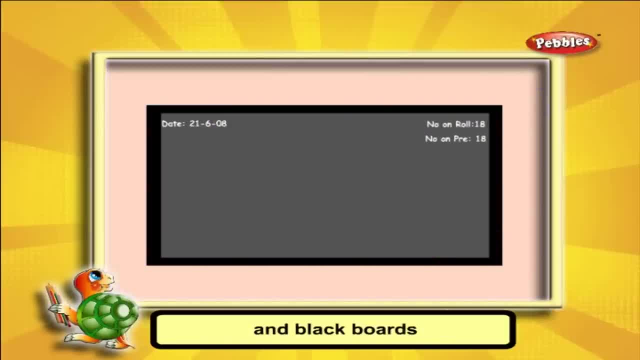 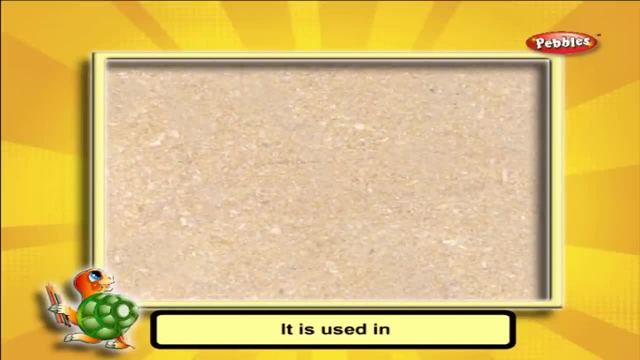 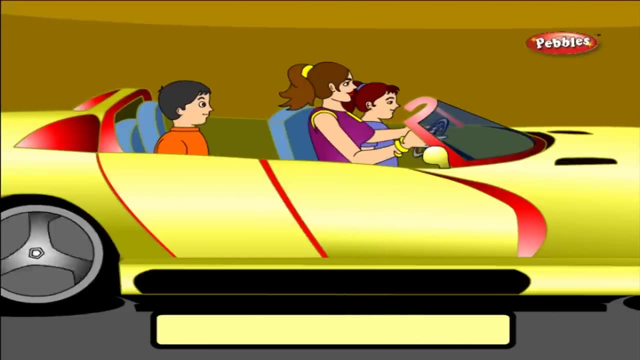 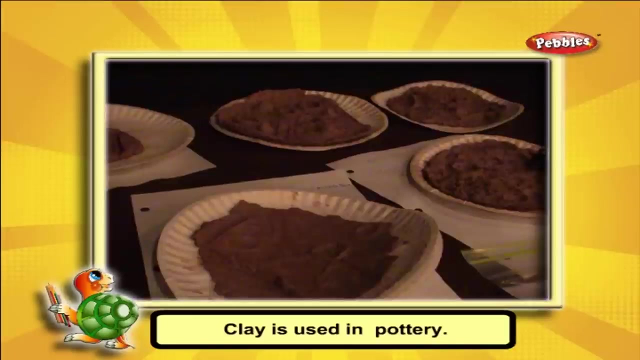 It is used for making slates and black boats and also used for roofs of houses. Limestone is a soft rock. It is used in manufacturing of cement. Yes, we get talcum powder from talc. Black is a soft stone. Clay is used in pottery. 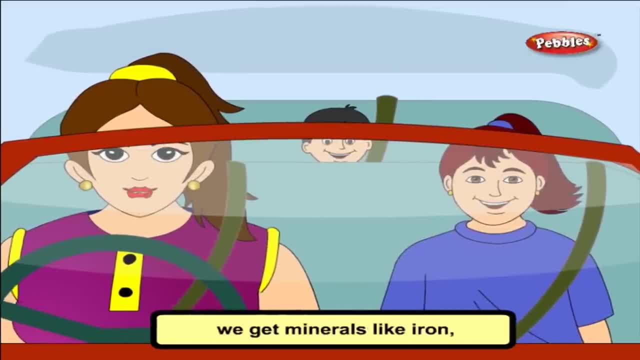 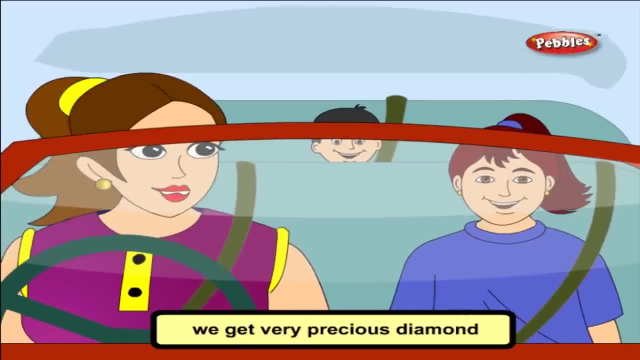 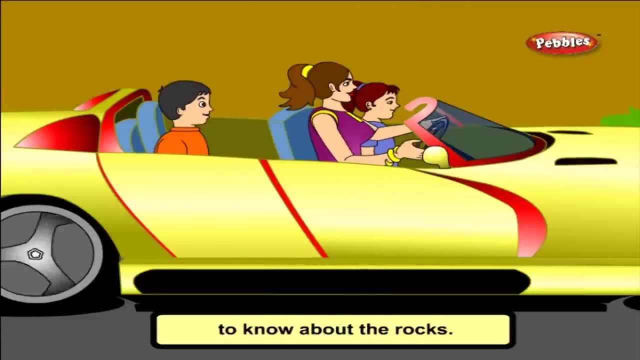 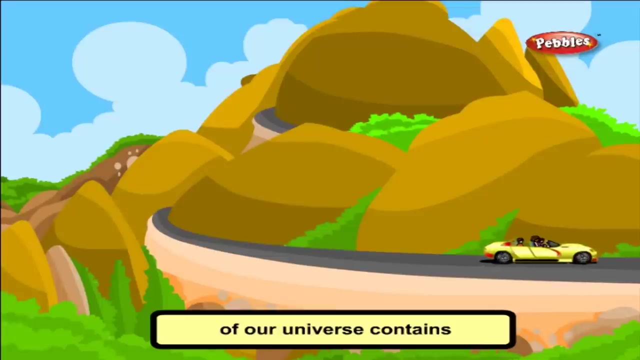 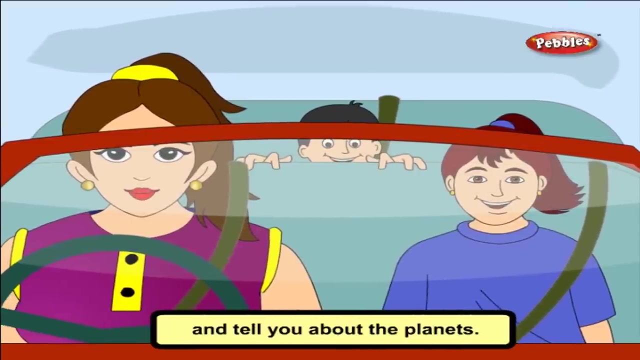 Good question. We get minerals like iron, copper, silver, gold and mica. We get very precious diamond also from the earth rocks, So I guess the planet has a very good potential for getting a good amount of water. Rahul, Tomorrow I will take you to the planetarium and tell you about the planets. 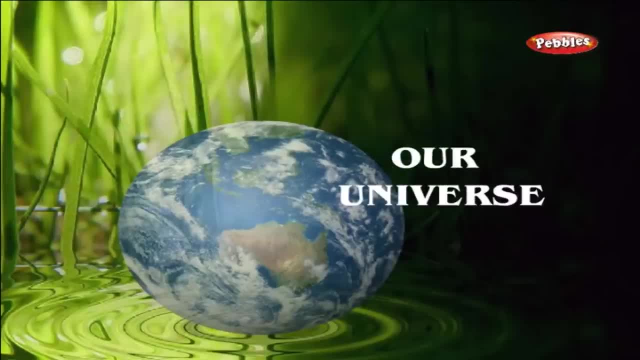 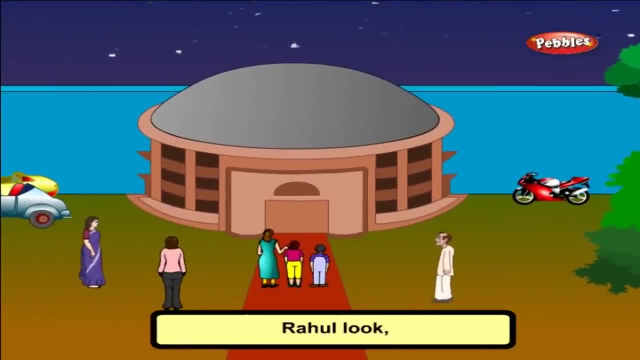 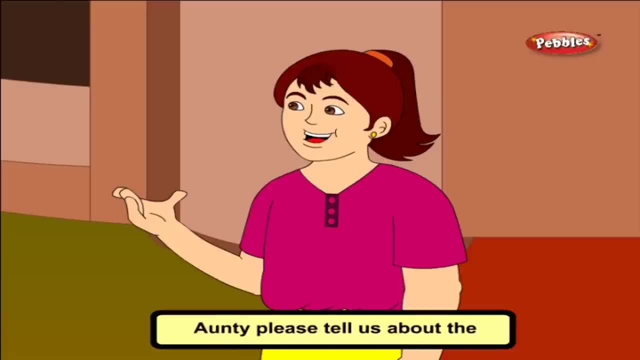 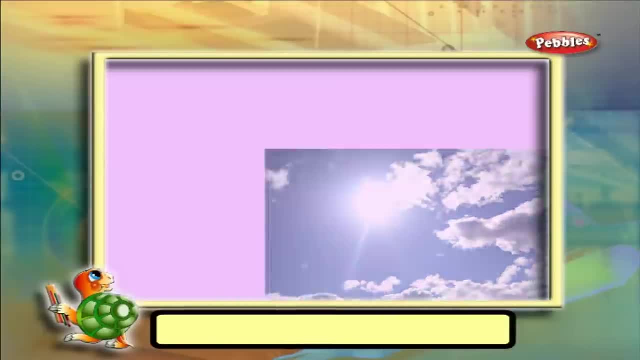 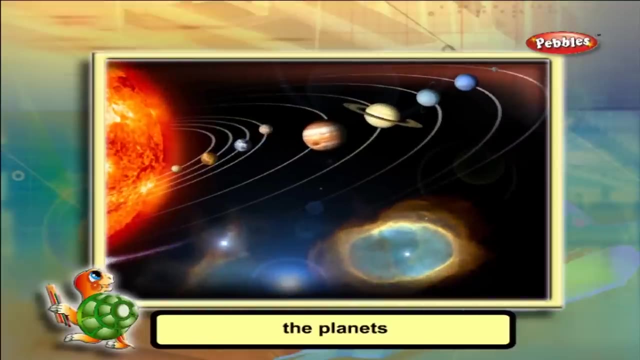 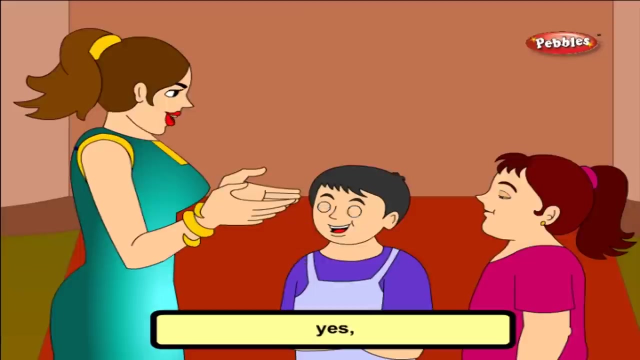 Yes, Yes, I'm going to tell you about the planets. Yes, Our universe consists of the sun, the moon, the earth, the planets and the stars. Yes, the sun is the natural source of light. It is a hot ball of fire. 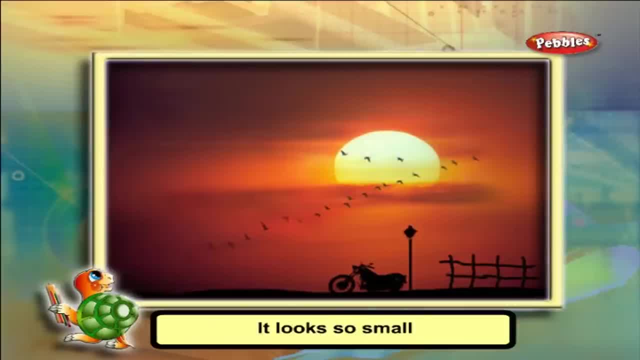 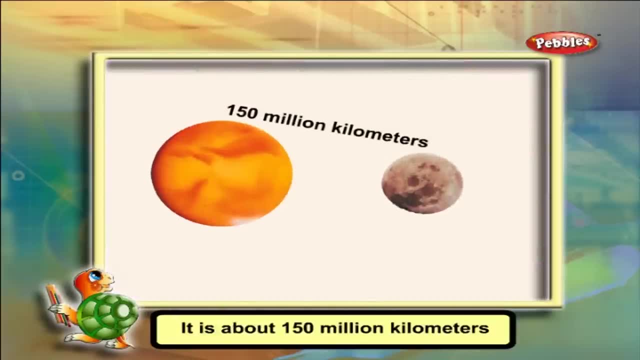 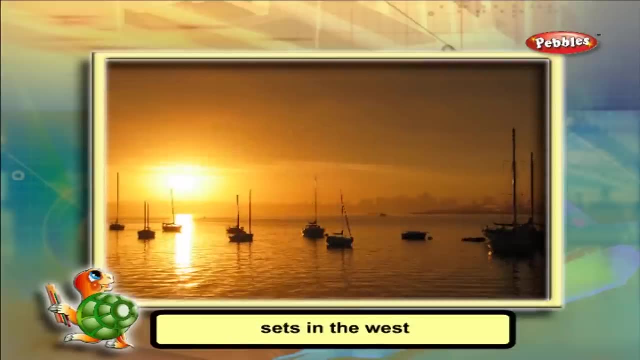 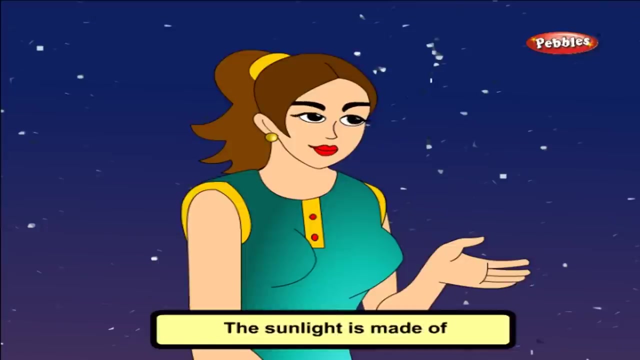 It is made up of hot gases. It looks so small because it is very far away from us. It is about 150 million kilometers away from us. It rises in the east and sets in the west. It gives us light and heat. The sunlight is made of different colors. 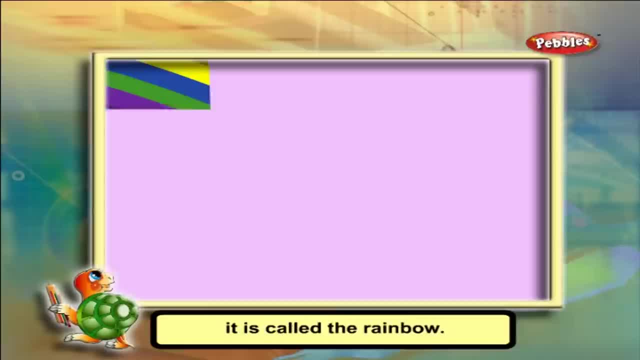 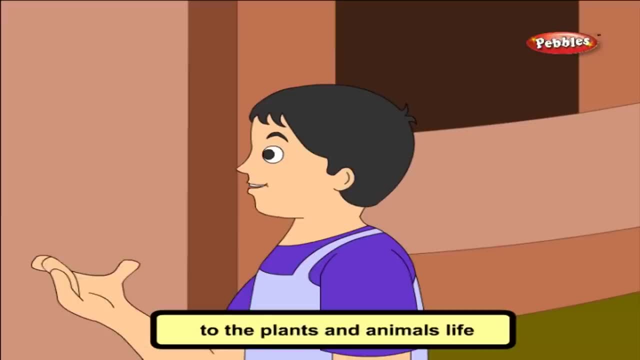 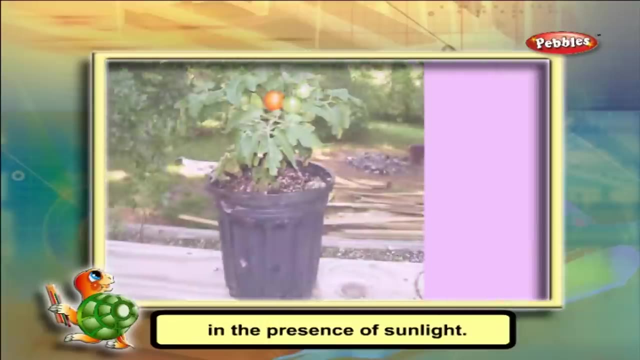 Yes, we manage to progress to a deep palestine. Yes, we do, Yes, we do Yes. it produces the sun. We are programmed to minimize it. Plants prepare their food in the presence of sunlight. Fruits get ripened due to the heat of the sun. 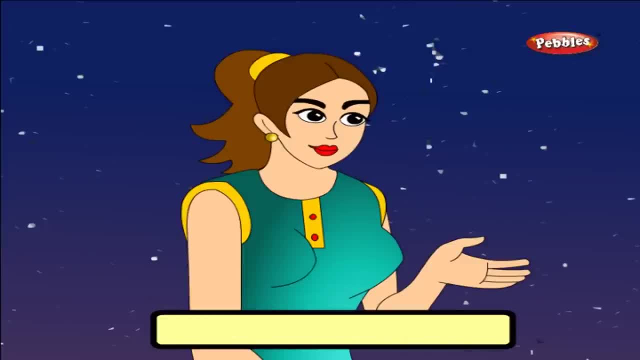 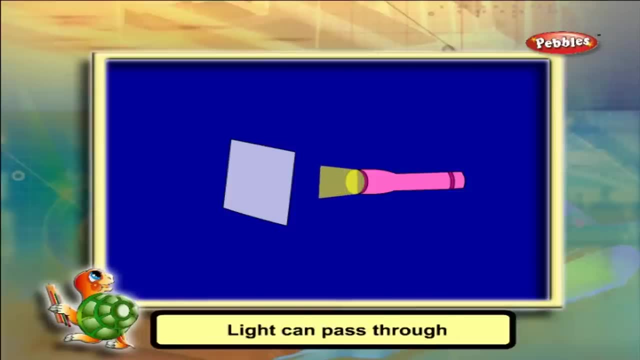 There could be no life on earth without the sun. Yes, there are. Yes, there are. Light can pass through some objects. We can also see through them. We call them transparent objects, like the glass and the water. Light cannot pass through some objects. 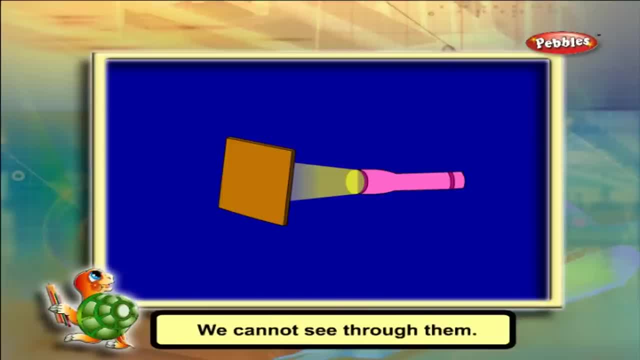 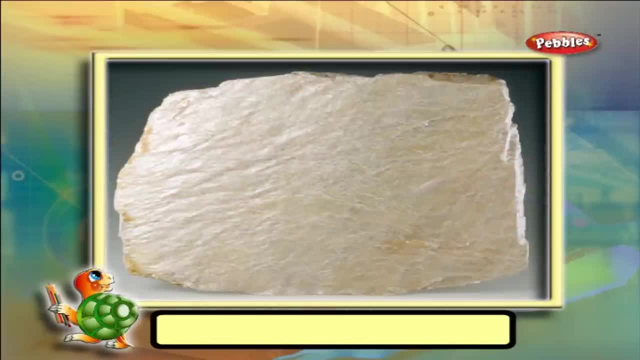 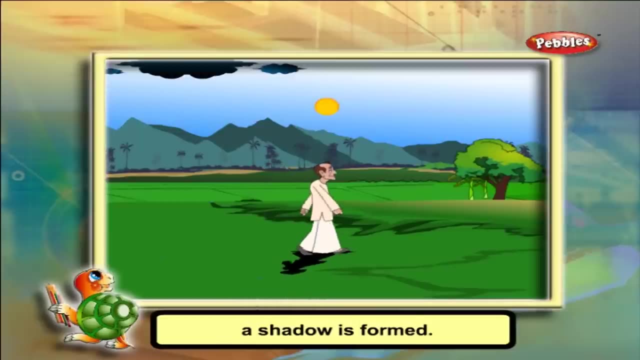 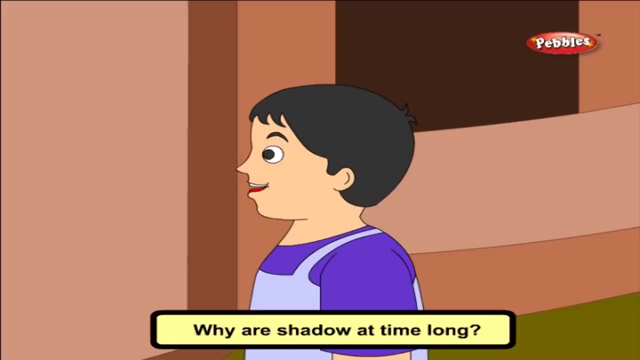 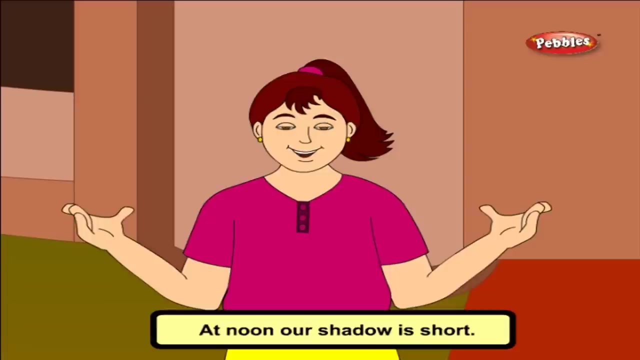 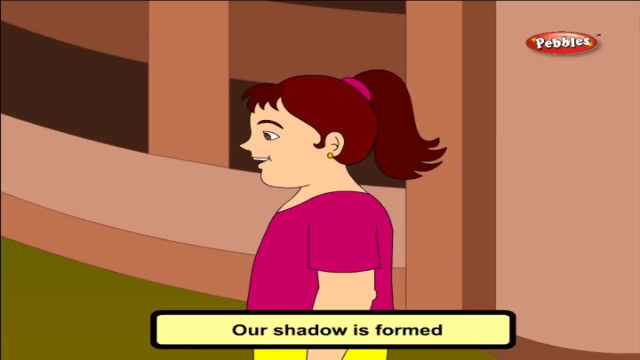 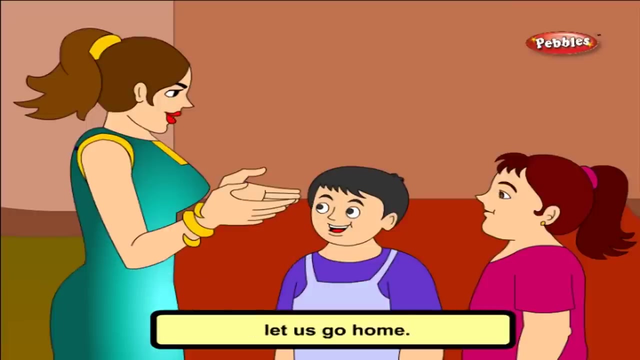 We call them opaque objects. We cannot see through them. Examples are wood and stone. When light cannot pass through an object, a shadow is formed. When we walk in the sunlight, a shadow is formed on the ground. When we walk in the sun, a shadow is formed on the ground. 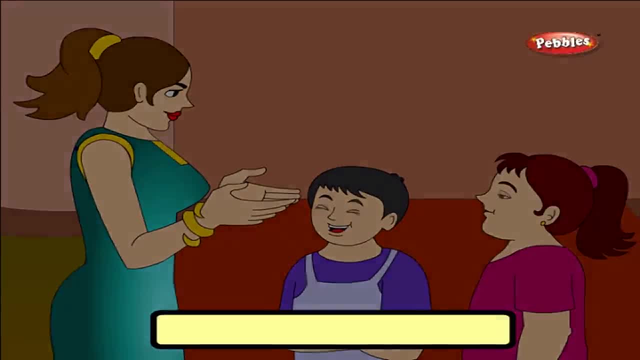 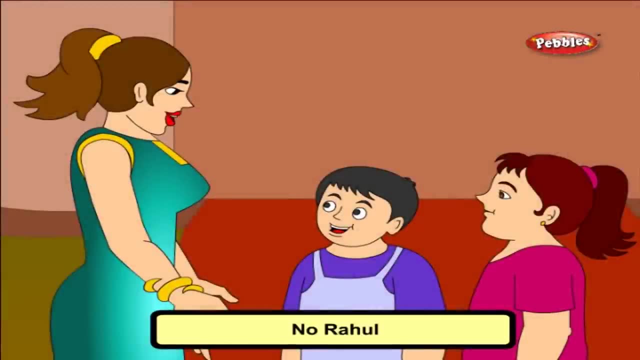 When we walk in the mist, a shadow is formed on the ground. No, Rahul, a home is a very important place. We need a house to protect us from heat, cold, rain, wild animals and even thieves. Go home, Go home. 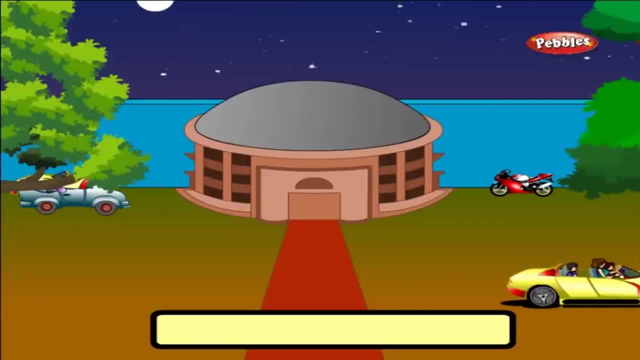 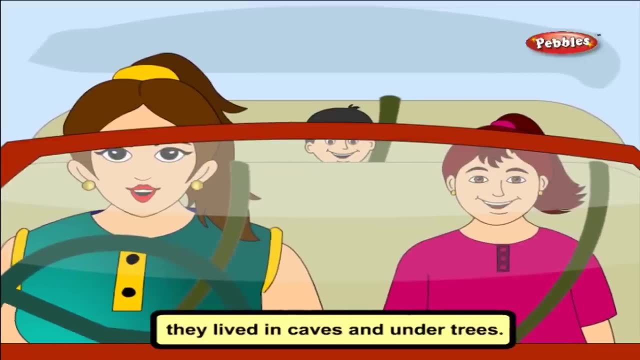 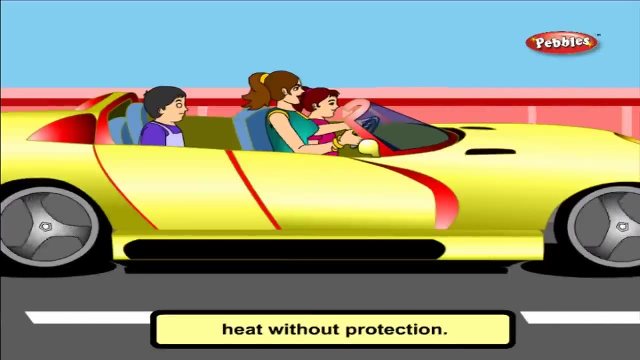 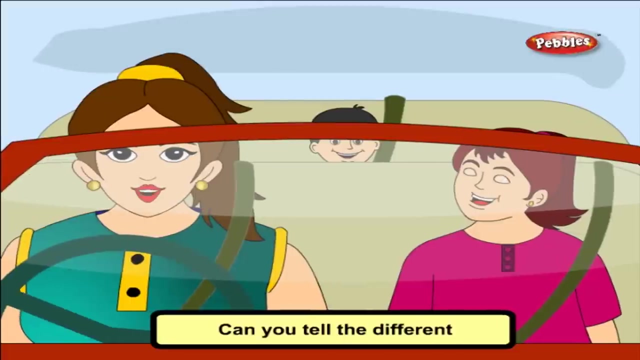 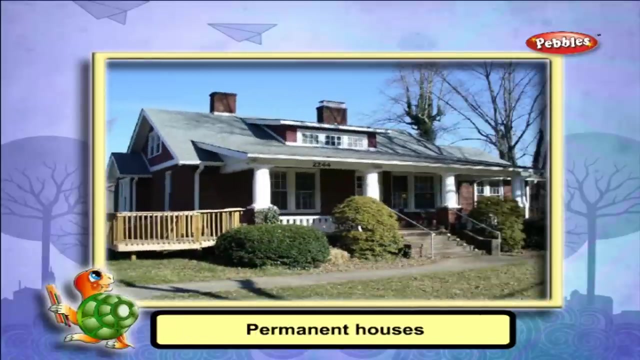 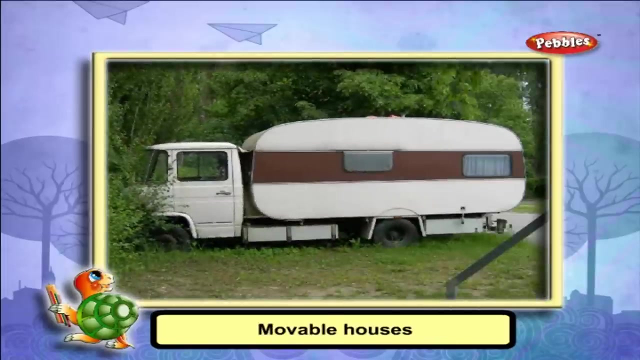 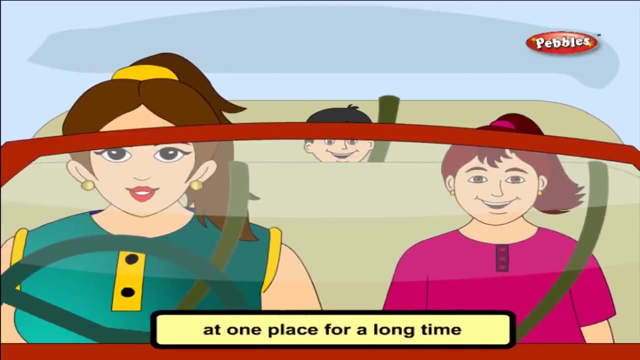 Hello, No, they lived in caves and under trees. They had to live in rain, cold heat without protection, but they realized the importance of shelter. Priya, can you tell the different types of houses? When people choose to live at one place for a long time, they build homes called permanent. 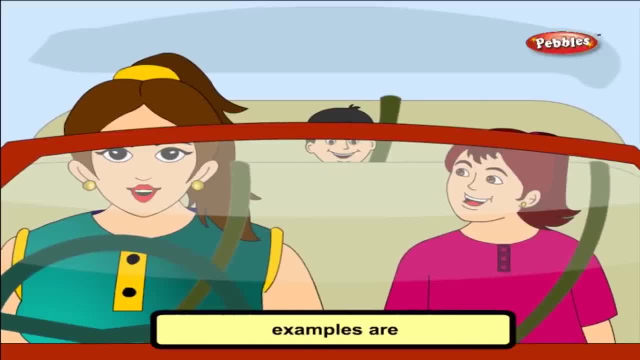 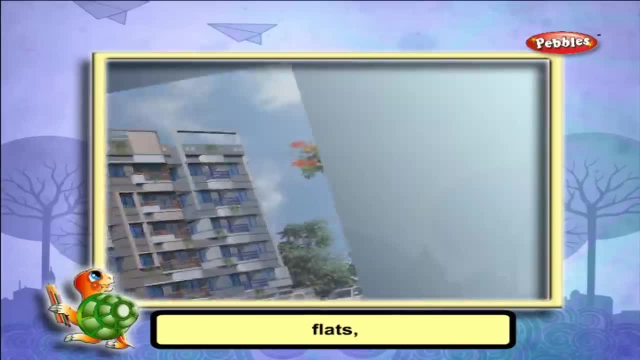 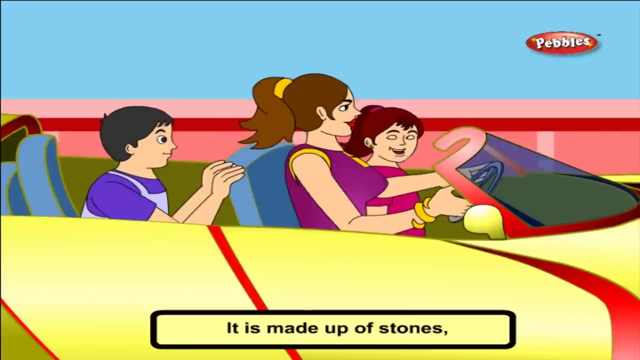 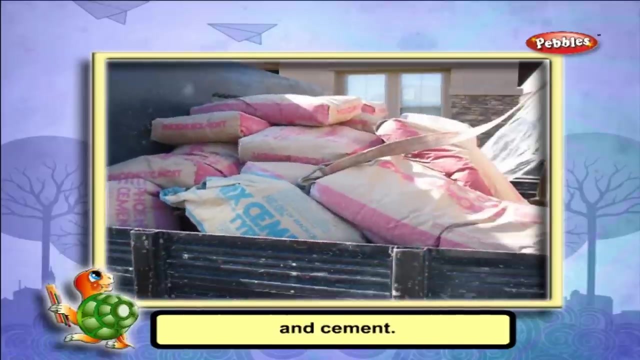 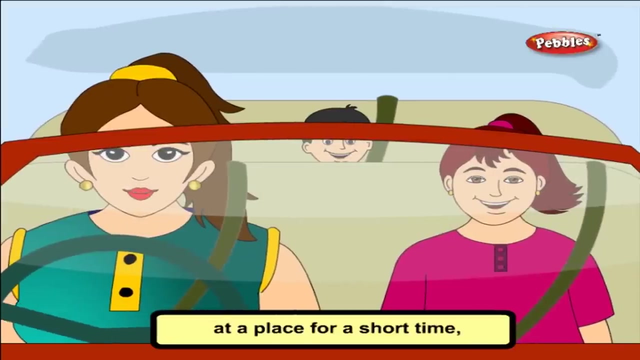 houses Like the houses where we live in today. Examples are multi-storied apartments, flats, bungalow. When people choose to live at a place for a short time, they build homes called permanent houses, Like the houses where we live in today. 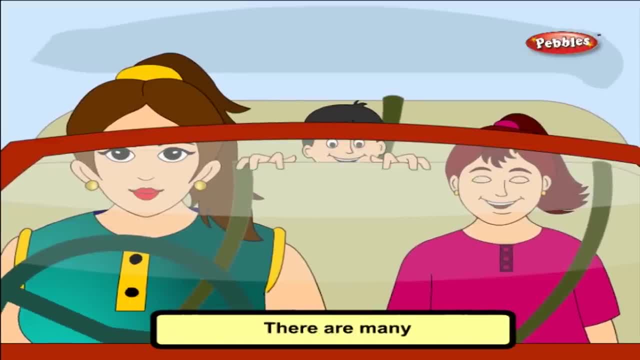 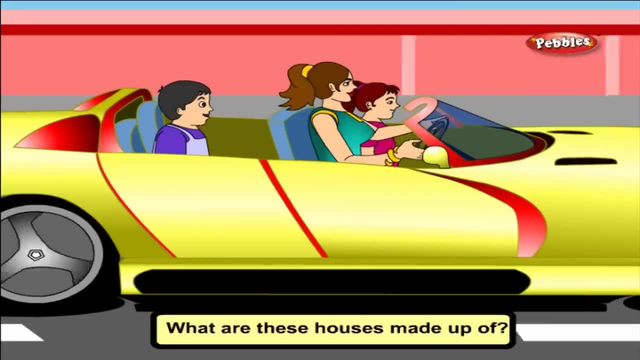 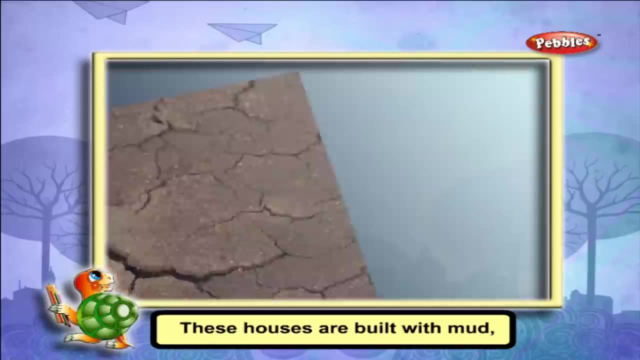 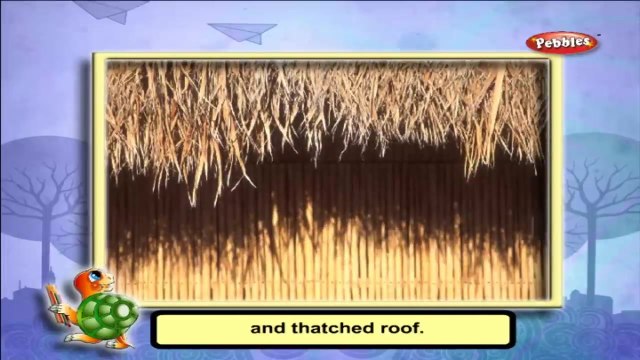 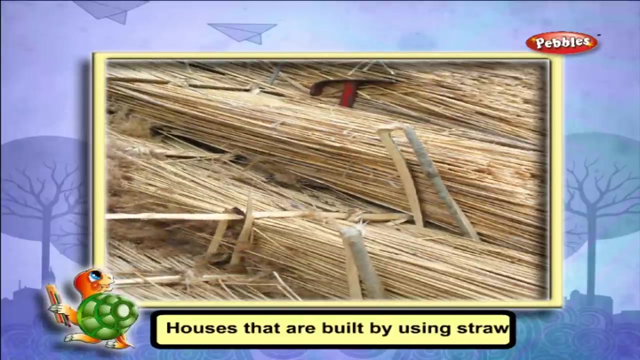 When people choose to live at a place for a short time, they build temporary houses. There are many types of temporary houses, like the huts, and gradually I'm growing a lot of flowers. Now she is about to eat a huge piece of my fruit. 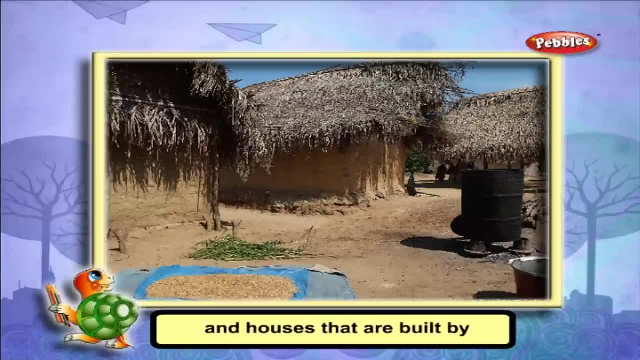 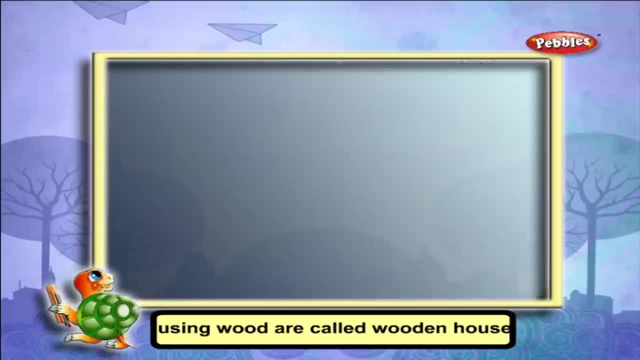 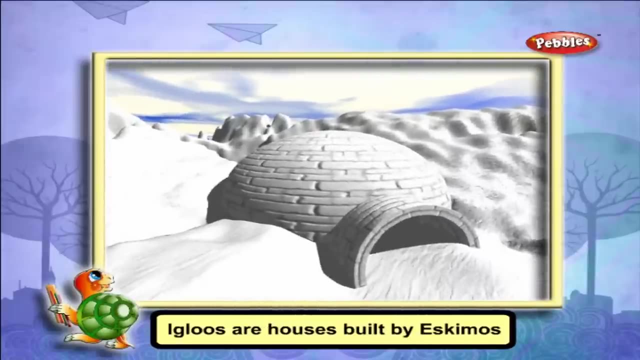 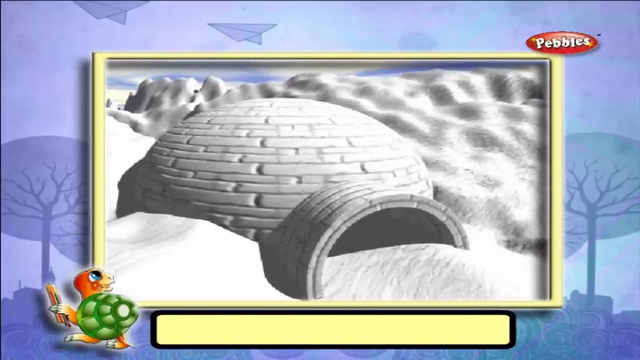 I'm growing that too, And now she is about to eat my little seed plant. I'm growing my little tree. Now she is about to eat my little seed plant. I'm growing that too, And now she is about to eat my little seed plant. 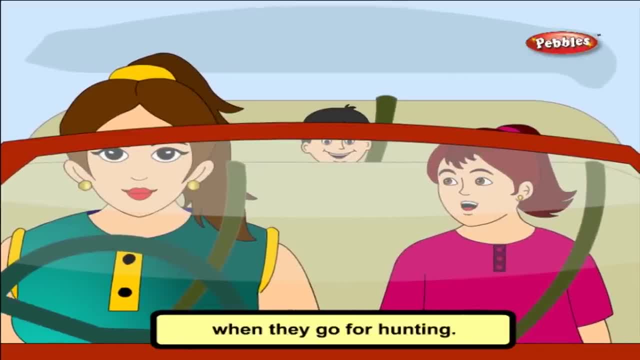 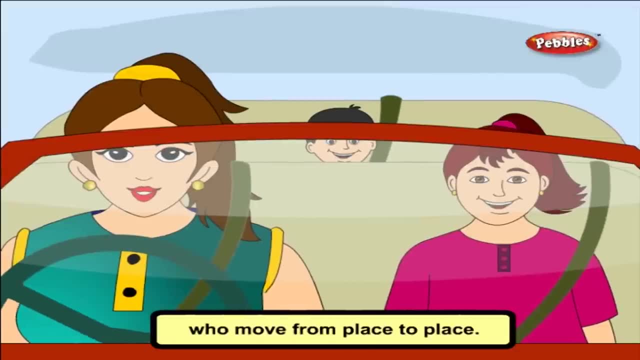 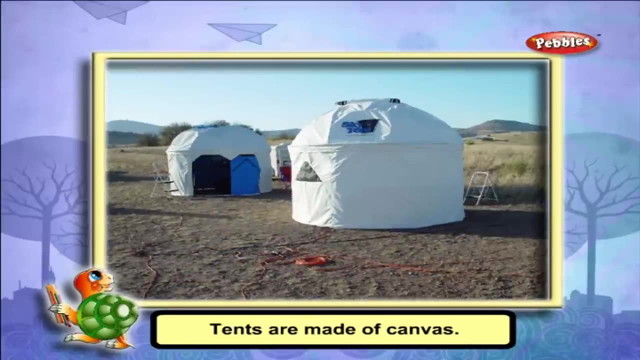 I'm growing that too, And now she is about to eat my little seed plant. The movable houses are used by the people who move from place to place. There are three kinds of movable houses. Tents are made of canvas. It can be easily shifted from one place to another. 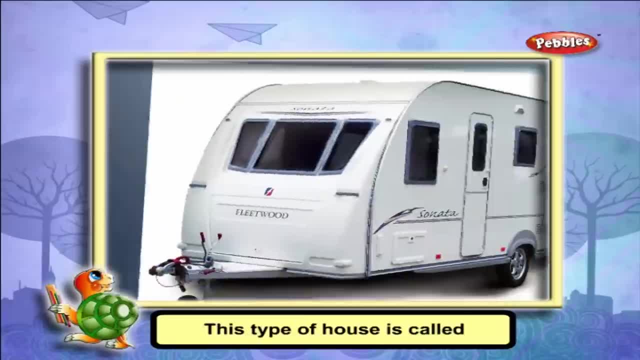 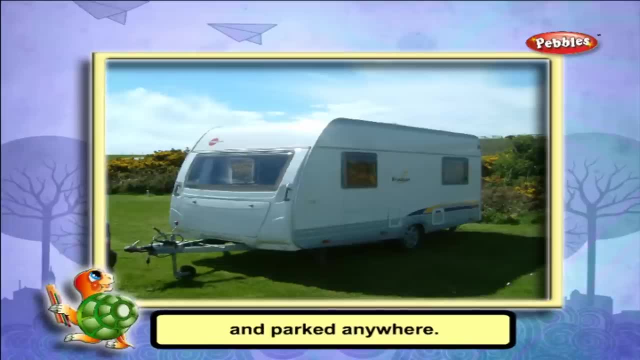 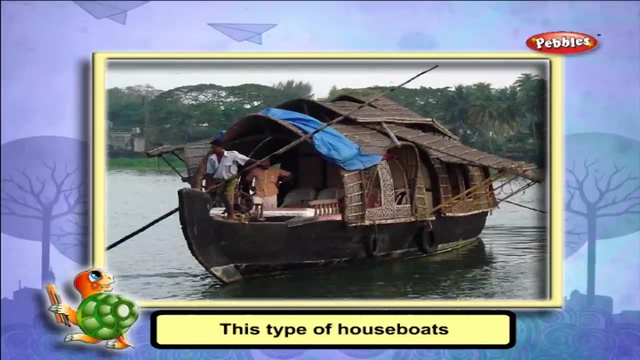 Caravans are built on wheels. This type of house is called a house of wheels. It can be taken to any place and parked anywhere. House boats are made of wood float on water. This type of house boats are found in places like Dal Lake in Kashmir. 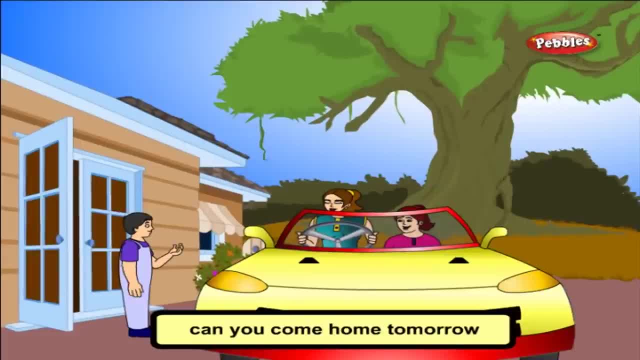 This type of house boats are found in places like Dal Lake in Kashmir. They are very useful to animals in way of trees. There are three types of houses. There are some type of houses: It, Jonah and the other house. also, There are more than three types of houses. 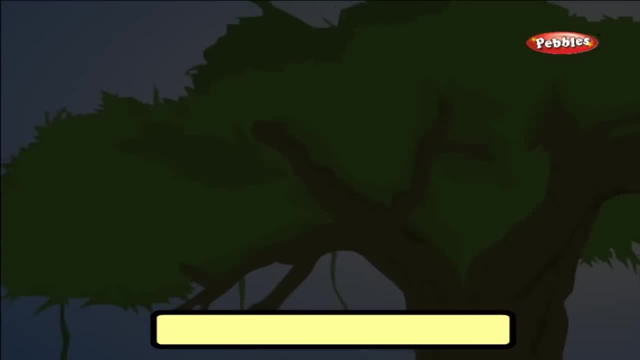 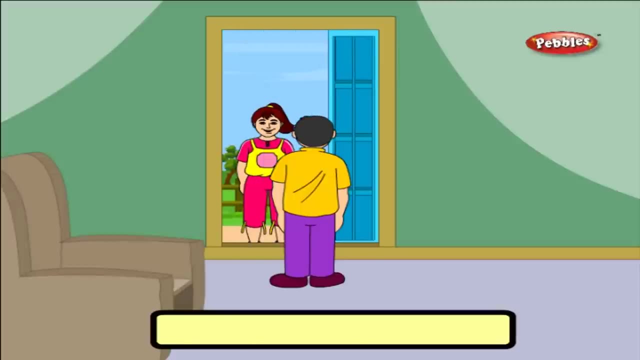 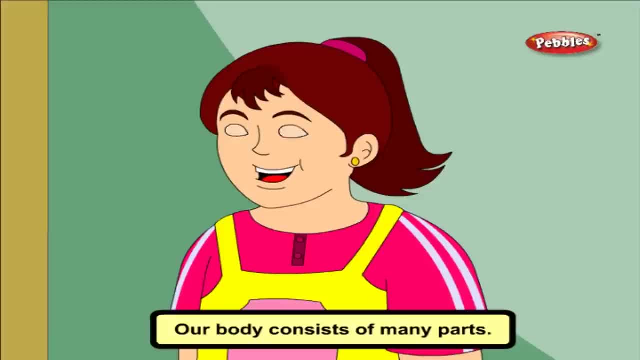 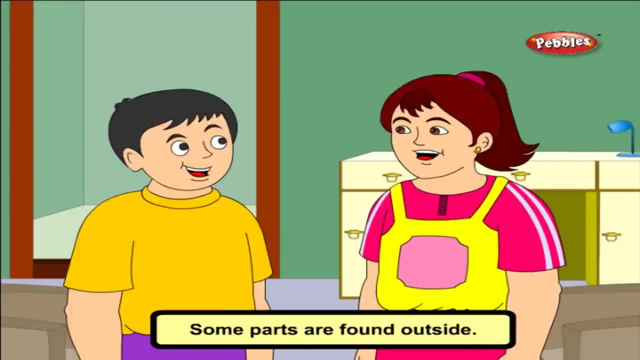 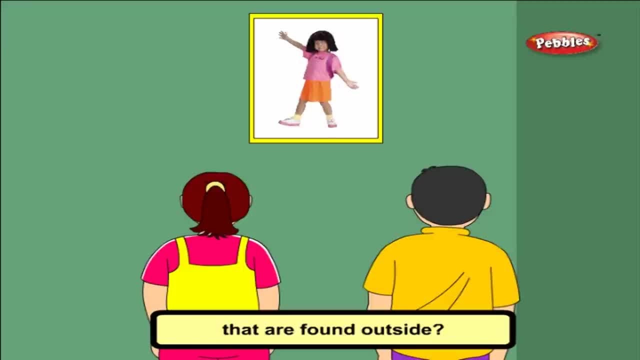 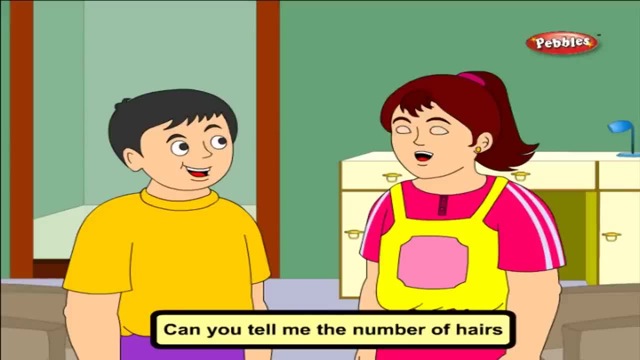 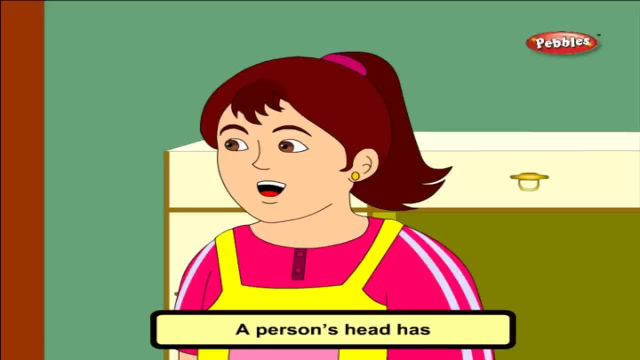 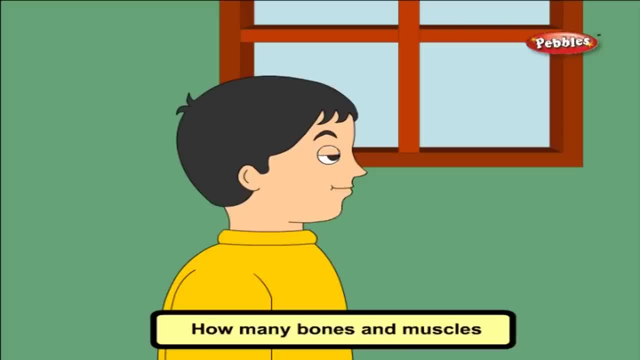 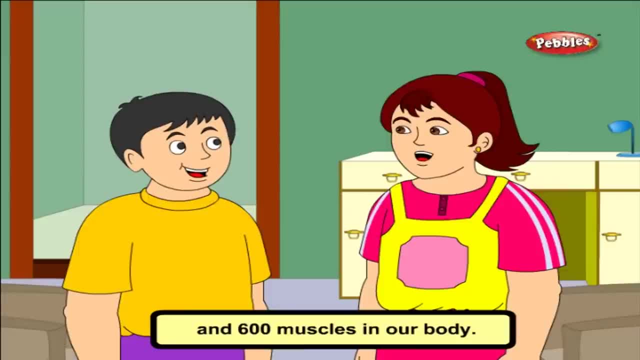 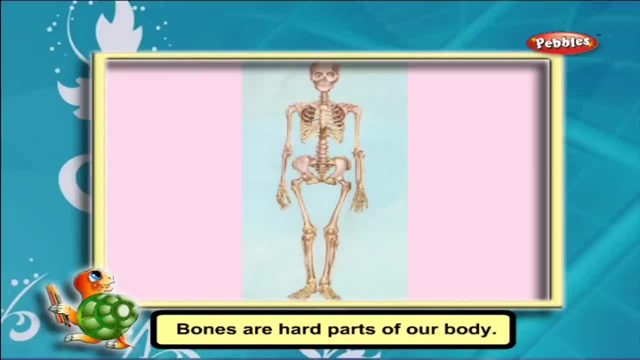 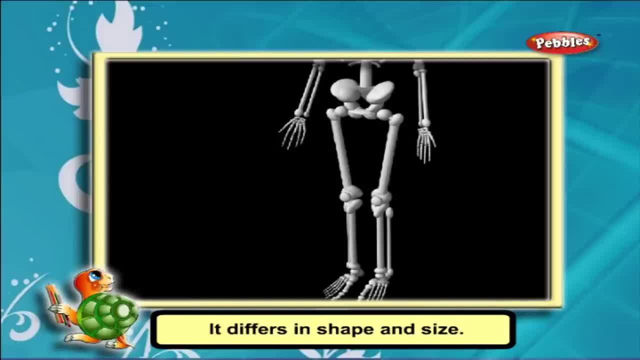 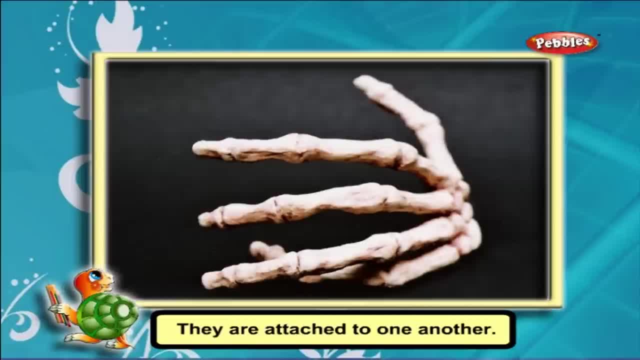 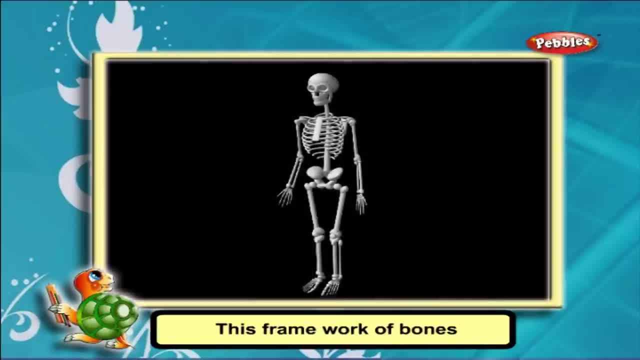 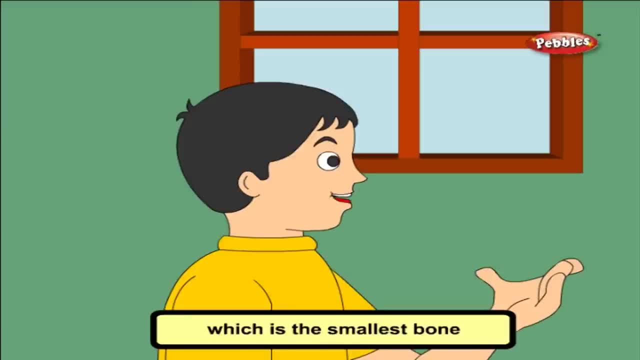 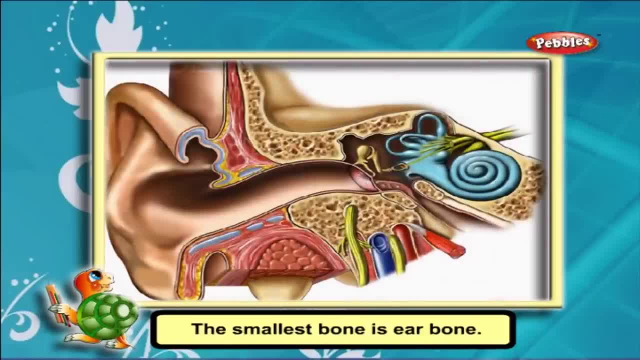 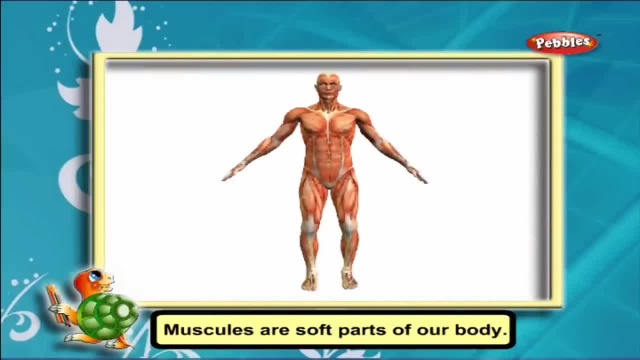 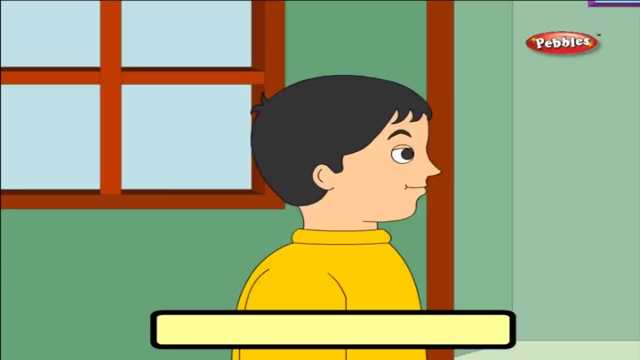 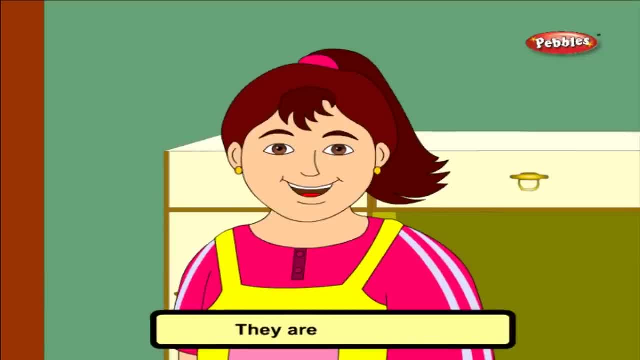 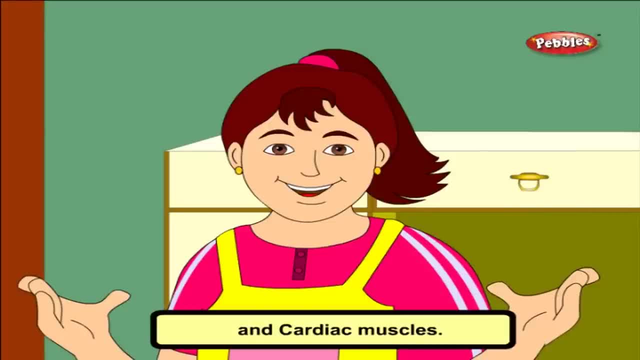 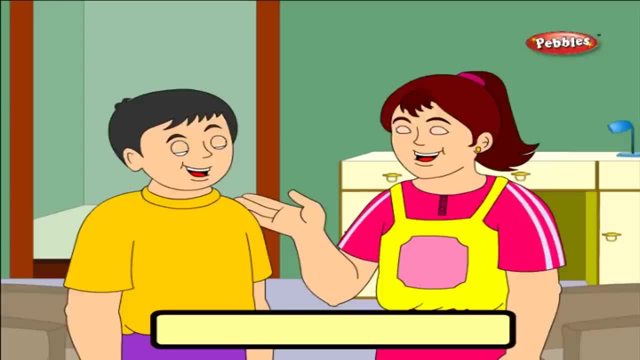 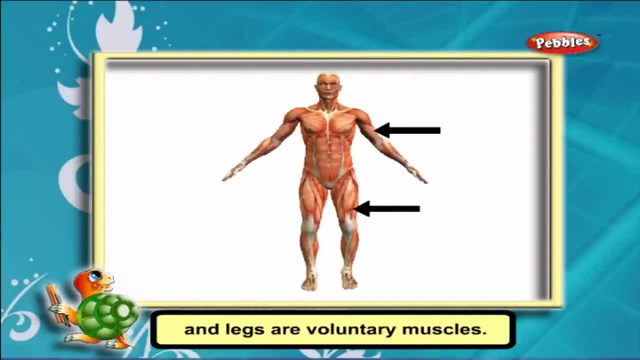 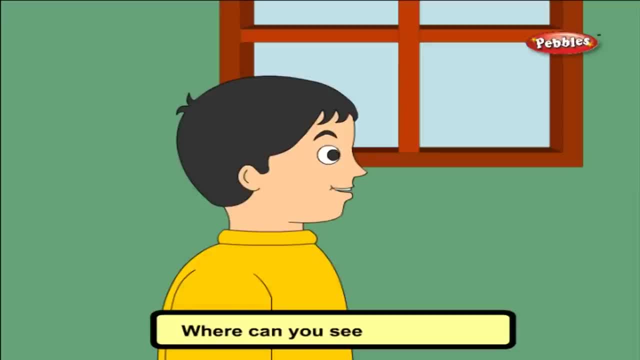 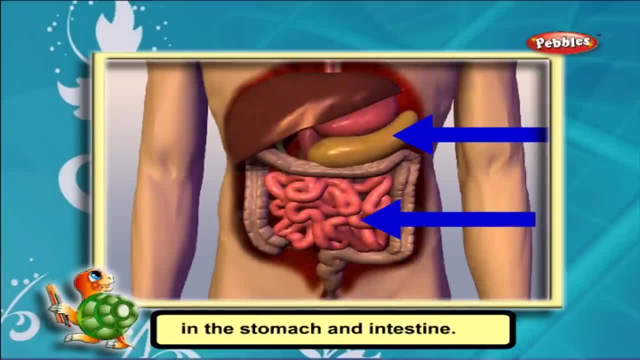 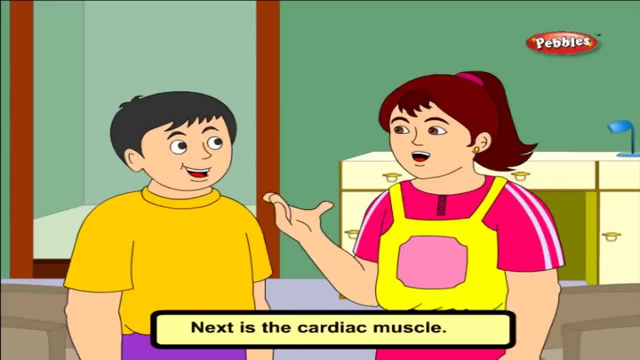 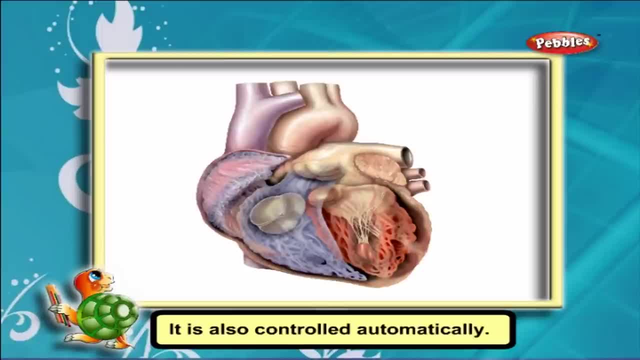 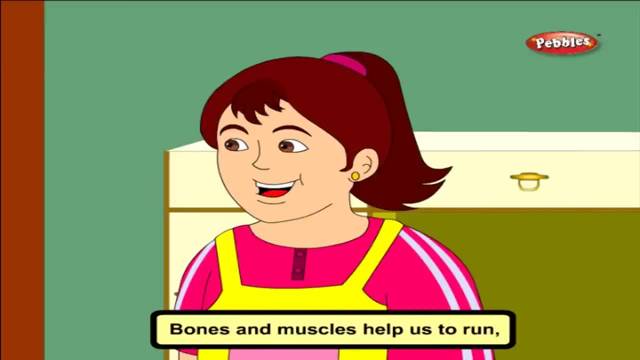 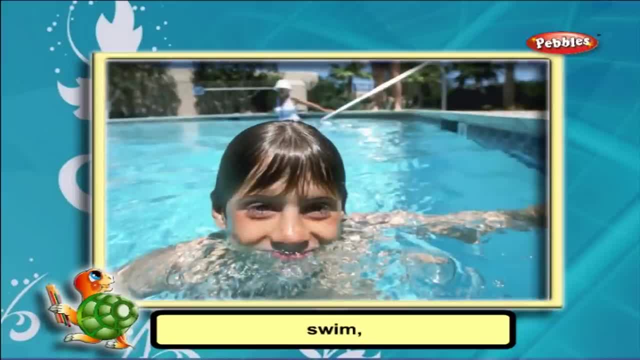 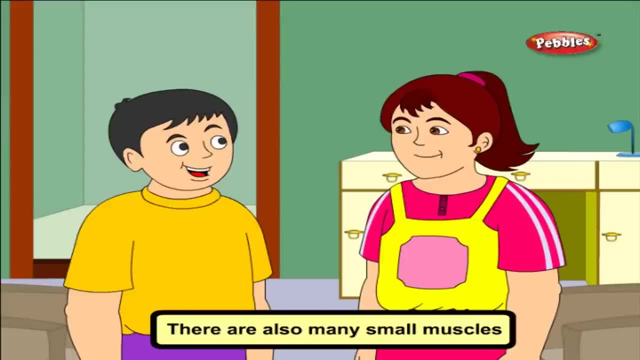 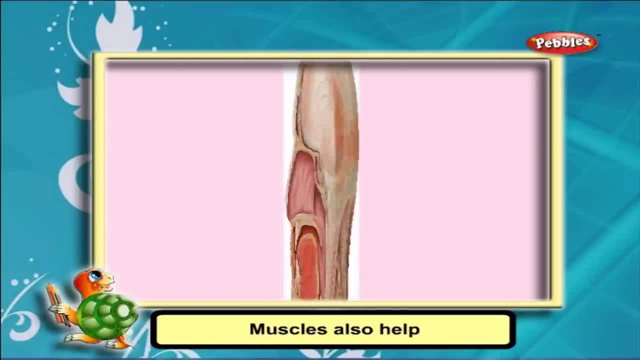 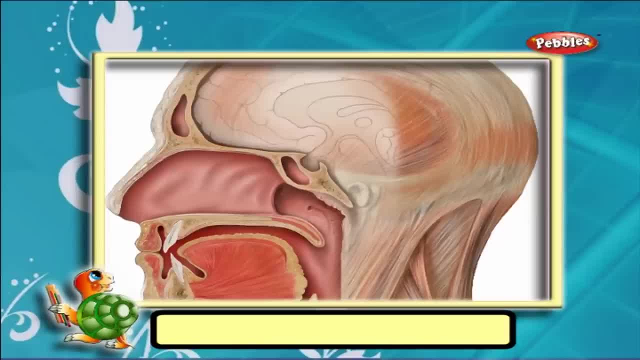 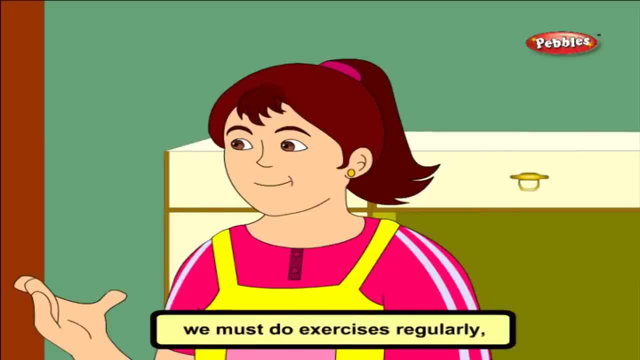 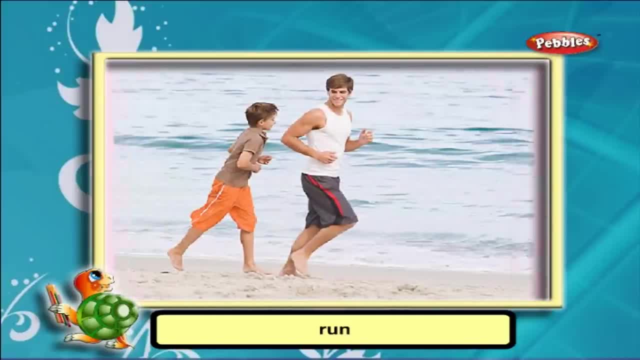 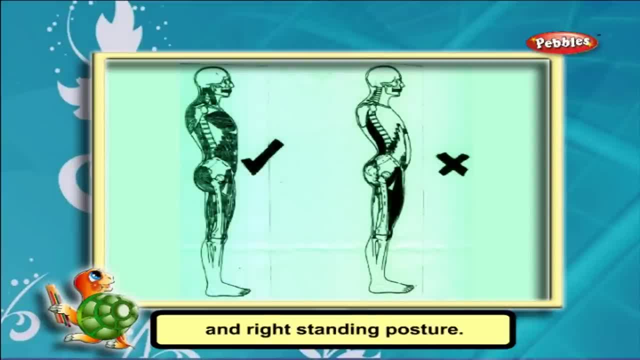 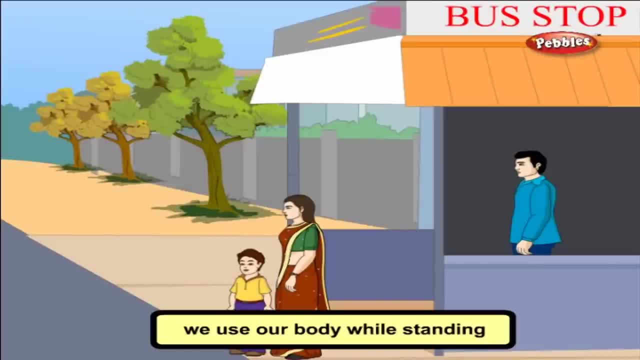 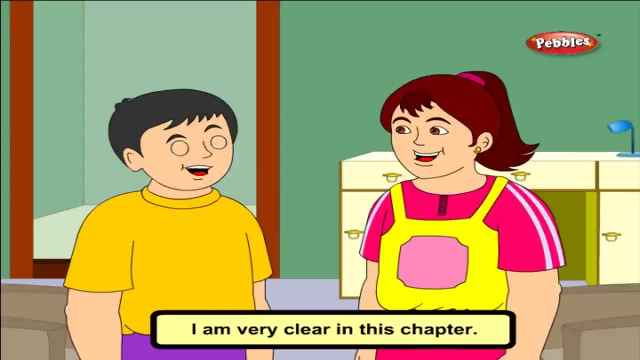 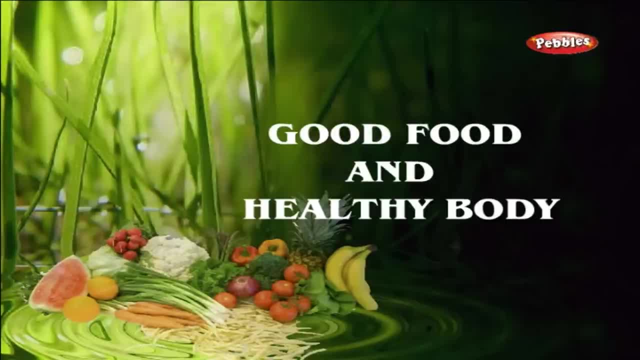 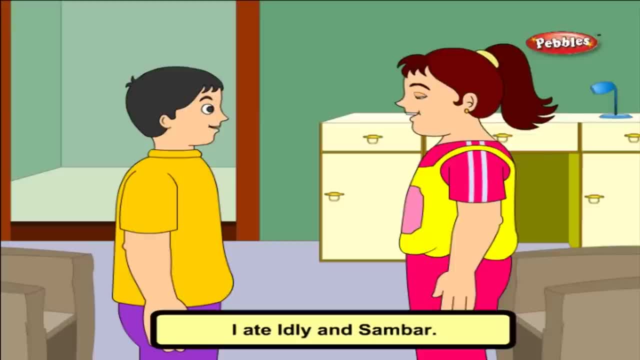 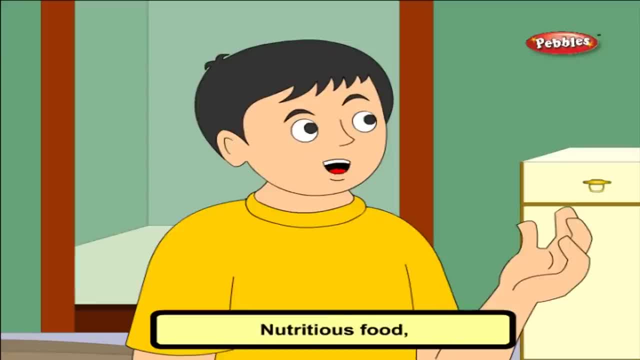 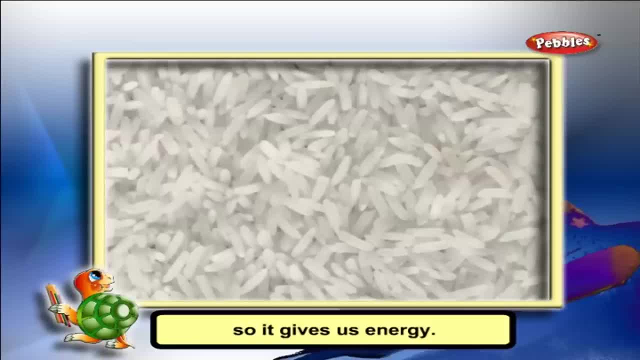 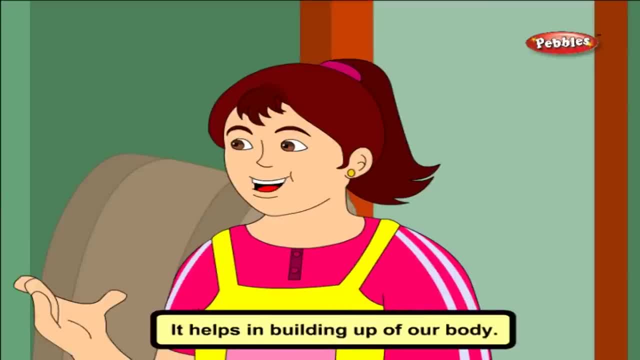 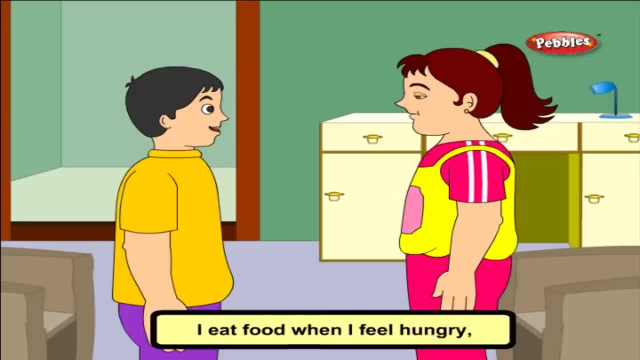 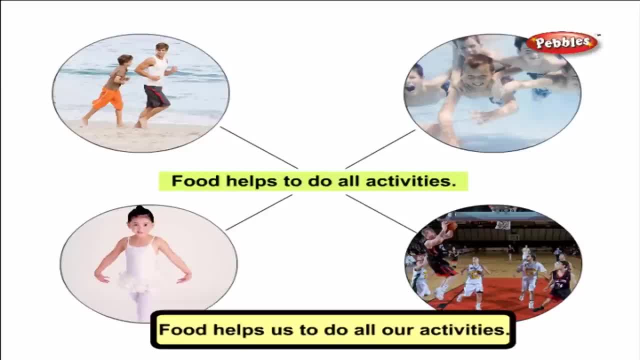 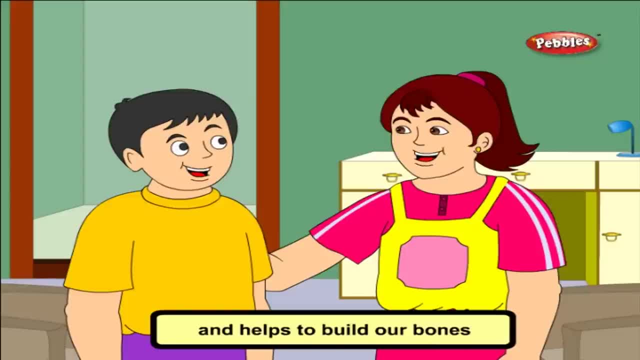 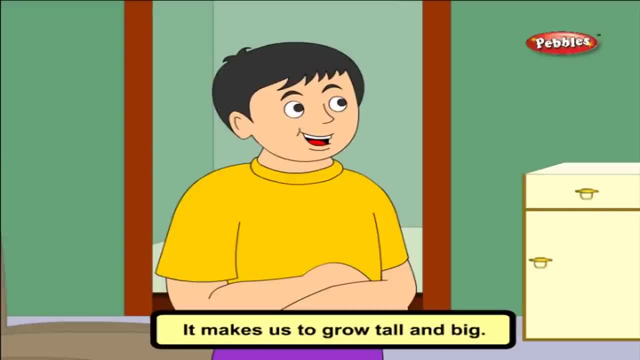 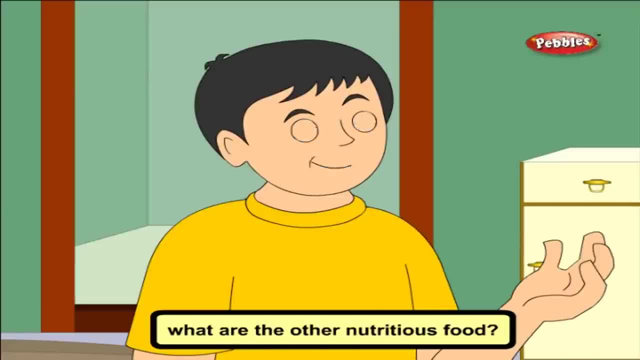 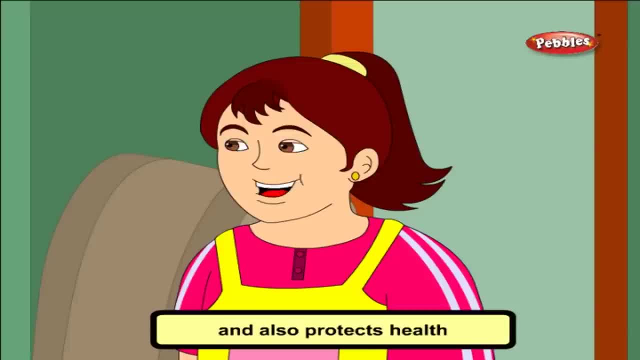 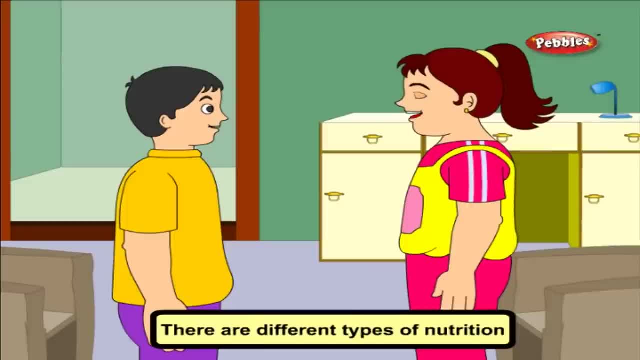 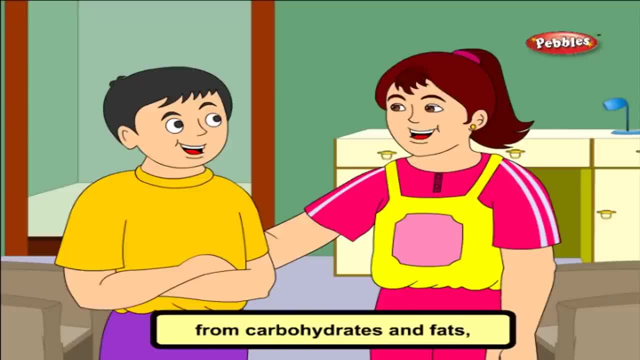 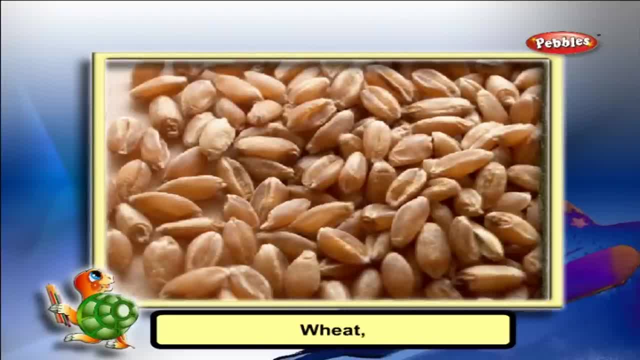 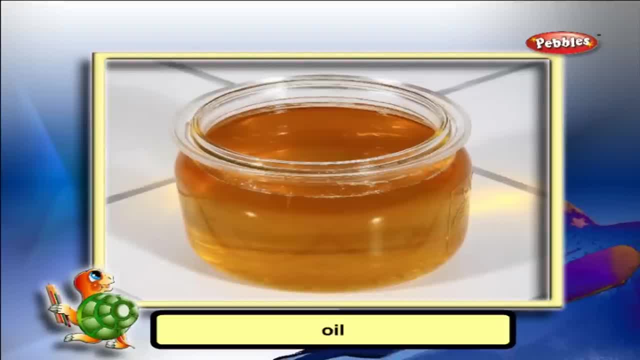 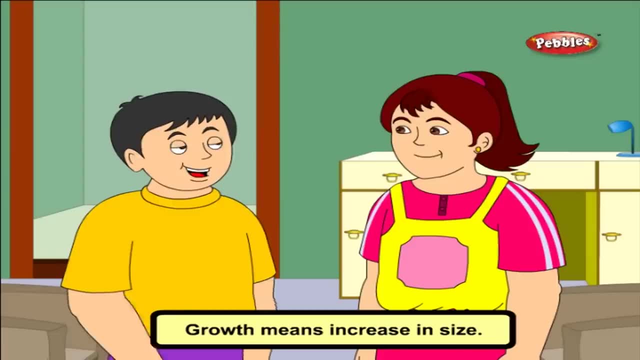 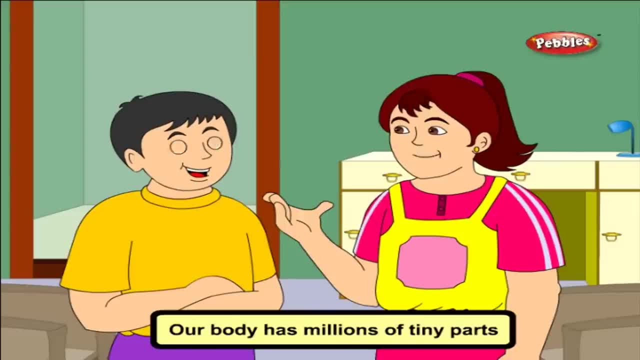 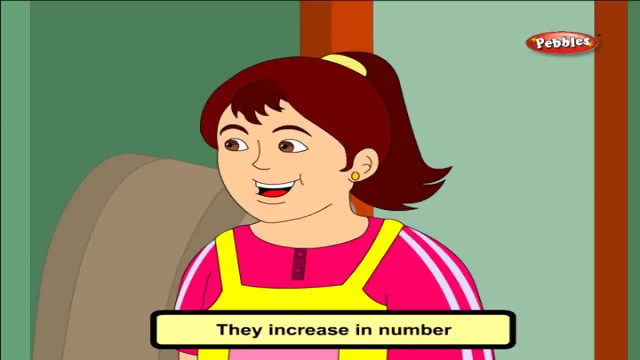 I was a body and I was a man forever. I was a person forever. I was a man forever. I was a human being. I was a human being forever. I was a human being forever. I was a thing I didn't have to. 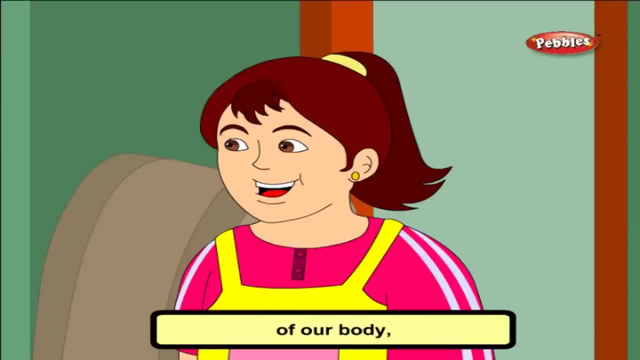 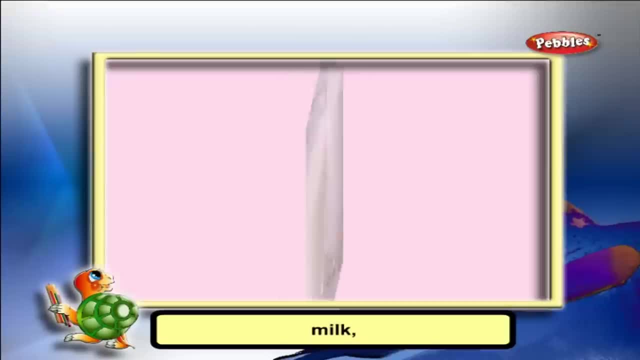 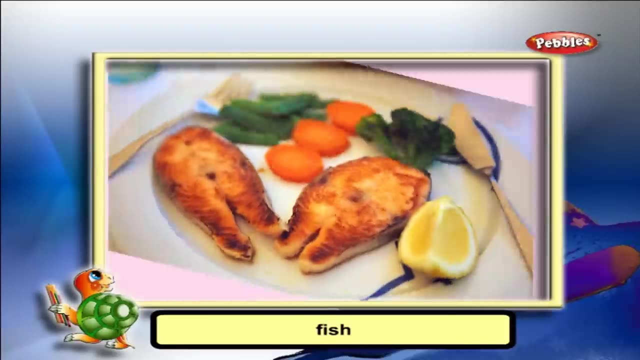 Once I had it, I was deep in guide and testimony. I just got up and I was asleep. I just got up and I was asleep. I was like who's there? Who is this? Every time I would go to bed. I won't sleep tonight, but not tonight. 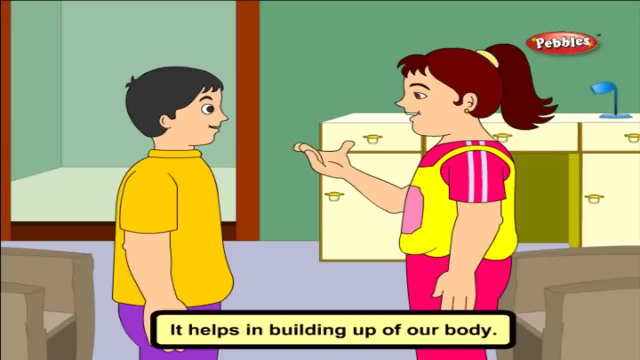 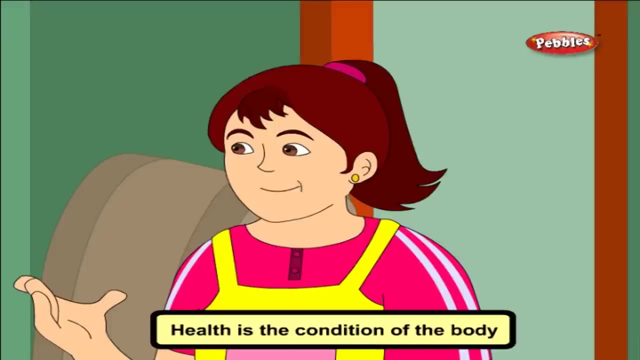 He would get me up Twilight Azalea, a hot body. then it is going to have 40 or 50 results. What does it have to do? It has to do with the issue of the body being without energy or diseases. 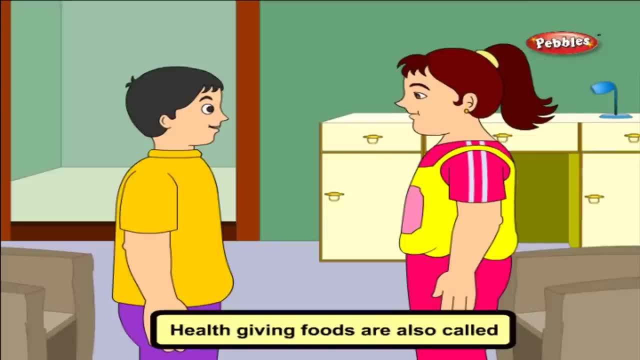 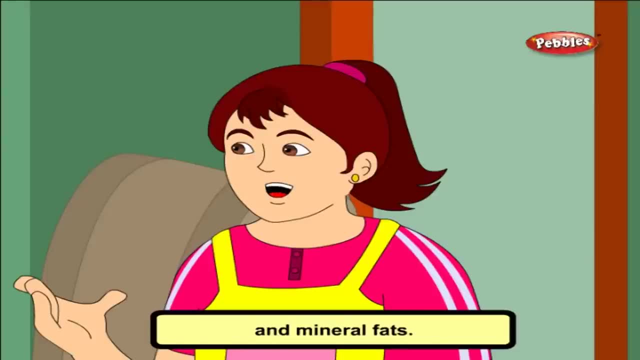 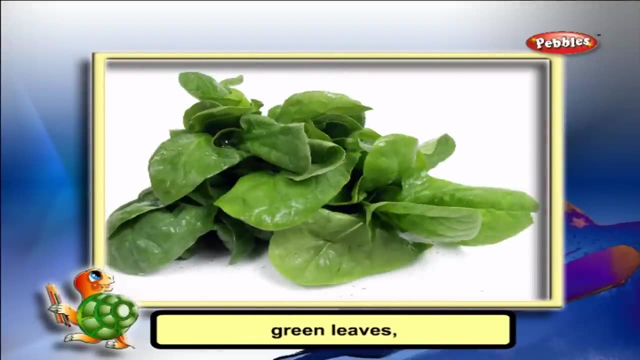 You may have any problem- almost like mine- but that doesn't mean that you shouldn't be running like that. Now you can run in a way that you want to. I love you, my dear. Thank you. I love you, my love. 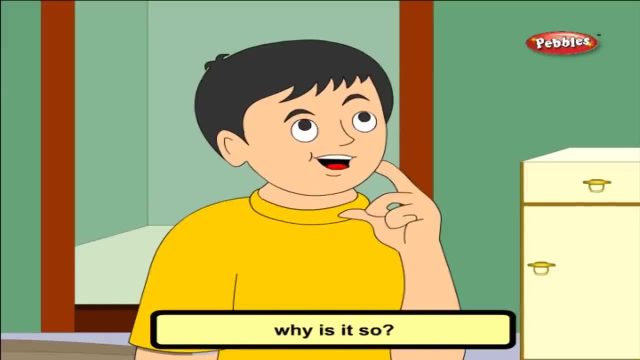 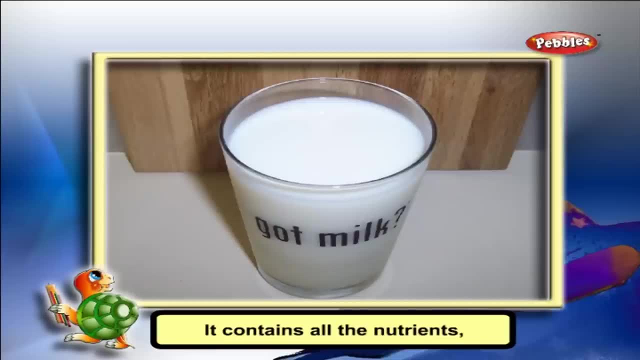 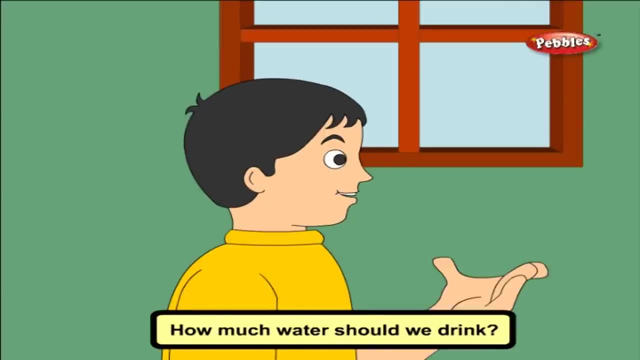 I love you so much. I love you, my dear. I love you so much. I love you, my dear, I love you, my dear. Thank you, Thank you, and we are calling for much greater development. We are trying to make these changes more visible and community. 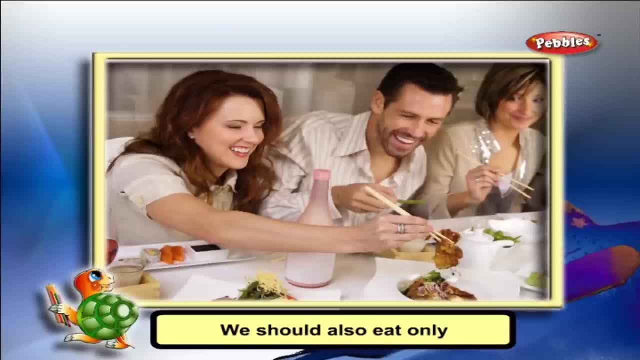 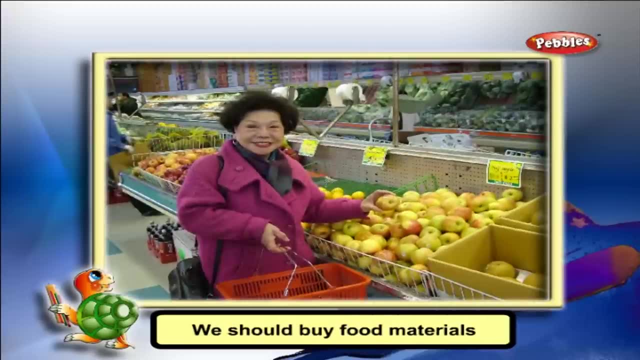 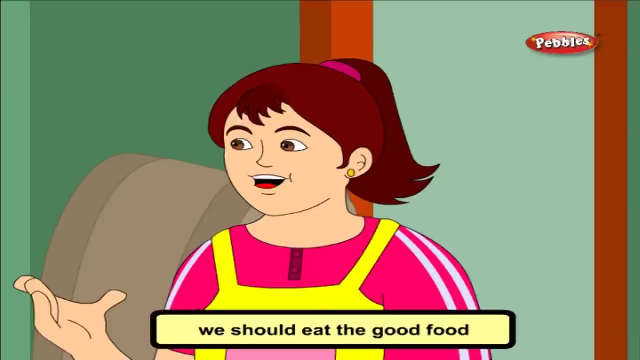 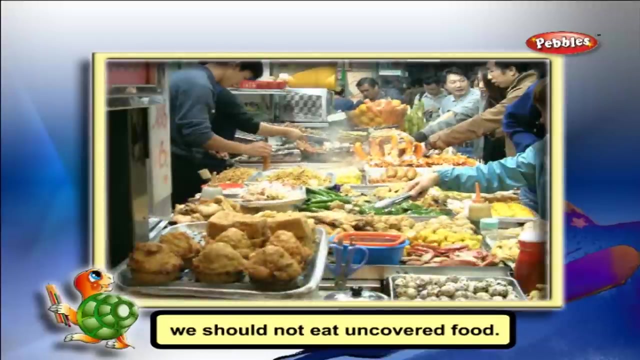 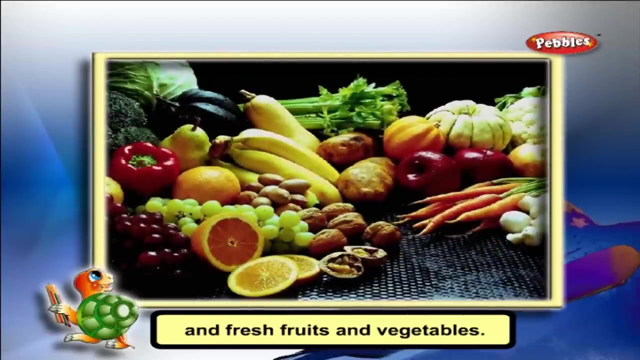 We are also working on the implementation of the new environmental rights act. We are also working on the implementation of the new iblings, Wagnerami, for example, and we are儿s working on these plans. This project requires pass to all the grandchildren and the everyone in the group. 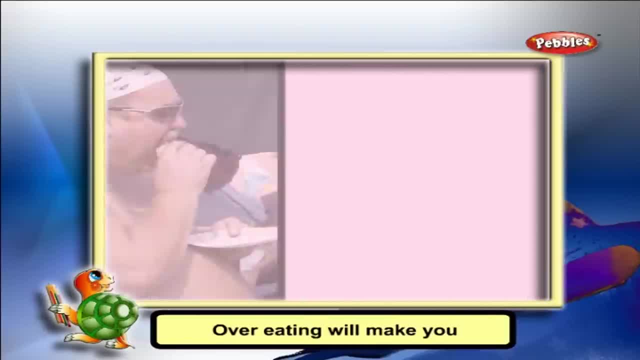 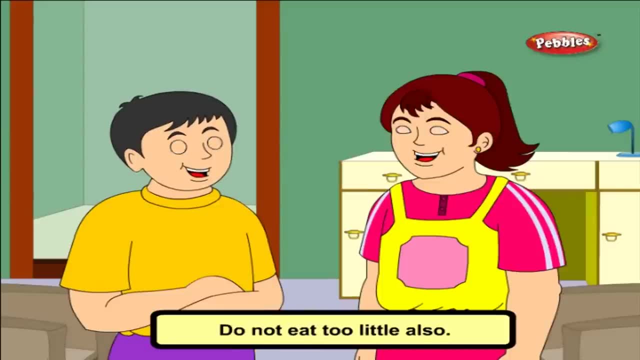 We can do this. Thank you Allrius. safer to you, Mr Graham, The heart is a way of life, of truth, of unity, truth, faith and power In general. when you carry a mouthful of food, you give your heart. 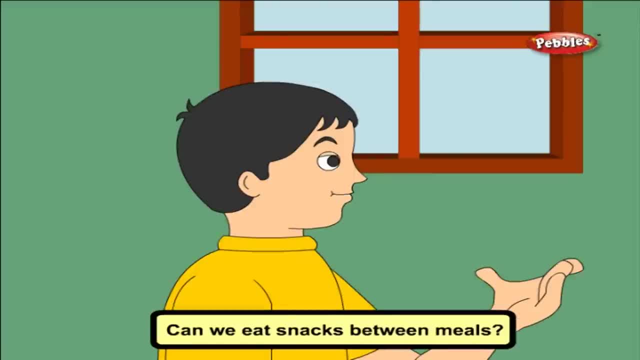 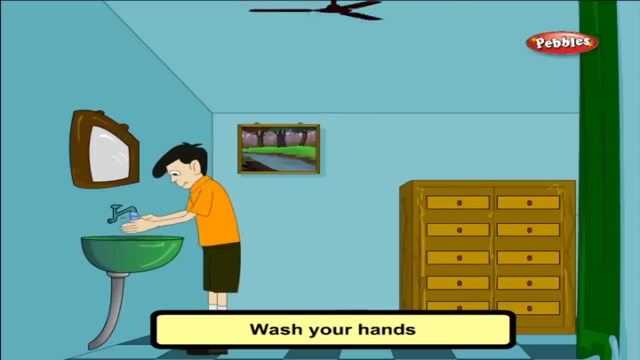 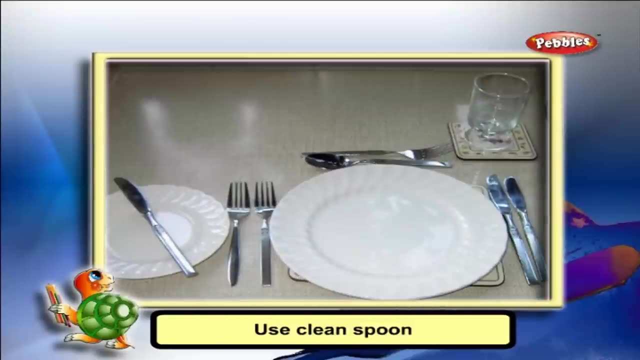 But today there might be a surprise in between places. No, it is not for what they eat. What you have in your mouth is not for what you eat, but for what you have in your mouth. You are standing in the kitchen of a castle. 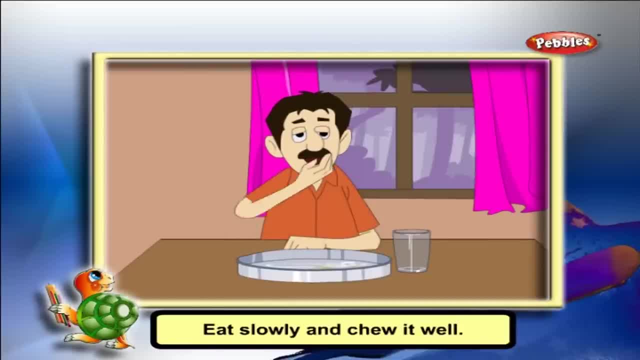 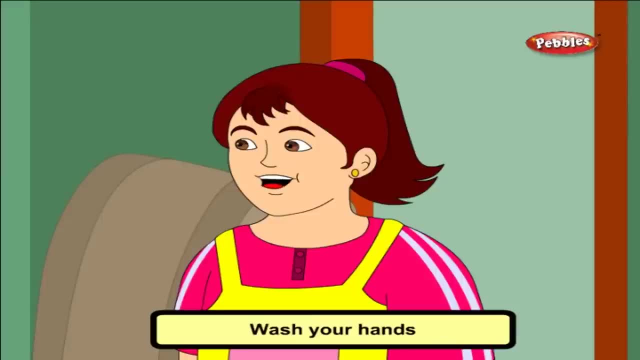 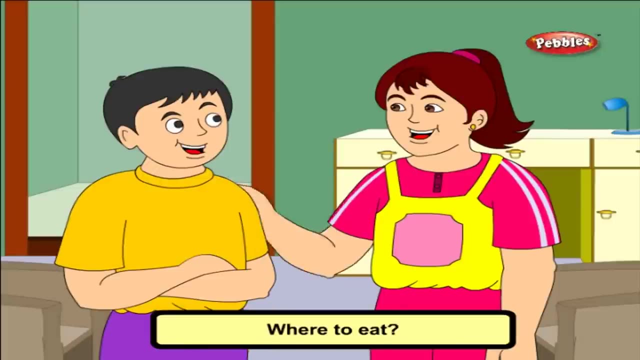 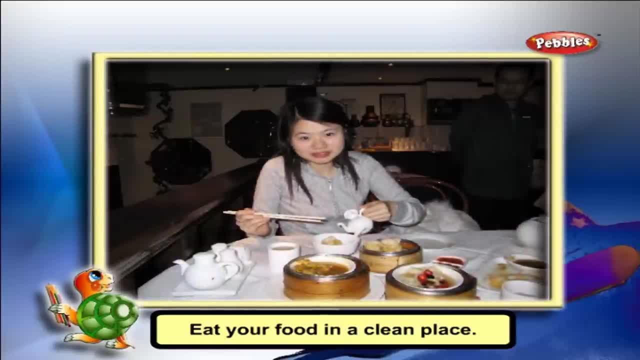 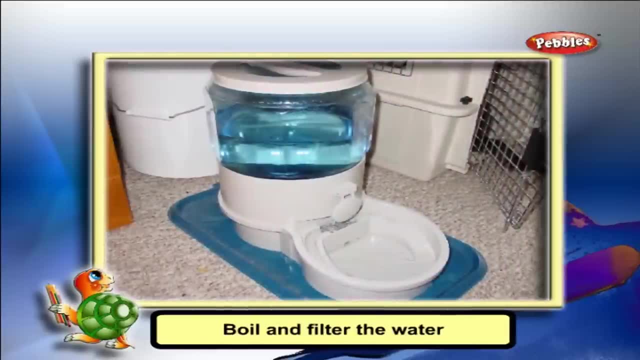 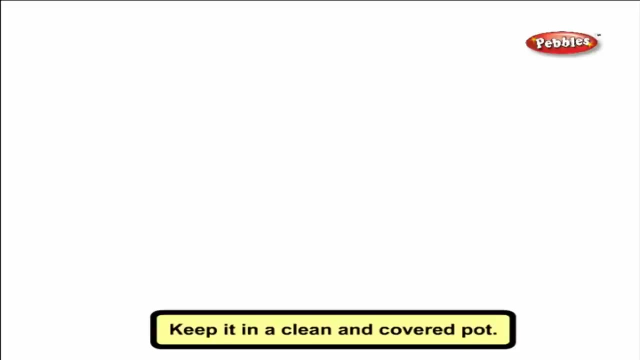 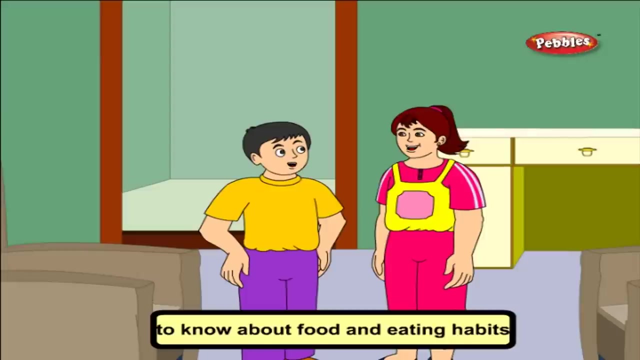 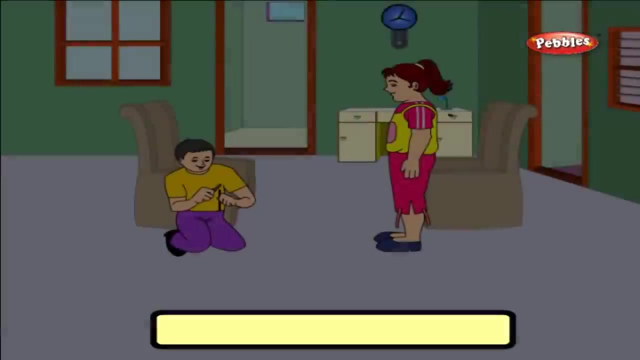 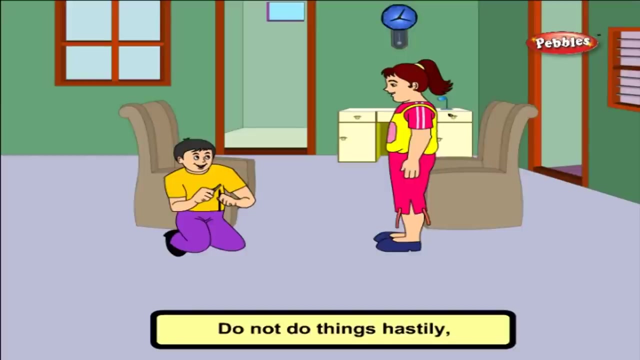 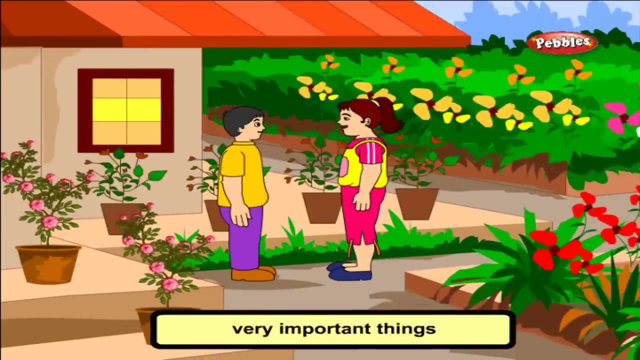 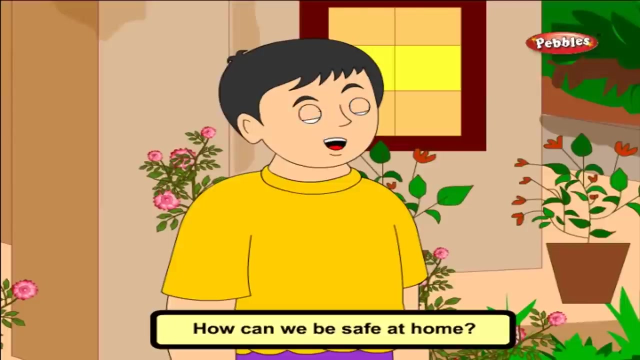 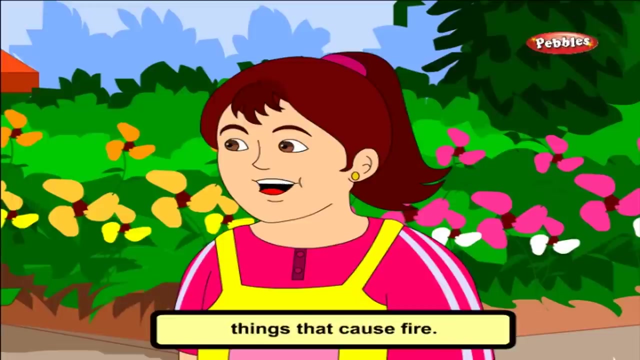 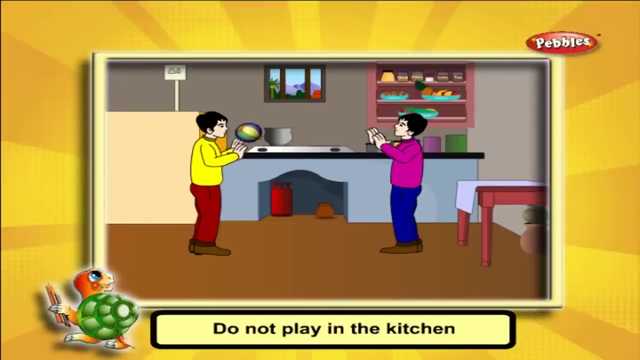 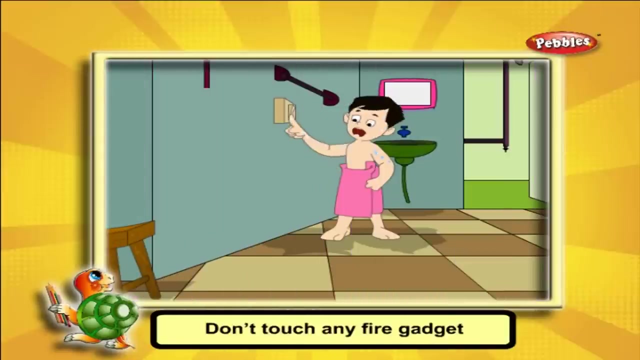 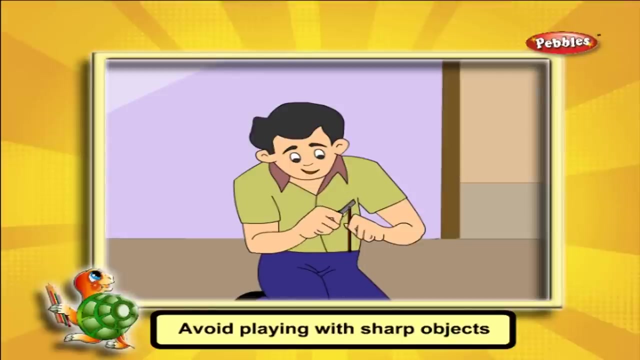 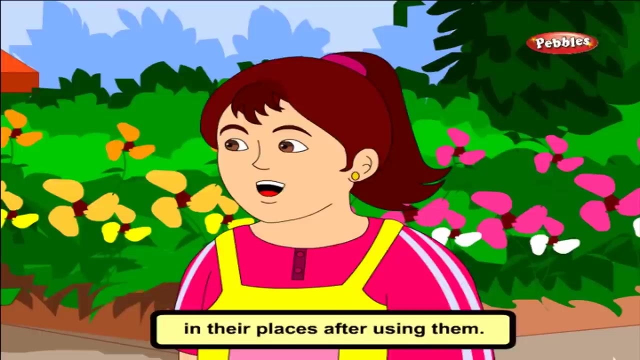 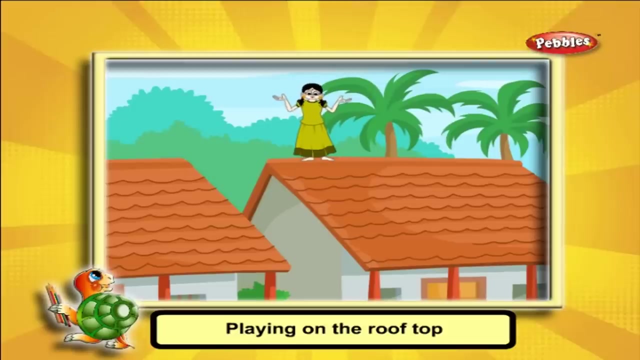 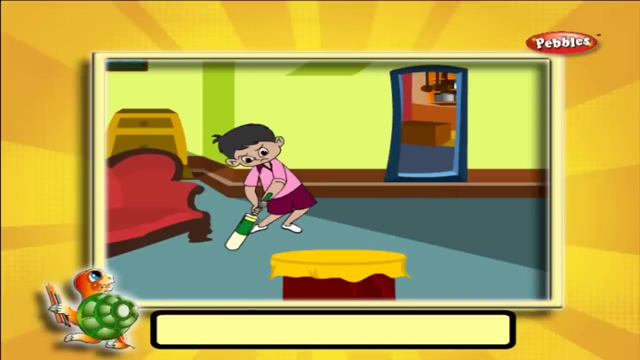 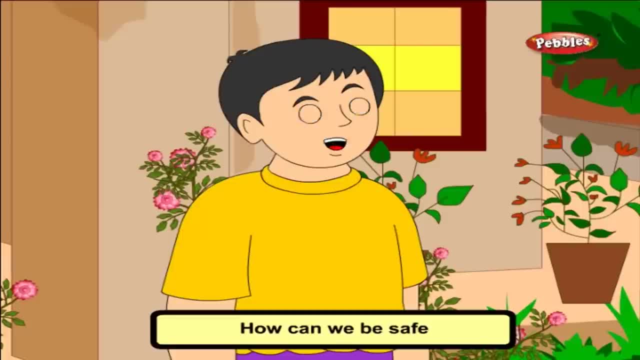 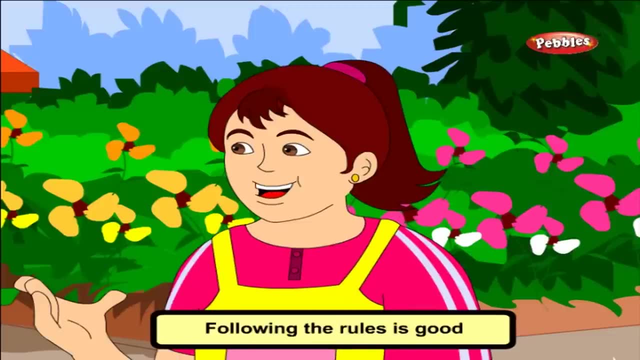 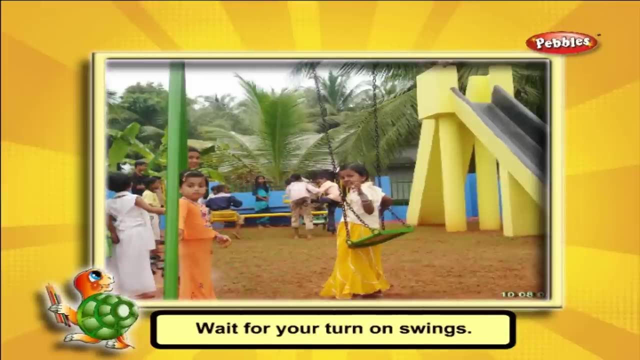 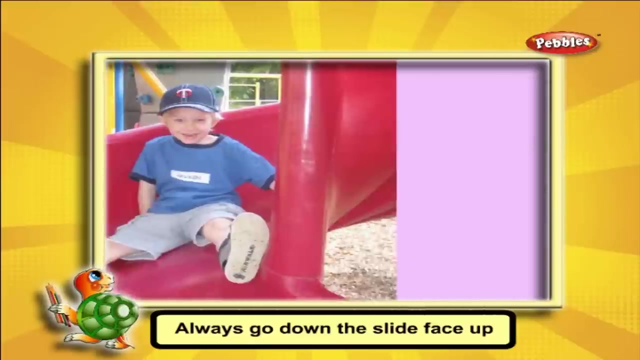 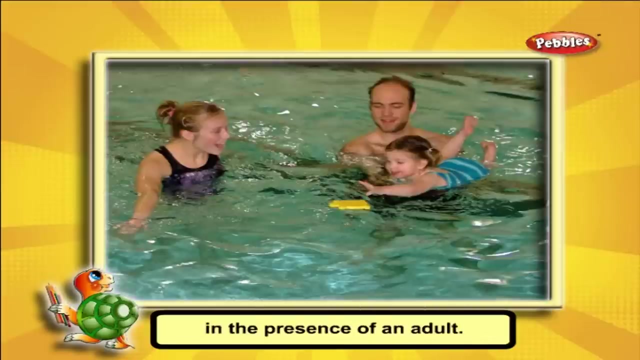 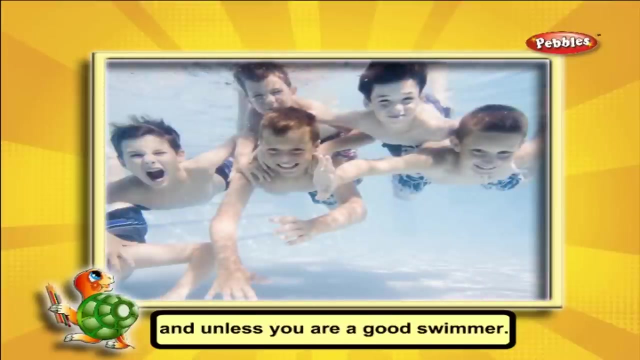 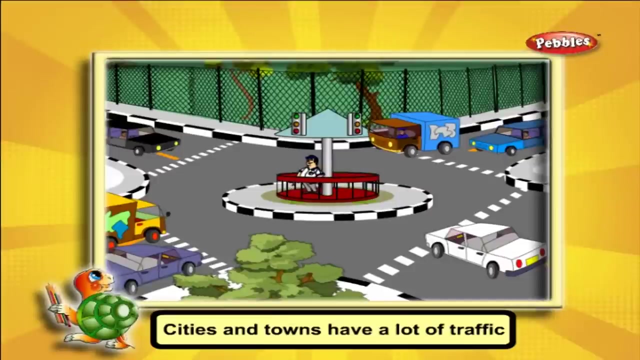 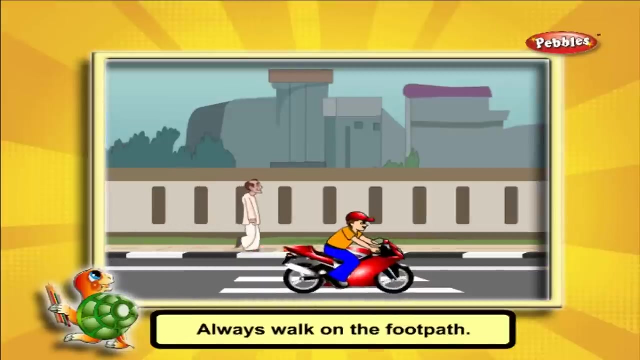 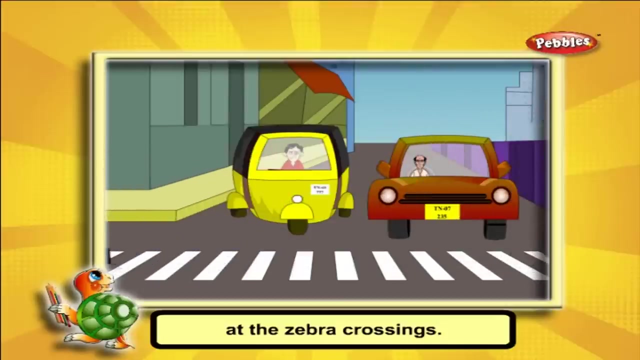 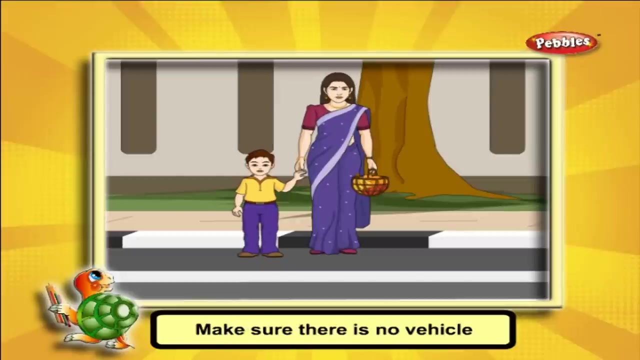 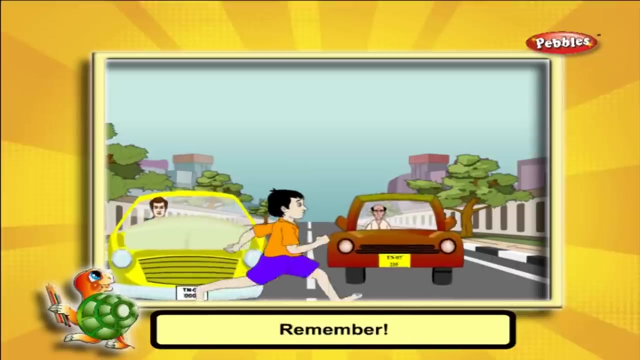 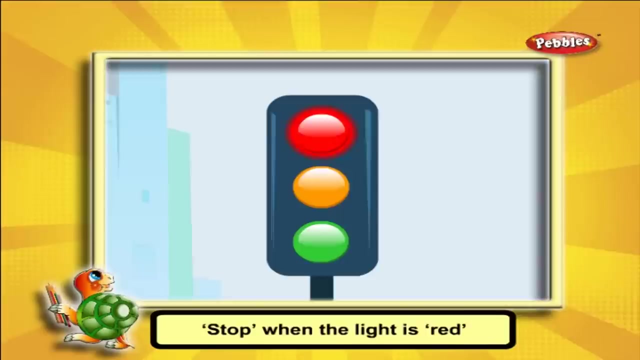 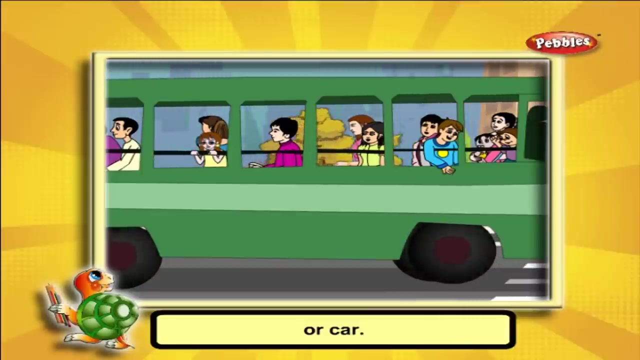 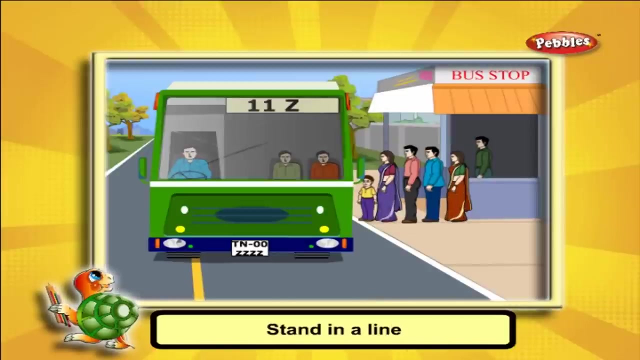 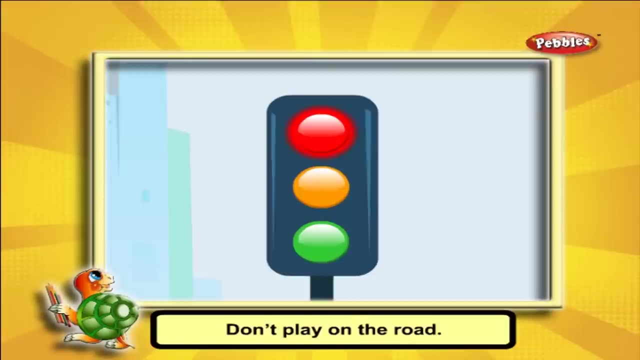 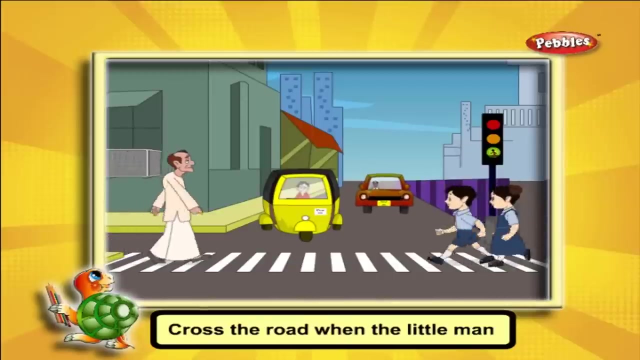 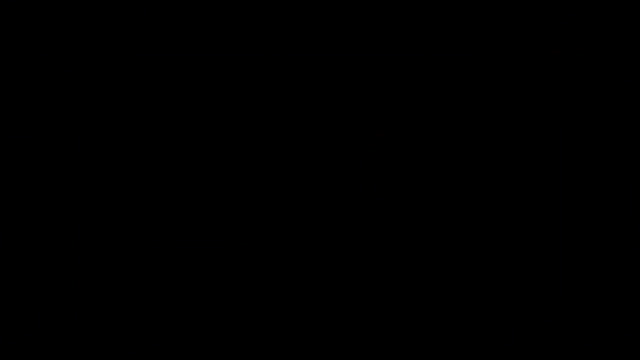 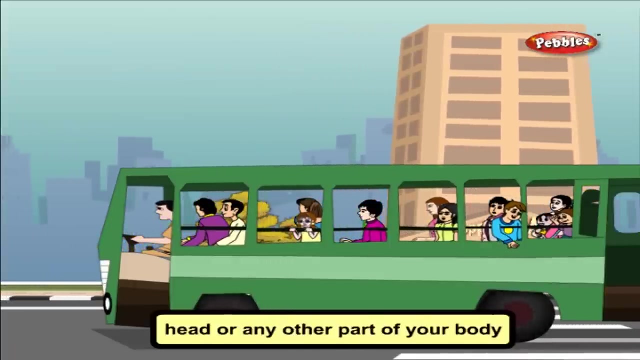 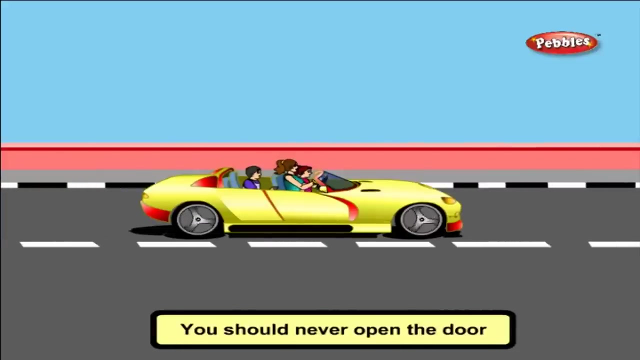 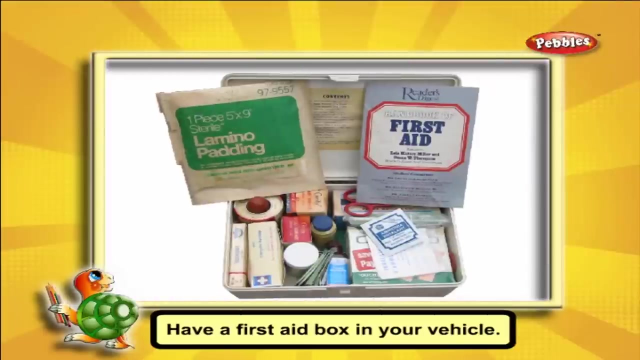 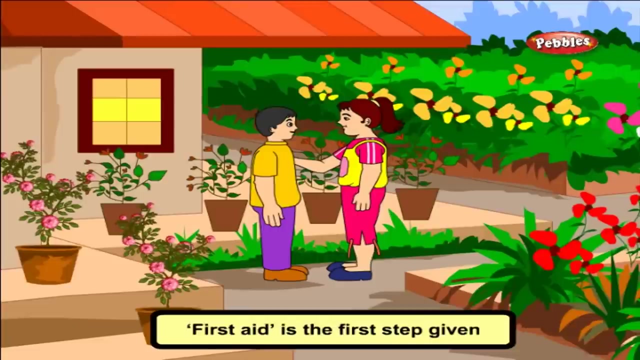 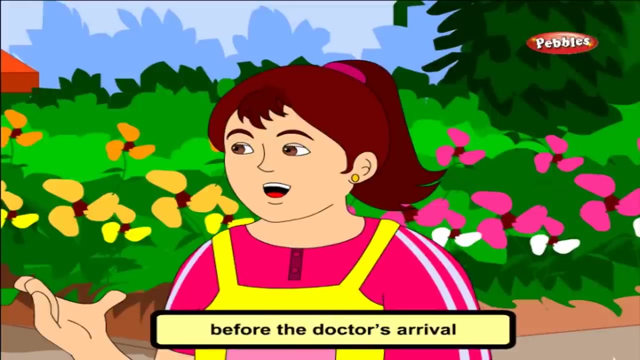 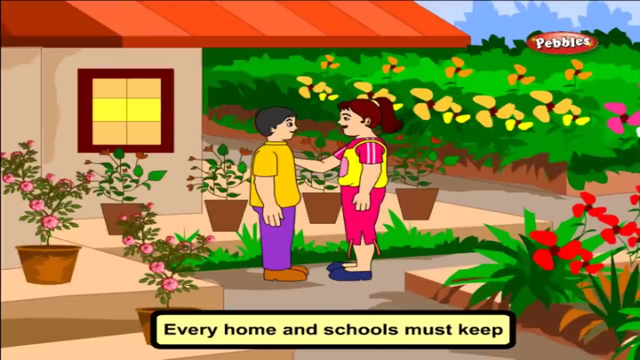 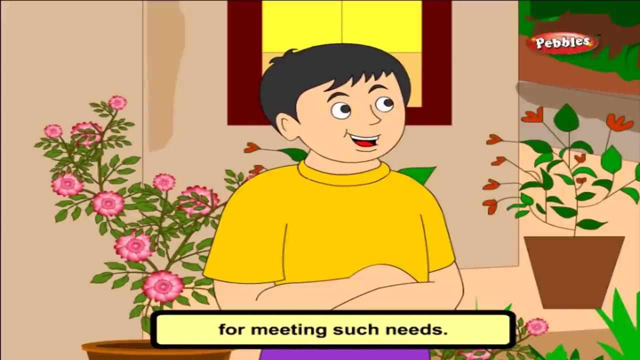 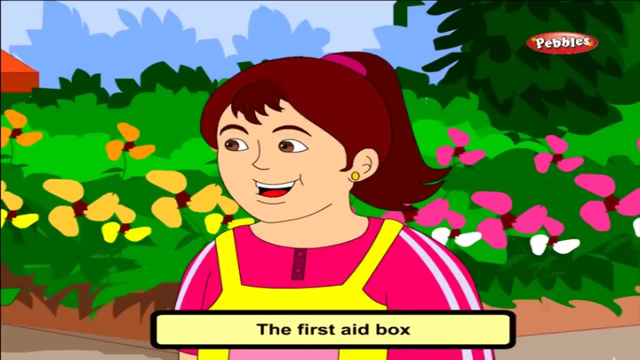 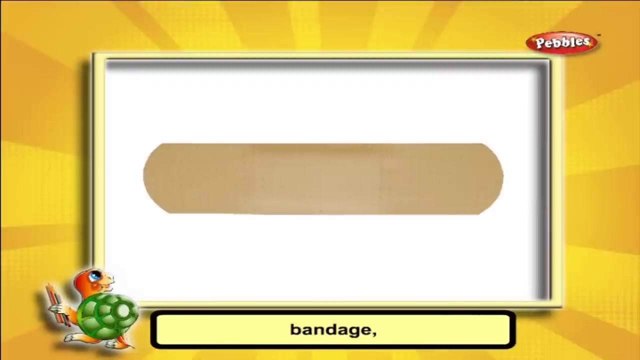 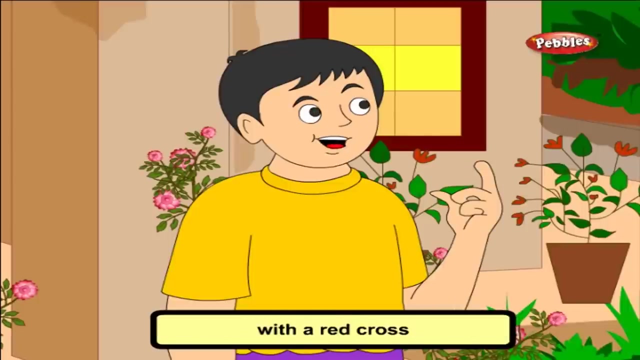 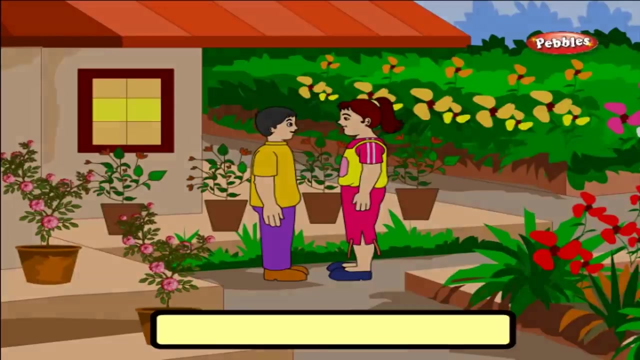 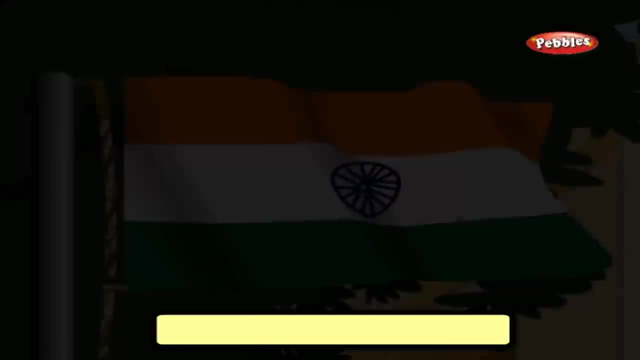 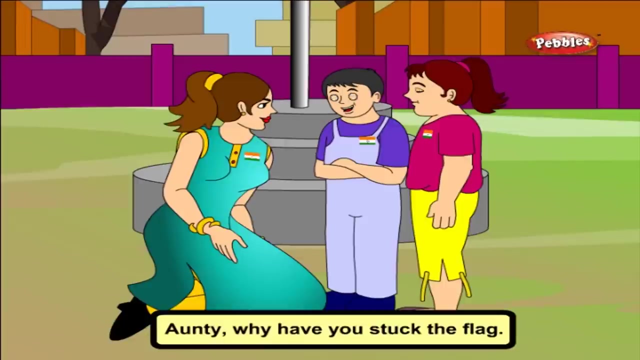 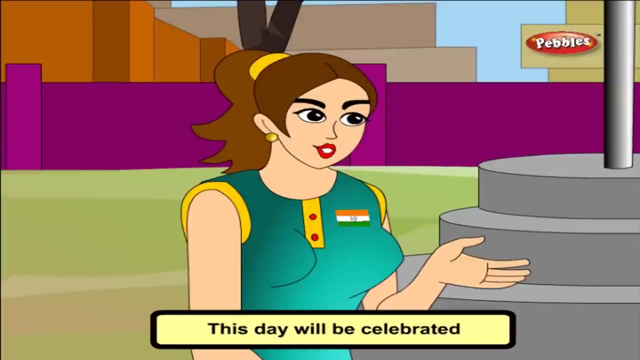 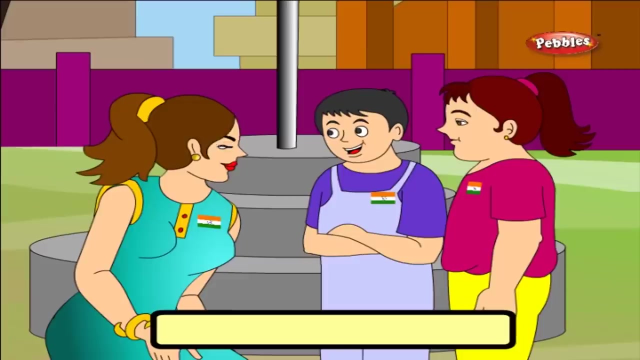 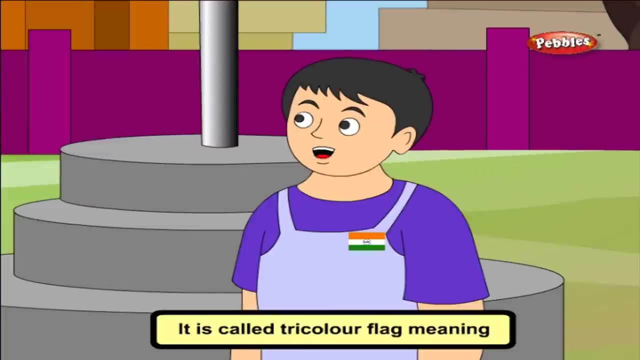 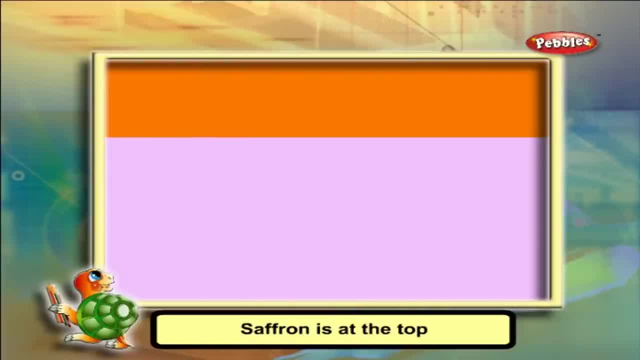 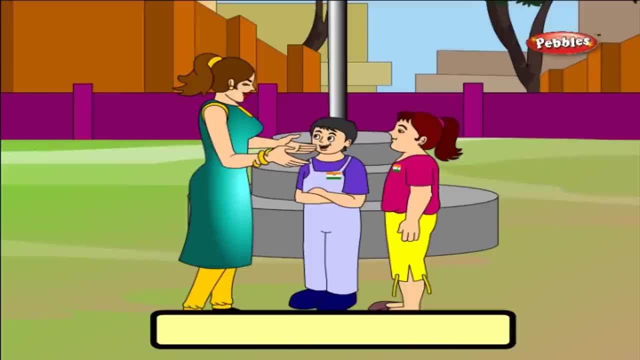 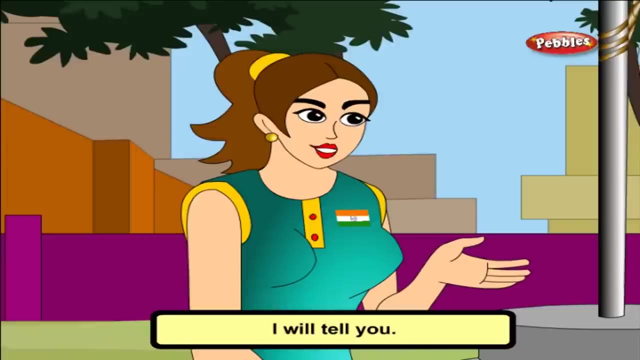 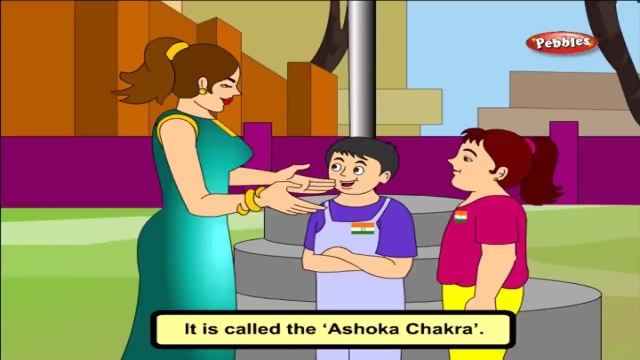 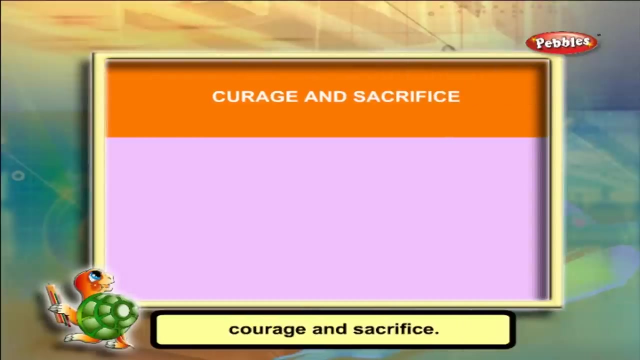 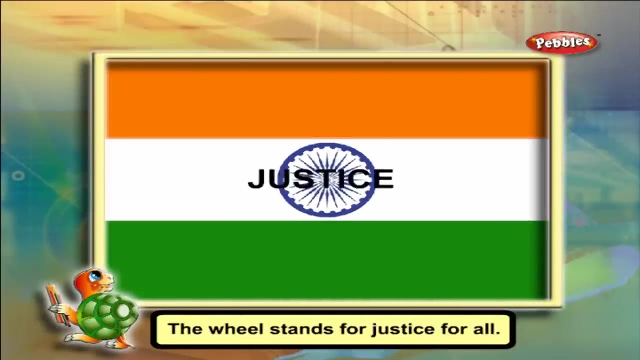 Thank you for watching Good. What is the other name for that blue wheel? I will tell you. Don't worry, It is called the Ashoka Chakra. Rahul. tell me the significance of those colors, Rahul. what is the significance of those colors? 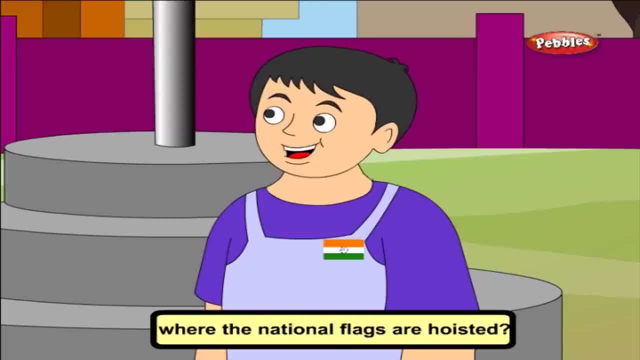 Rahul the cool color seekers' nick Satori, Yes, Satori, Yes Satori, Yes Satori, Satori, Yes, Sori, Sori, Sori, Yes, Sori, Sori. 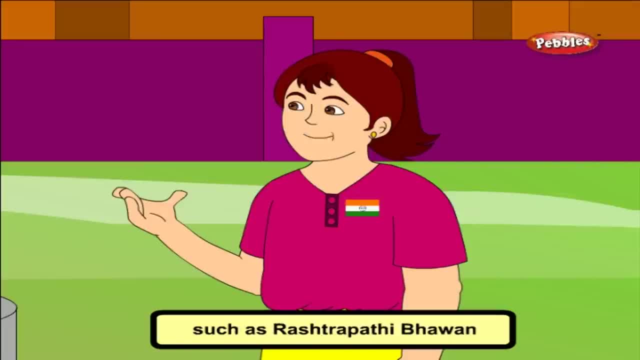 Yes, Sori, Yes, Yes, Sori, Sori, No, Sori, Sorińst, Sori, Sori, Sori, No Sori. États-M Shoes everything. H changshuo, everything. 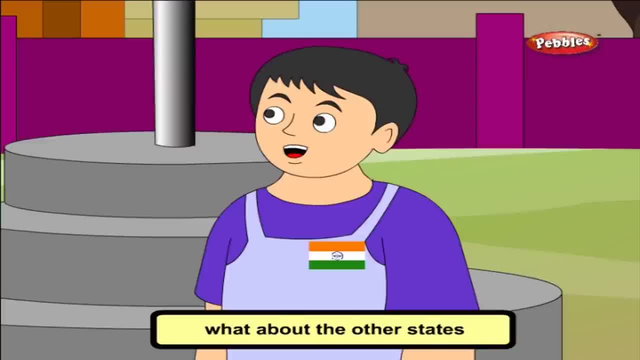 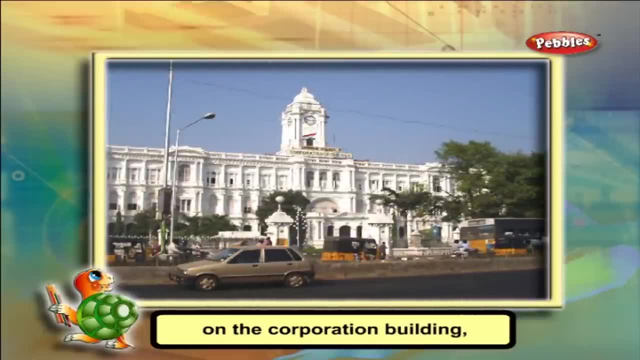 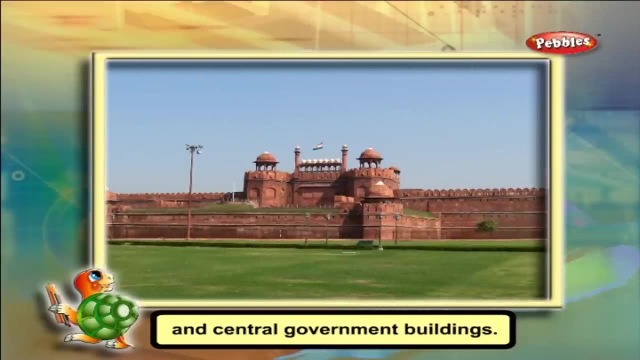 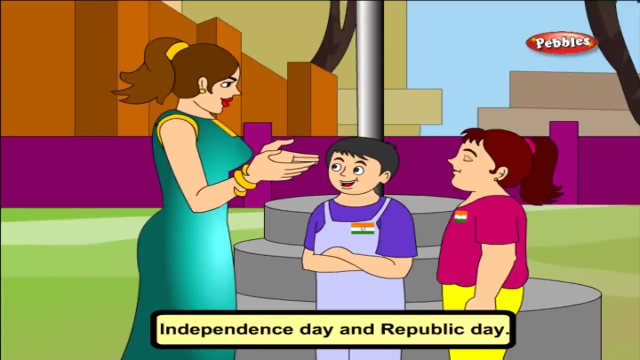 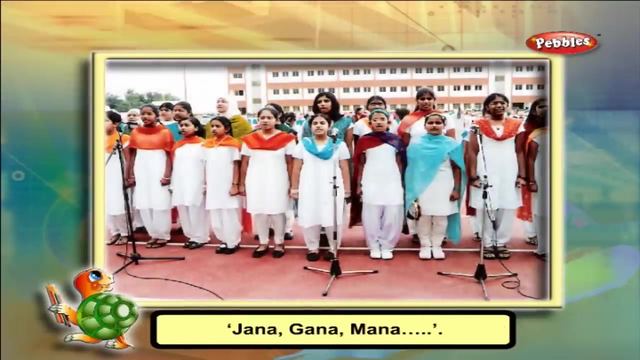 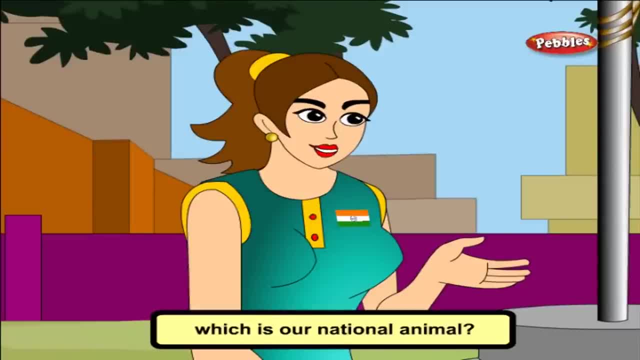 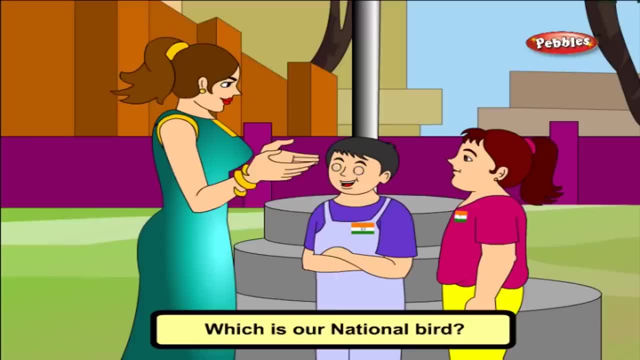 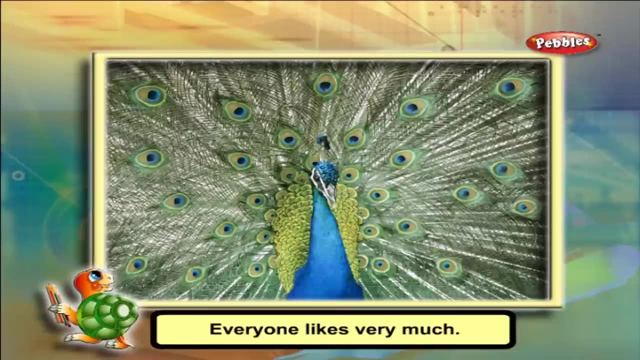 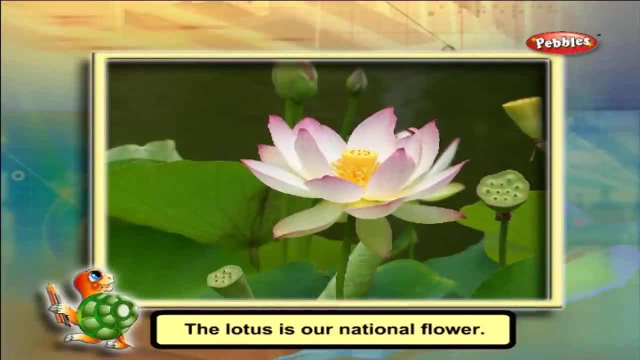 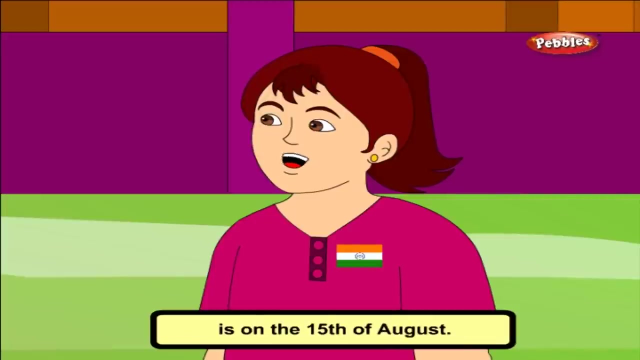 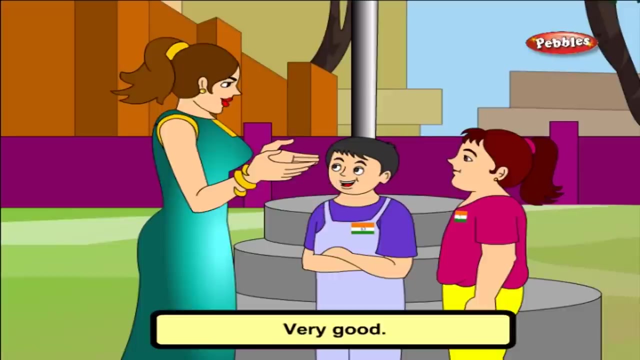 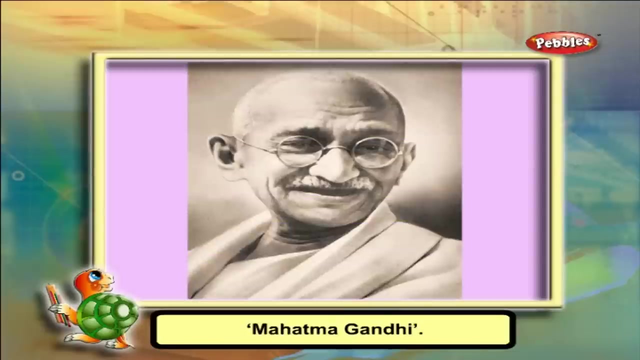 Rahul, do you know which is our national animal, Which is our national bird, Which is our national flower? Priya name any three national holidays? Very good. Who is called the father of our nation, Priya? tell me about our national anthem.